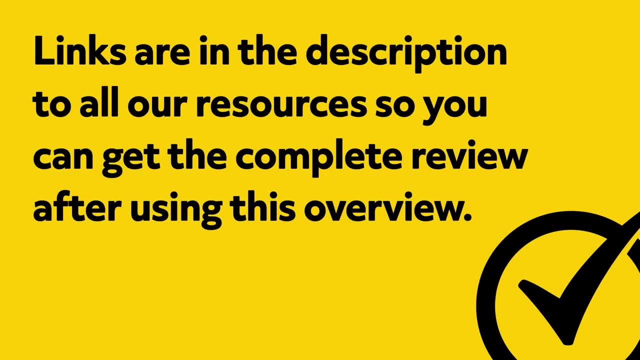 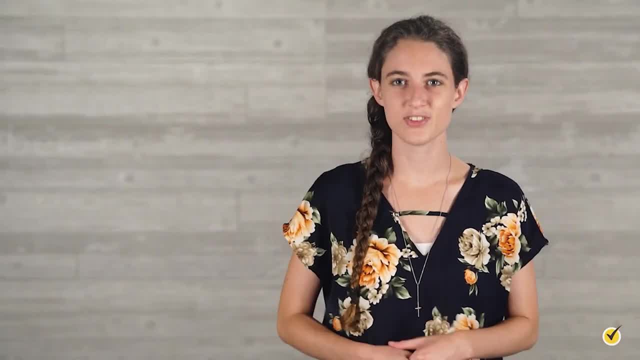 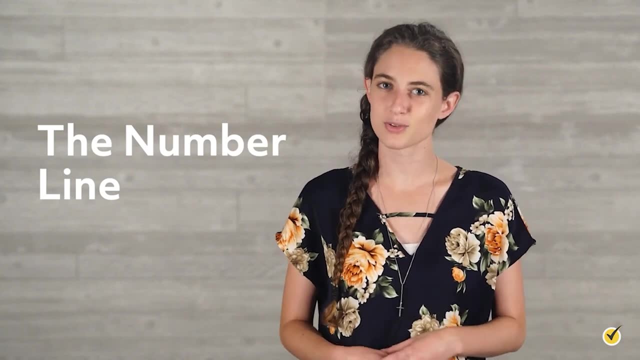 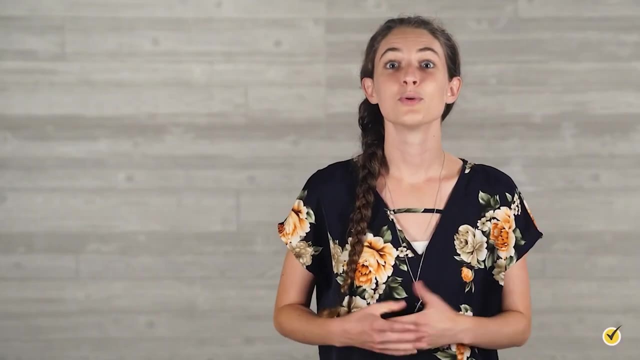 Hello and welcome to this video about the number line. In this video we will explore how to read number lines, draw and plot points on a number line and add and subtract with a number line. Let's get started. We will use a number line to represent numbers in counting order. The number to the left. 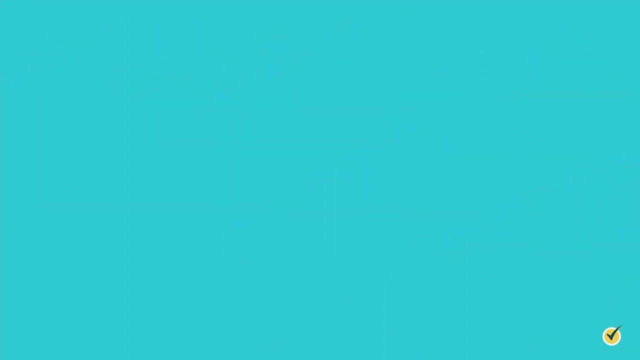 is always smaller than the number to its right. To draw a number line, we first start by drawing a straight line and then we put arrows at the ends. The arrows represent the fact that the number line goes on forever in both directions. When dividing the number line with tick marks, 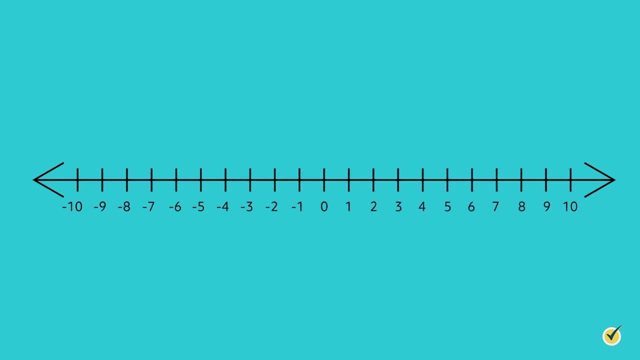 it is important to place the tick marks equally spaced apart. This shows that the distance from any two numbers is the same. For example, the distance from 1 to 2 is the same as the distance from 2 to 3.. The most important number on a number line is 0, because every other 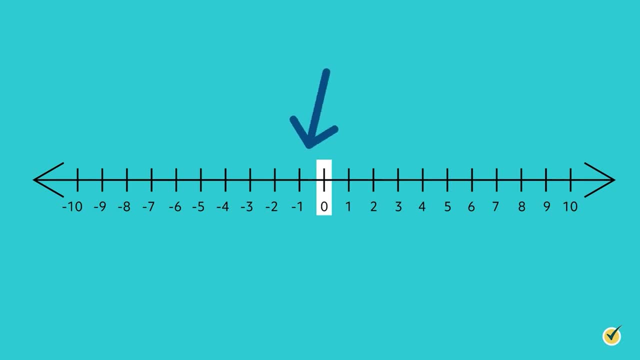 number is spaced off of how far away it is from 0. Numbers to the left of 0 are negative and numbers to the right of 0 are positive. Number lines continue infinitely in either direction. so the number line you see is always only part of the whole number line, Because 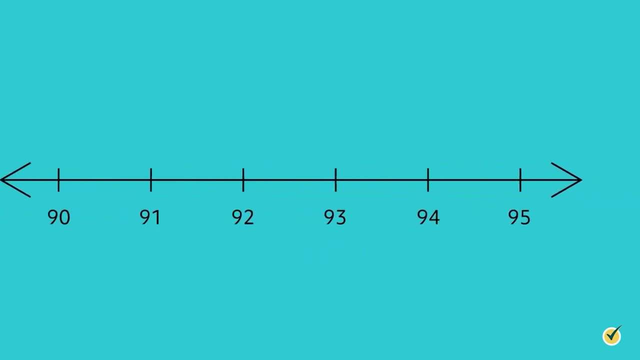 of this. even though 0 is the most important number, it might not show up on your number line. For example, your number line might look like this: if you are trying to plot the grade you got on your test, Number lines can be used to represent a specific number In. 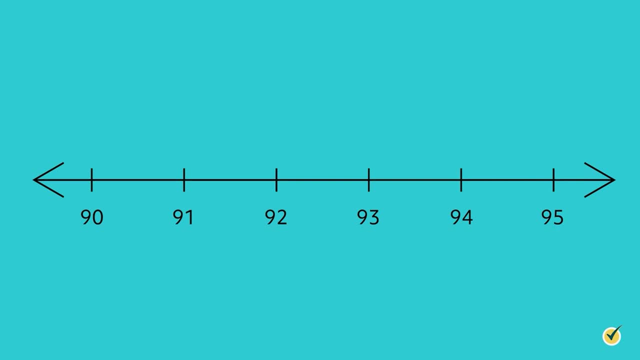 the example we just mentioned, we will use a number line to represent a specific number. We can use the number line to represent a test grade of 94 by putting a dot above the number. like this, Plotting a negative number would happen the same way. Simply put a dot. 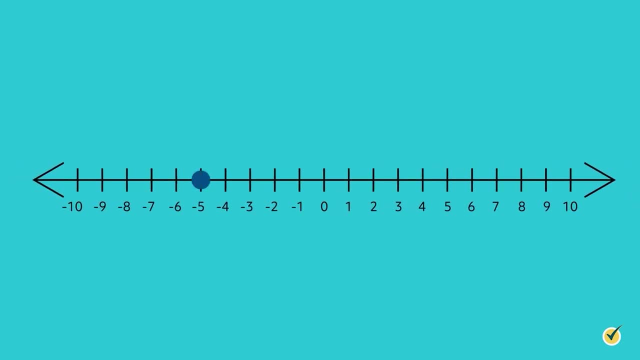 over the number you are wanting to represent. The number line here shows the number negative, 5.. We can also use a number line to help us add and subtract numbers. Movement to the right is for addition and movement to the left is for subtraction. To use the number: 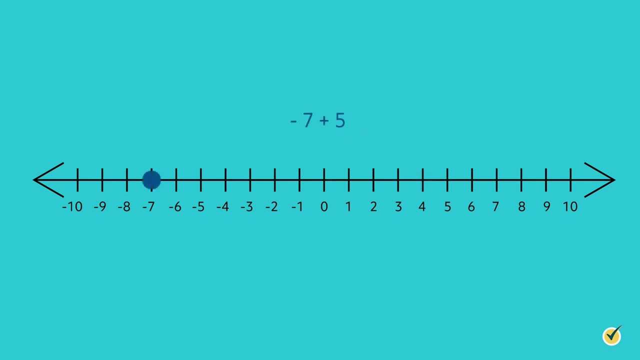 line for adding and subtracting. we start by plotting a point at our first number, Then we move right or left, depending on the operation. Let's practice by adding negative 7 plus 5.. We will start at negative 7, and since the 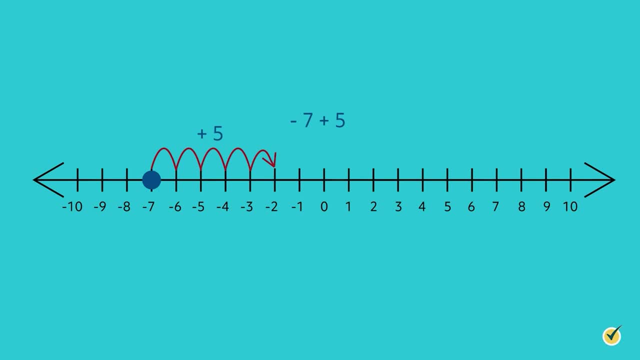 operation is addition, we will move to the right 5 spaces. As you can see, we land on negative 2.. Therefore negative 7 plus 5 equals negative 2.. Now let's try subtracting 9 minus 4.. We will start at the number 9 on the number line and since the operation is subtraction, 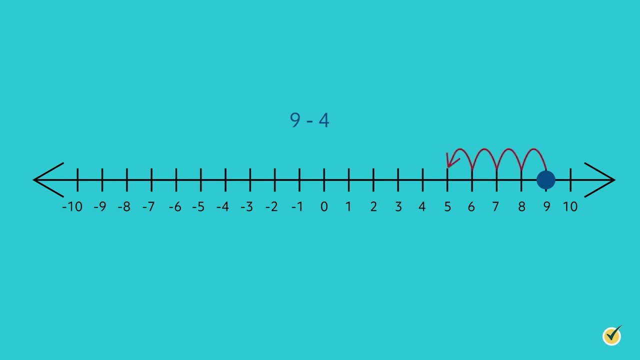 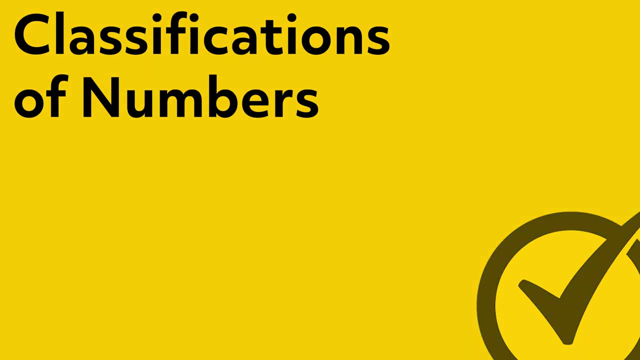 this time we are going to move to the left. We move left 4 spaces, which lands us on 5.. Therefore, 9 minus 4 equals 5.. Why do we classify numbers? Why do we give them names like integers, irrational numbers? 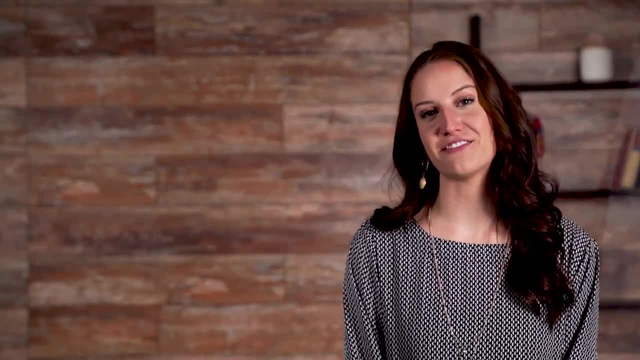 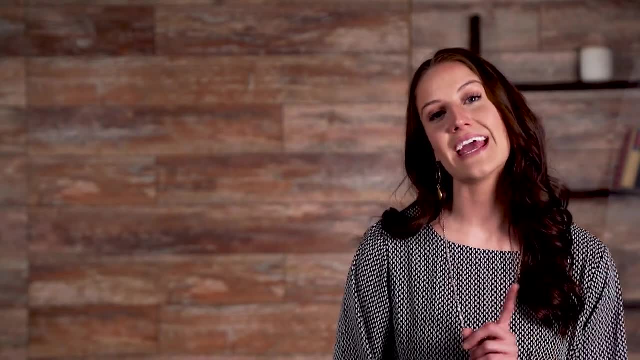 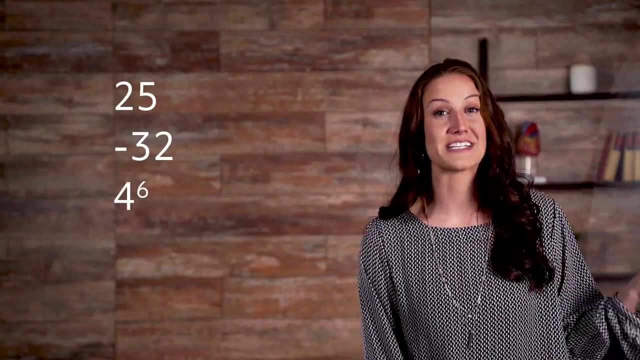 or negative numbers. For the same reason we classify anything, We want to make sure that everyone has an understanding of what specific numbers are called and what they mean. After all, there is a difference between 25 and negative, 32, and 4 to the 3rd. 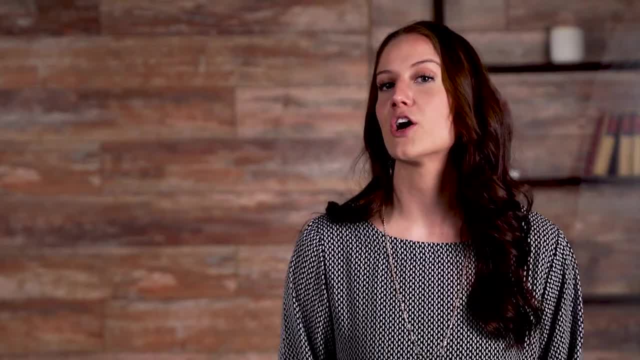 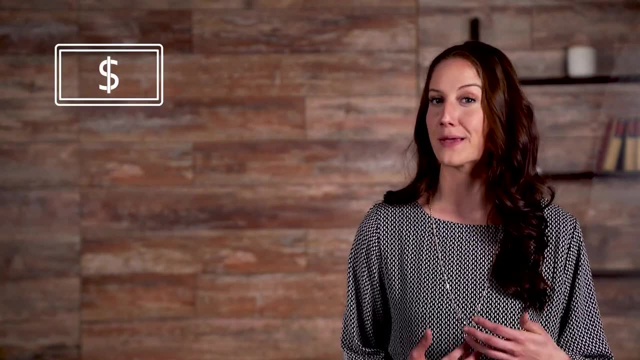 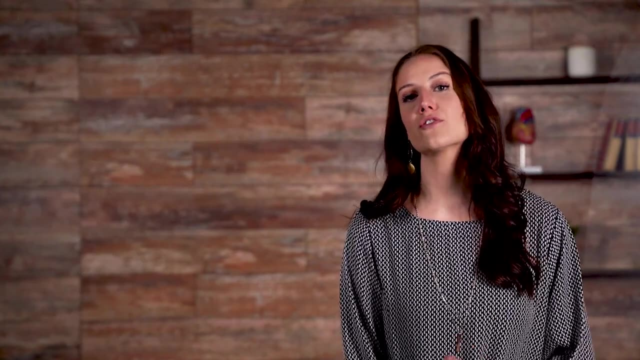 In this Mometrix video, we will provide an overview of numbers and their classifications. Numbers are our way of keeping order. We count the amount of money we have, We measure distance. We use percentages to indicate a sale. Numbers are an integral part of our everyday existence, Whether they are whole numbers, 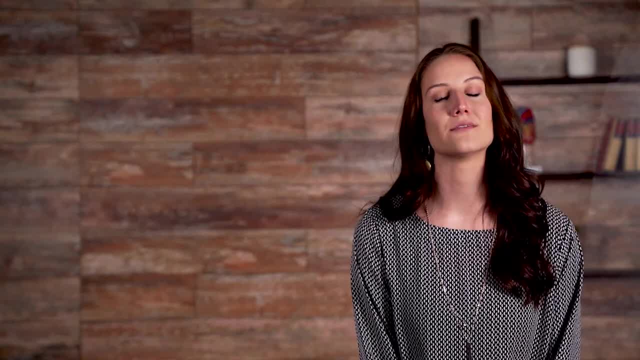 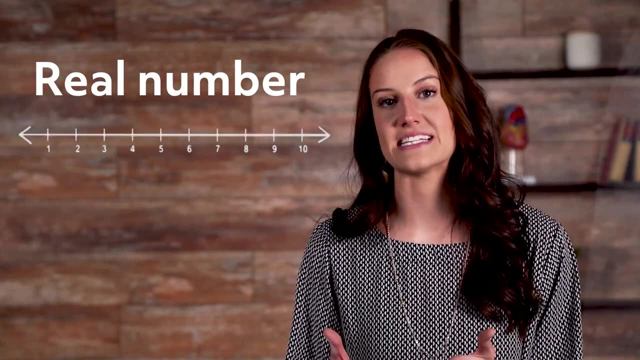 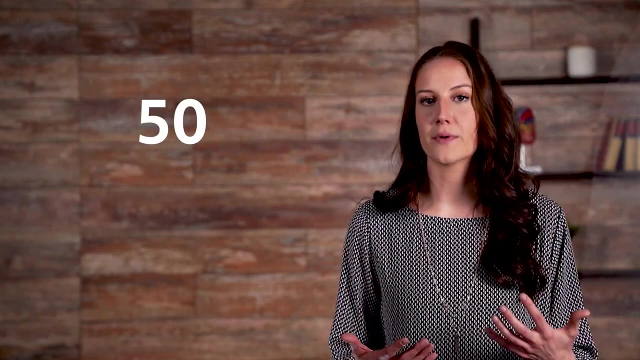 rational numbers or the first type of numbers. we are going to look at Real Numbers. A real number is any value of a contingent, A continuous quantity that can represent distance on a number line. Essentially, it's any number you can think of. 50 is a real number. 1 billion is a very large real number. 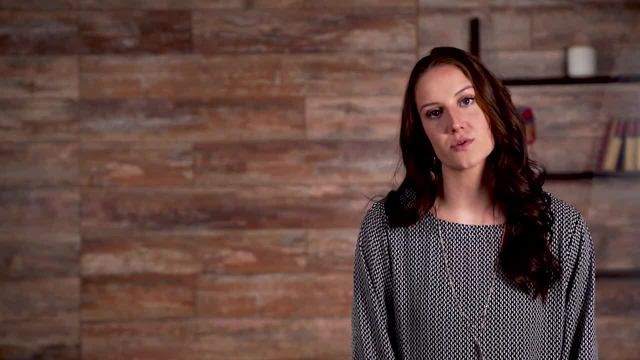 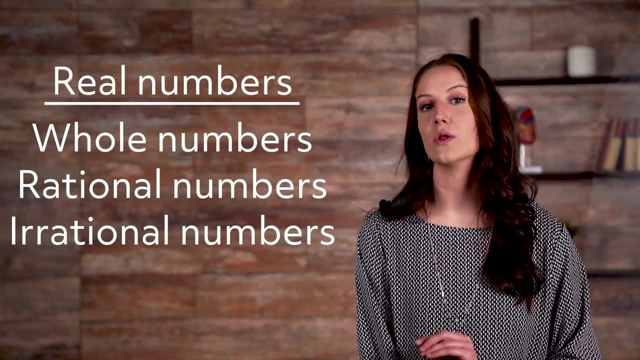 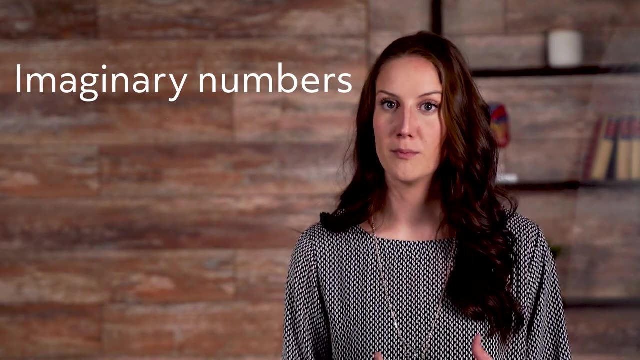 Real numbers encompass three classifications of numbers, which we will talk about in a little bit. Whole numbers, rational numbers and irrational numbers are all real numbers, Imaginary Numbers. Imaginary numbers are not real numbers. They are complex numbers that are written as a real number multiplied by an imaginary unit. i, For instance, the square root of 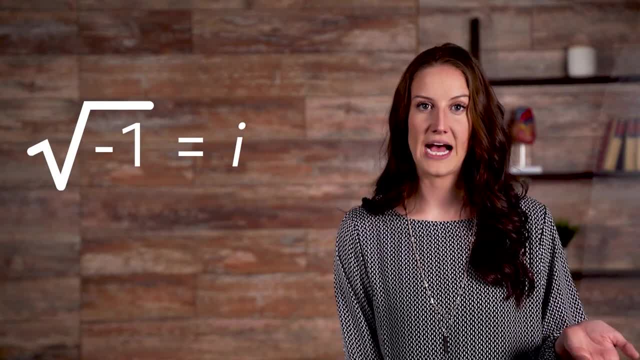 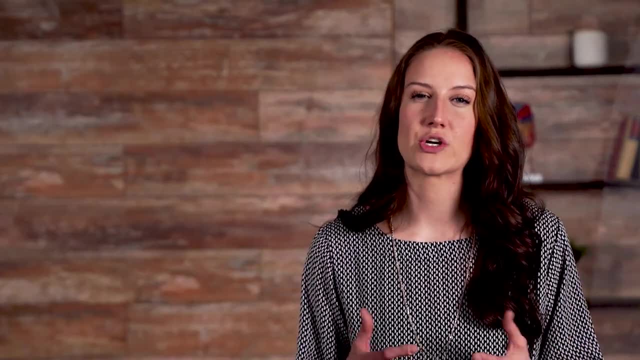 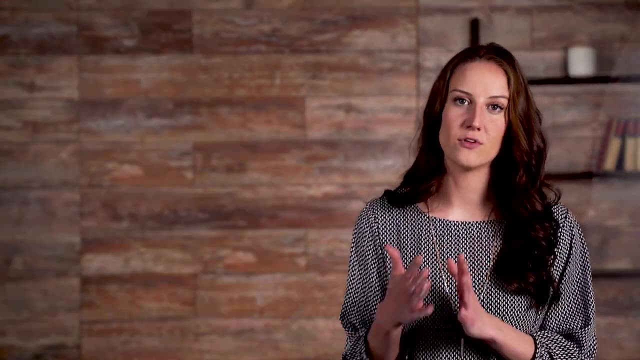 negative 1 calculates as the imaginary number i and the square root of negative 25 is 5i. Even though imaginary numbers aren't real numbers, they do have value. Electricians use imaginary numbers when working with currents and voltage. Imaginary numbers are also used. 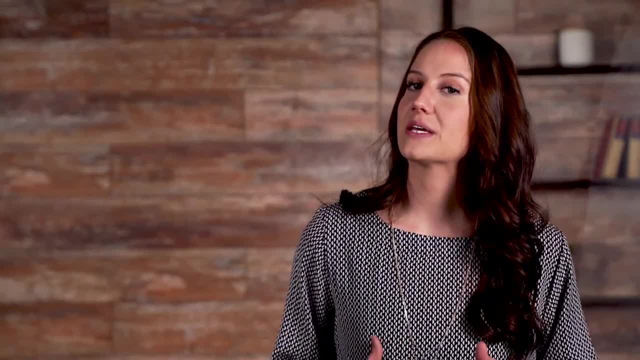 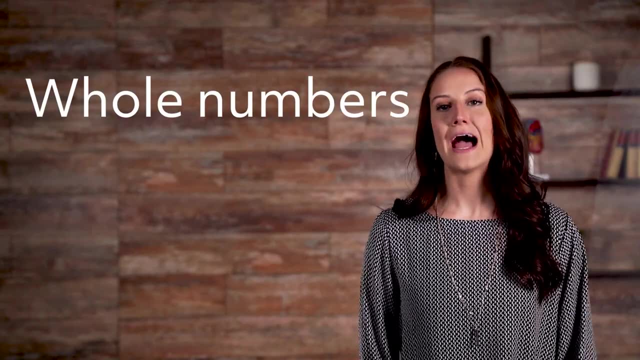 in complex calculus computations. So just because these numbers are called imaginary doesn't mean they aren't useful. Whole Numbers, Whole numbers, are numbers that we count with. 1, 2,, 3,, 4, and 5 are all whole numbers. 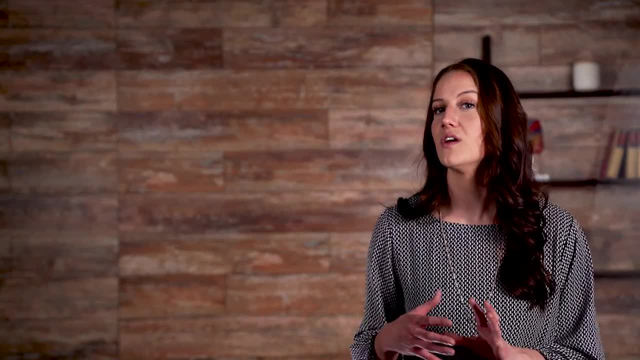 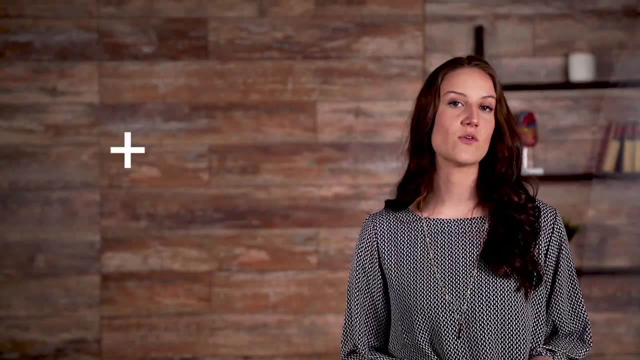 So are negative 17 and 0.. Whole numbers do not have fractions or decimals. All Whole Numbers, All whole numbers, are called integers. Integers can be positive or negative. whole numbers, All integers and whole numbers are part of a bigger group called rational numbers. 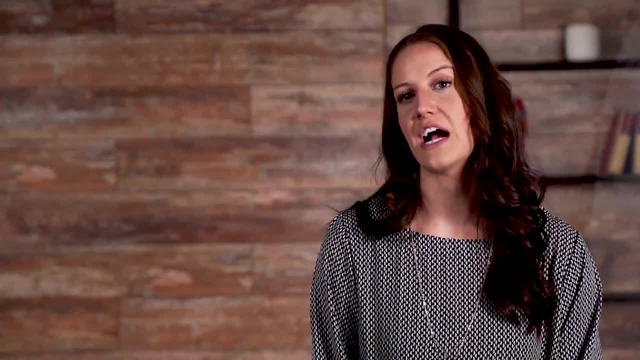 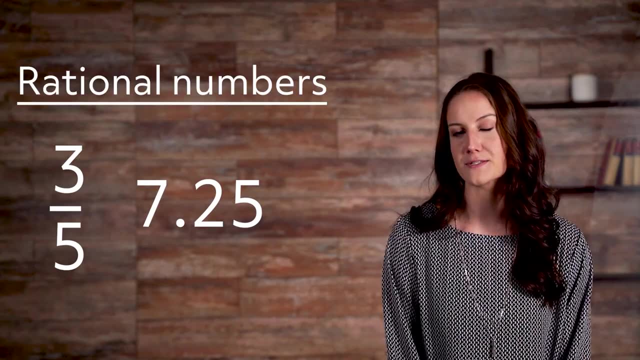 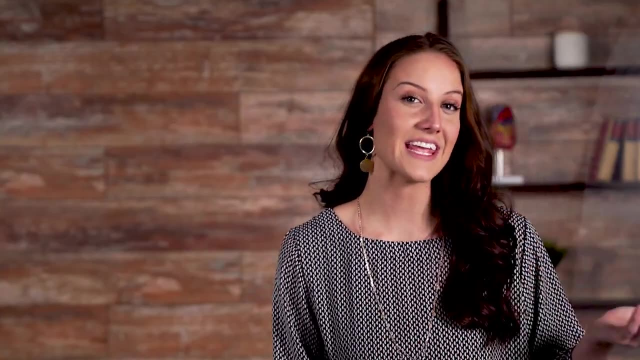 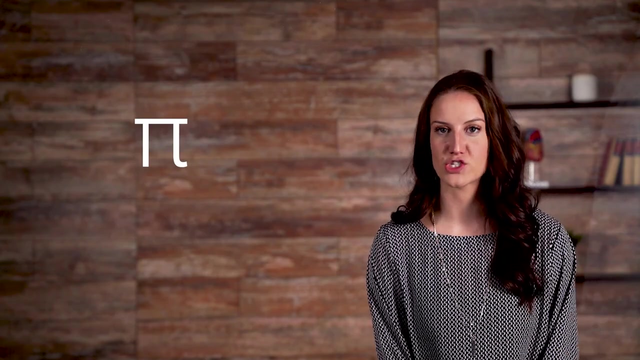 This group also includes fractions and decimals. That means that 3 fifths and 7.25 are rational numbers. Rational numbers can also be positive or negative. Rational numbers have opposites, which are called irrational numbers. These numbers can't be written as a simple fraction. Pi is the most famous irrational number. 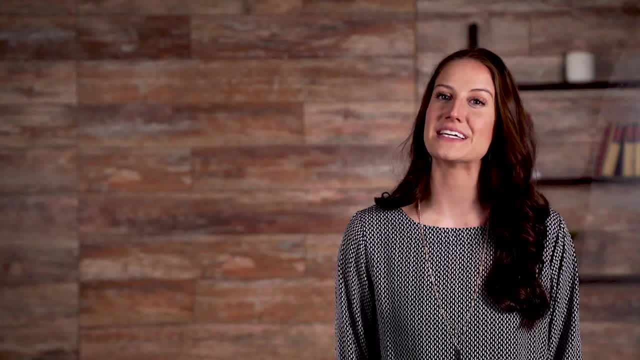 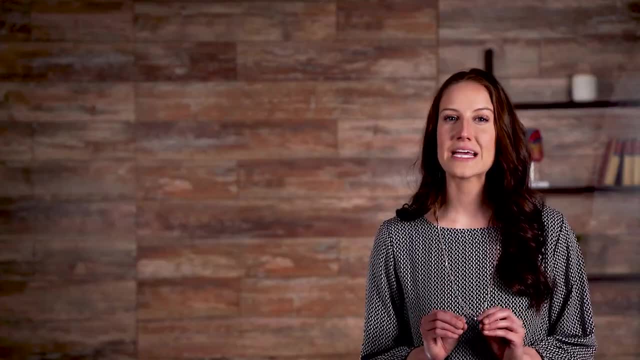 We have a close approximation of how to calculate pi, but it's just a clue. All Whole Numbers. Pi is a close approximation. Pi is renowned for going on and on forever. That's why it's an irrational number. You can't easily write it as a fraction. 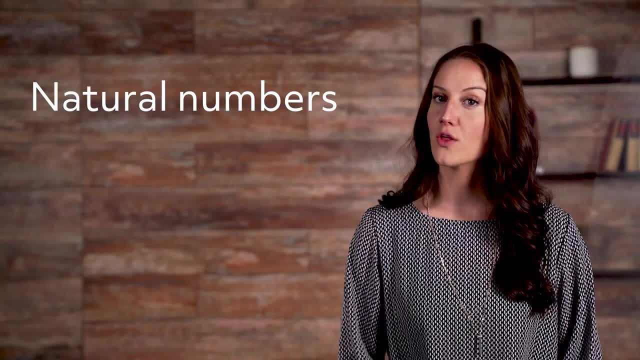 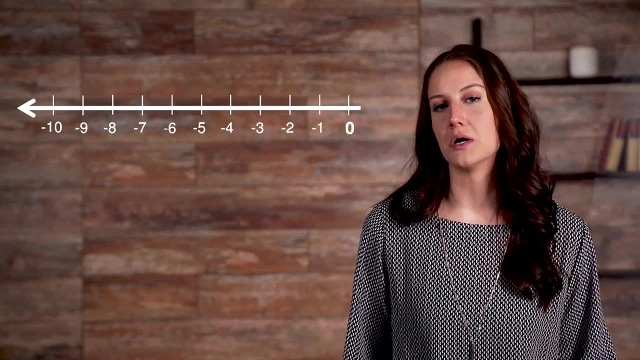 Natural Numbers. Natural numbers are those that are positive integers, although there is some debate as to whether natural numbers start at 0 or 1.. Negative numbers are exactly that: They are the numbers below 0.. There are several other number classifications as well. 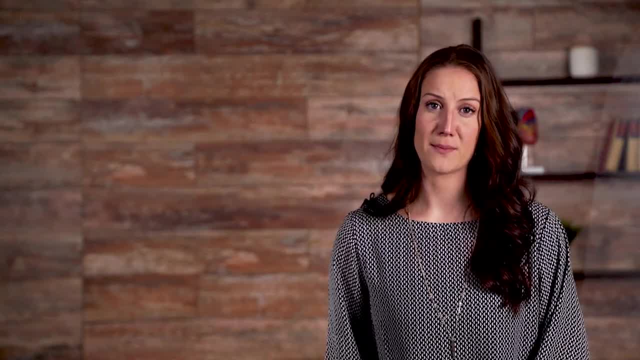 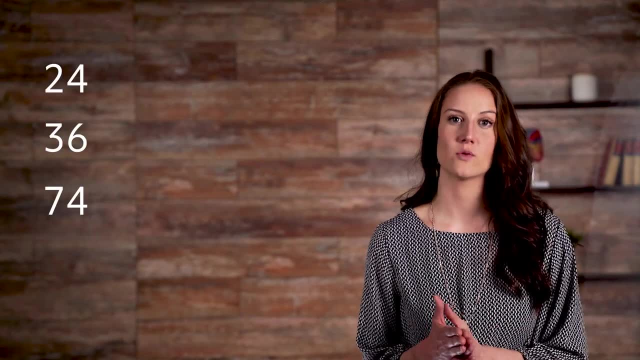 All Whole Numbers. Numbers are divided into even and odd numbers. If you can divide a number by 2, that number is even. So 24,, 36, and 74 are all even numbers, because if you divide them by 2, you get 12,, 18, and 37. 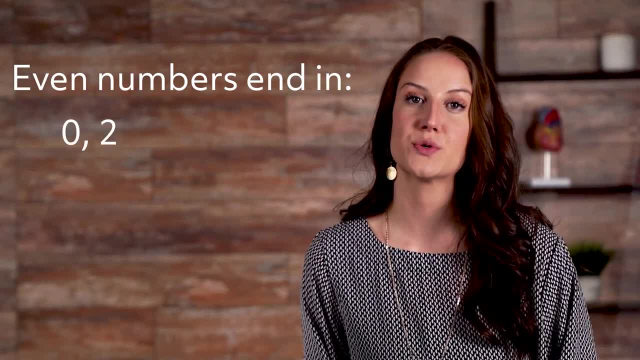 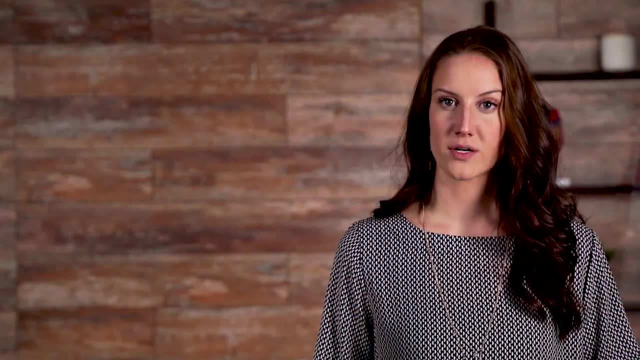 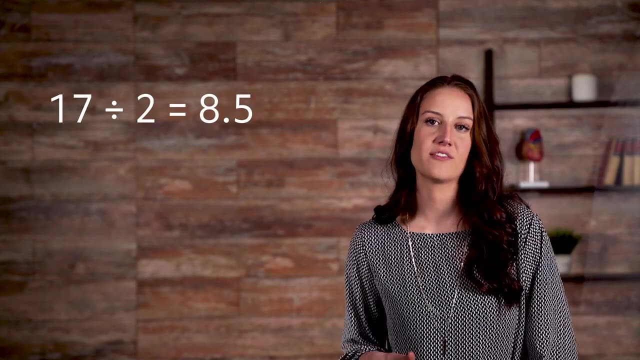 Even numbers always end with 0,, 2,, 4,, 6, or 8.. Odd numbers can't be divided by 2 and leave a whole number. Any odd number divided by 2 will leave a fraction. So 17 divided by 2 is 8.5.. 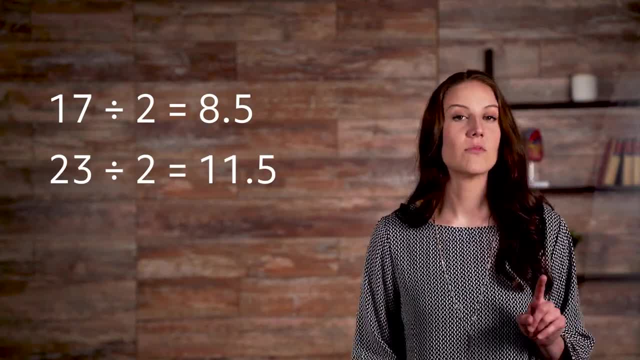 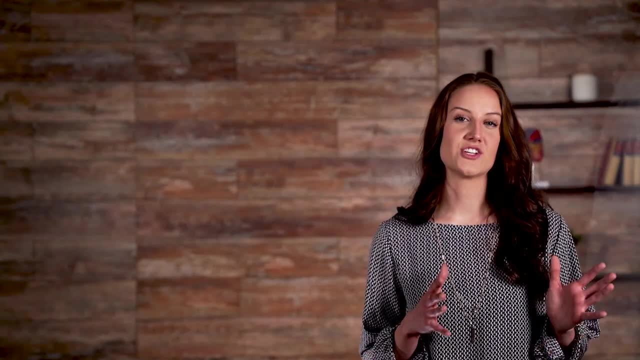 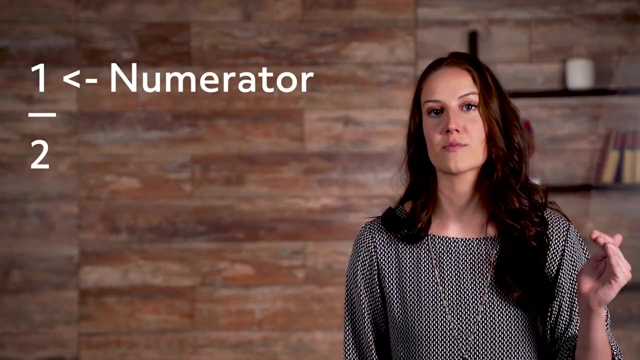 23 divided by 2 is 11.5.. All odd numbers will end in 1,, 3,, 5,, 7, or 9.. Numerators and denominators form fractions which are compromised of two integers. The number on top is the numerator, the number on the bottom is the denominator. 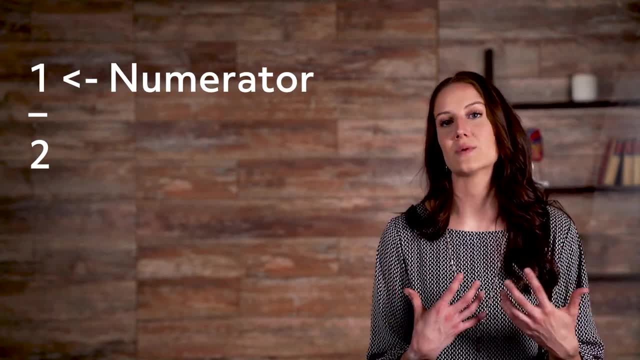 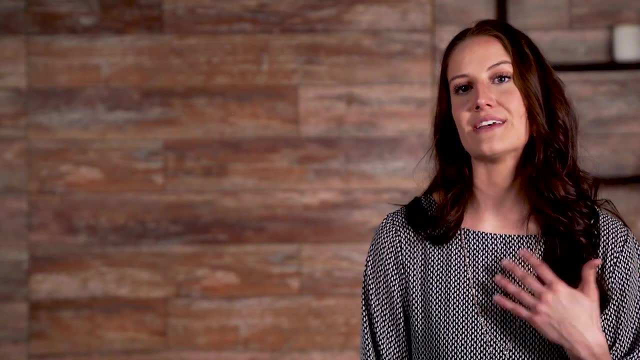 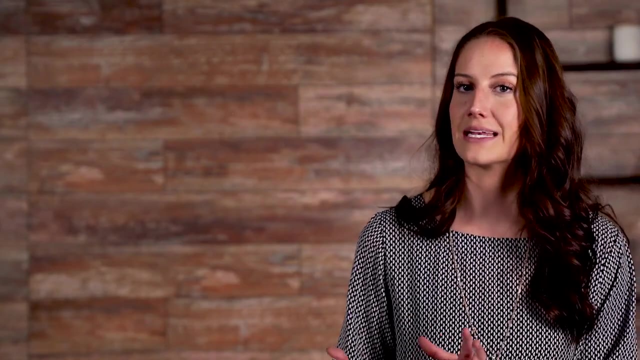 The numerator- the top number shows how many parts we have. The denominator- the bottom number shows how many parts make a whole. Let's say you have 6 apples and 3 of the apples get eaten. The number of apples you have left over would be displayed as 3 sixths. 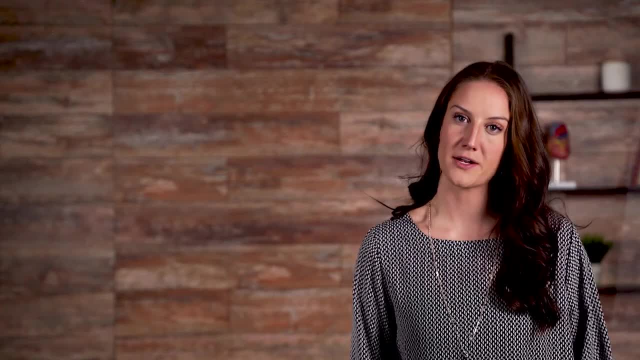 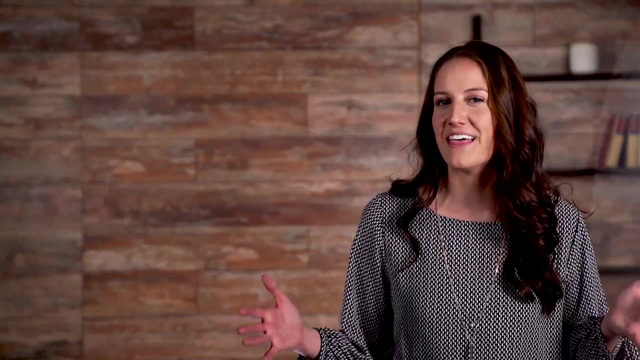 You would then divide 3, the top number, into 6, the bottom number, to determine the percentage of remaining apples. In this case the number is 50%. So that's our look at numbers in their classification. So that's our look at numbers in their classification. 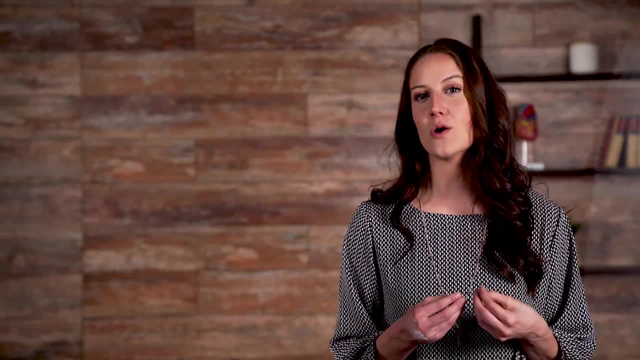 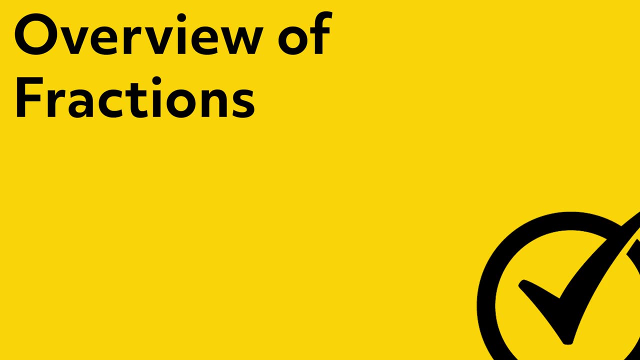 So that's our look at numbers in their classification, From whole numbers to irrational numbers. we need to know what to call numbers so we can know what they mean. From whole numbers to irrational numbers. we need to know what to call numbers so we can know what they mean. 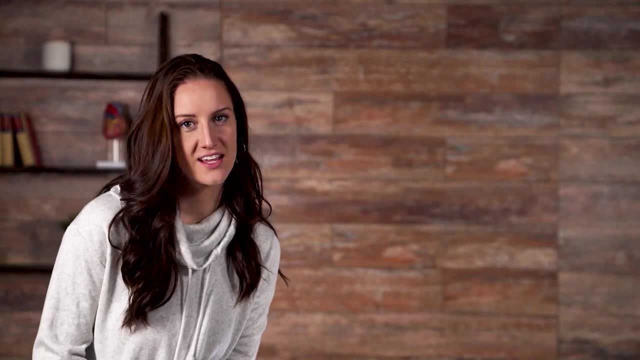 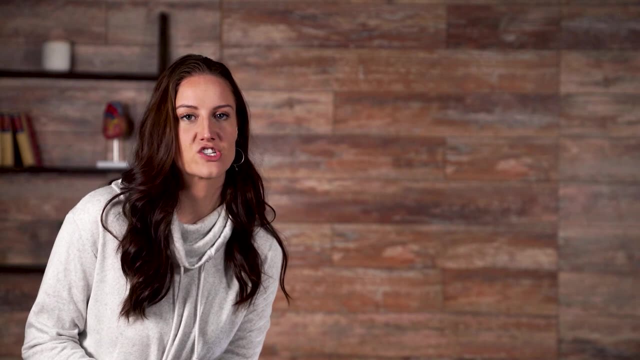 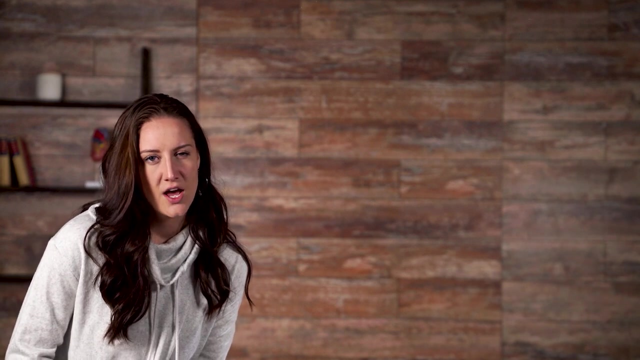 Hey guys, welcome to this Mometrix video on fractions. Fractions can be simple or complex. In this video we'll cover different types of fractions and how to add fractions with different denominators. So what is a fraction? A fraction is a part of a number. 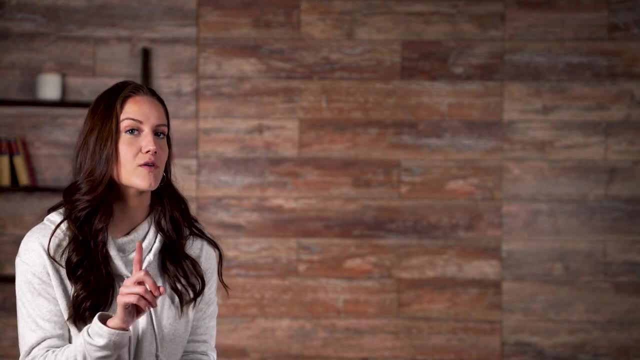 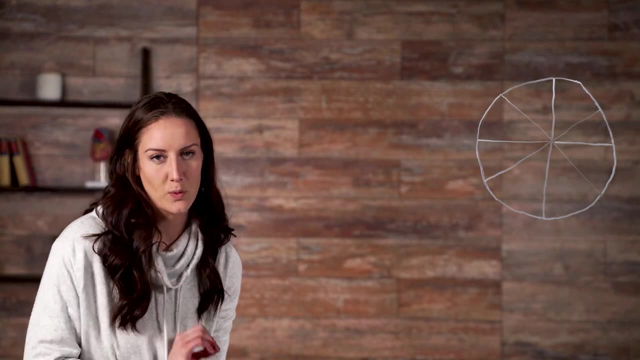 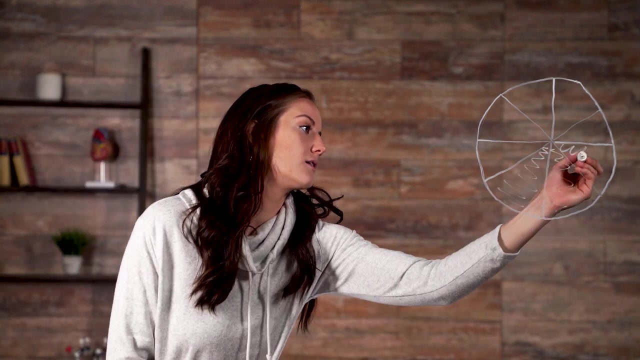 A fraction is a part of a whole, which means a fraction can never be a whole number. Think of it like this: Our circle is divided into 8 equal pieces. Let's say 3 pieces were filled in. Let's say 3 pieces were filled in. 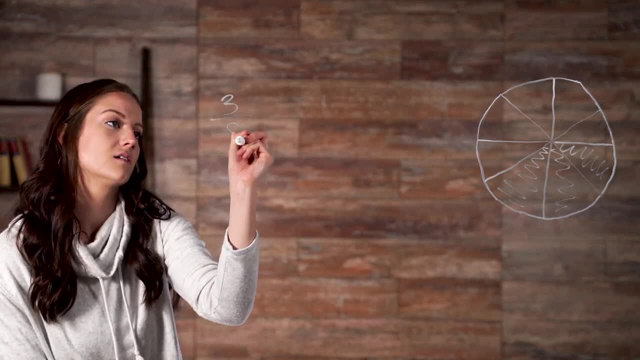 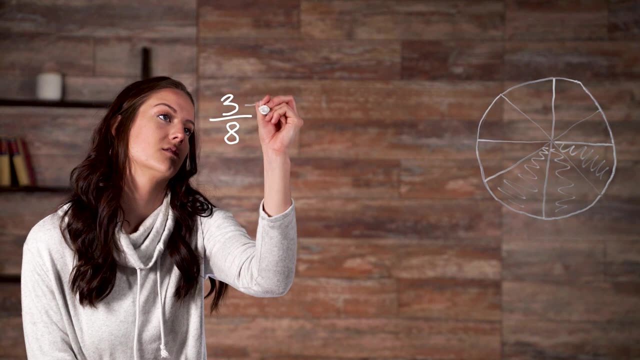 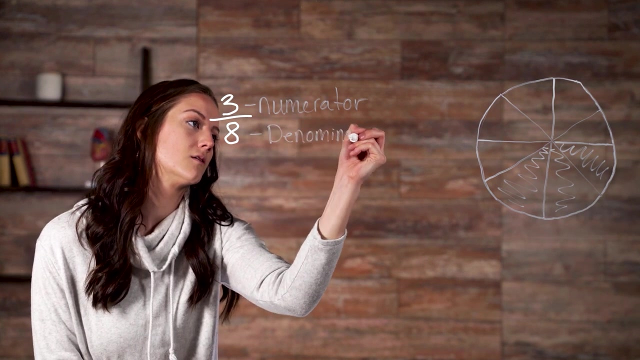 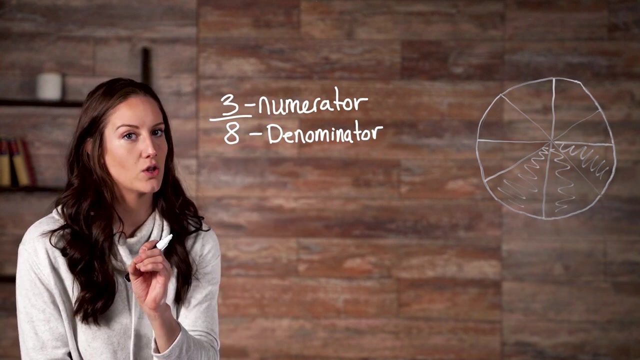 That means that 3 eighths of our circle is filled in. The top number is called the numerator And our bottom number is called the denominator. When saying fractions out loud, the denominator will usually be spoken as the ordinal version of the number. 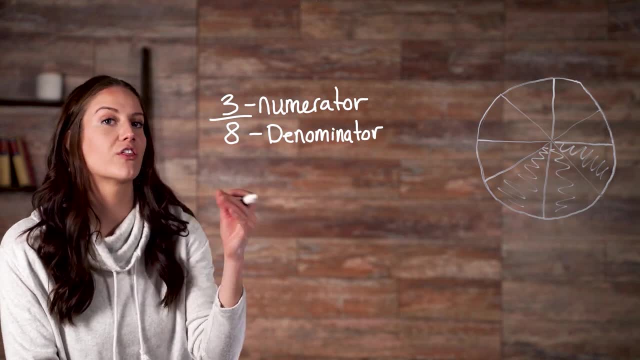 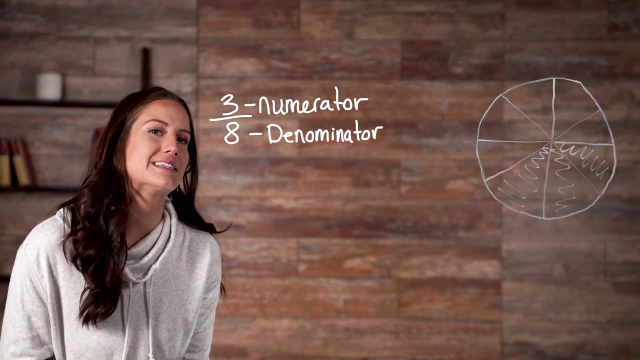 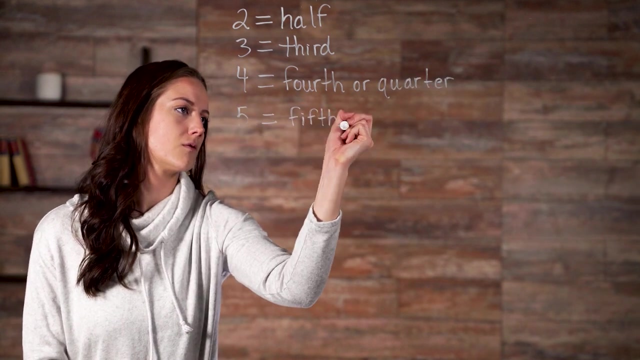 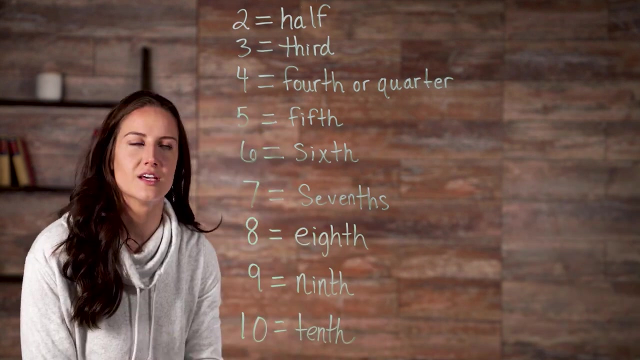 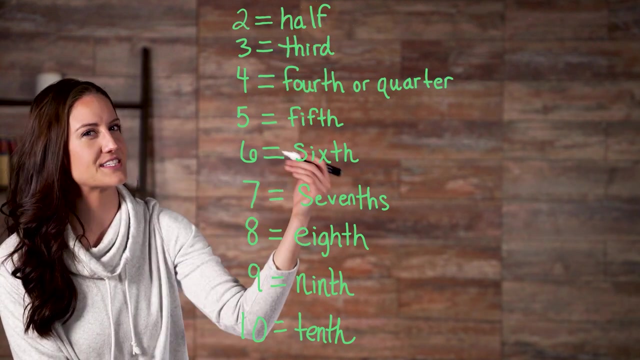 You would say eighth instead of eight, or third instead of three. Let's take a look at a list of our denominators and see how we would say them. As you can see, there are a couple of exceptions. If our denominator is 2,, you could say half instead of second. 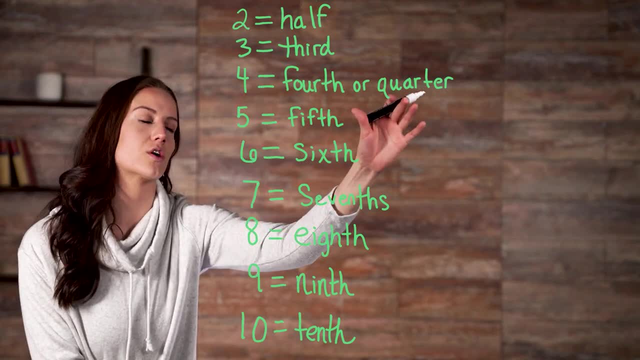 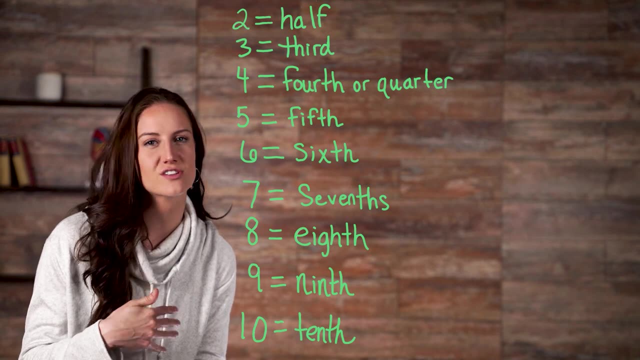 Or if our denominator is 4, you can say quarter instead of fourth, But either one is acceptable. Hopefully that helps you to understand how fractions are defined and also how fractions are defined, How to actually say them out loud. 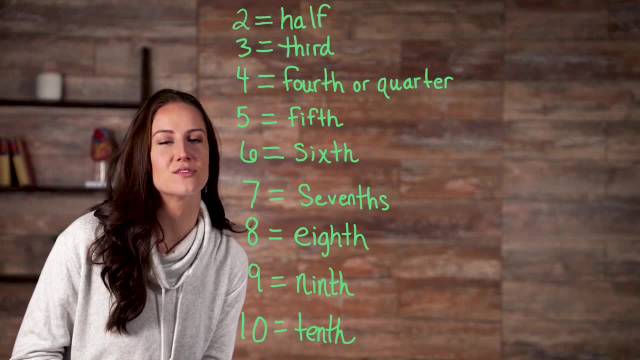 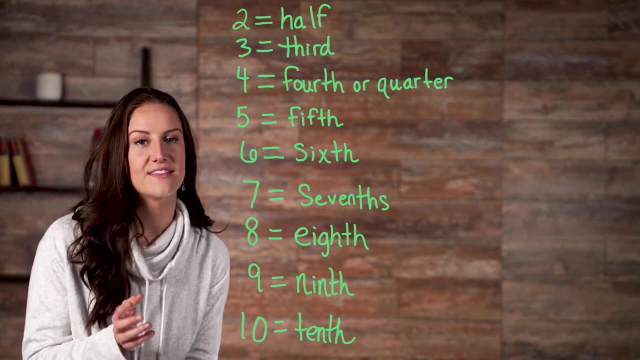 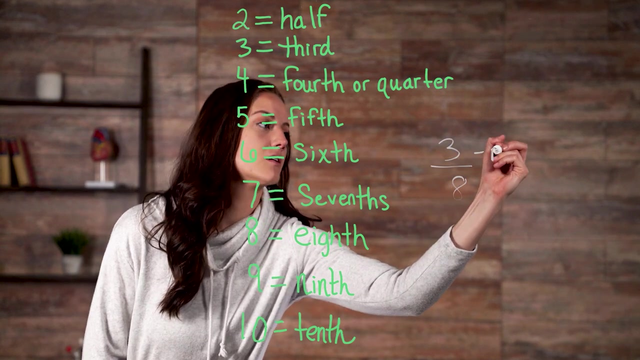 But there are different types of fractions. Let's take a look at those. First, we have a proper fraction. A proper fraction always has a numerator, which we looked at, that is smaller than the denominator. Our example that we used before 3 eighths. 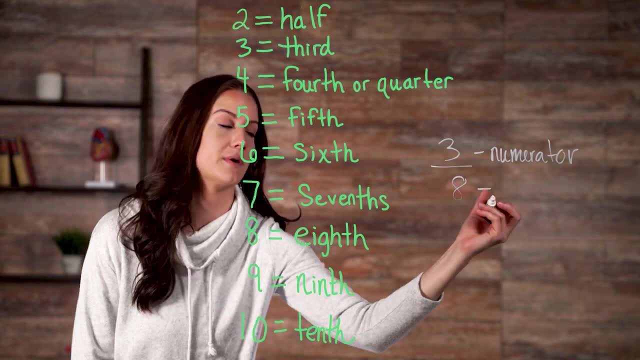 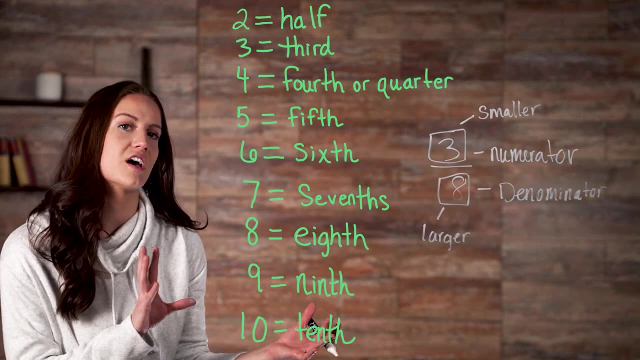 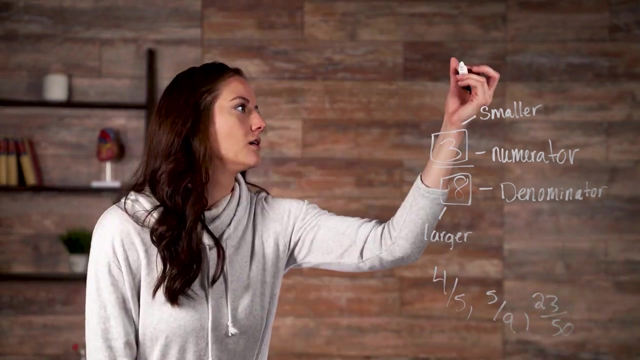 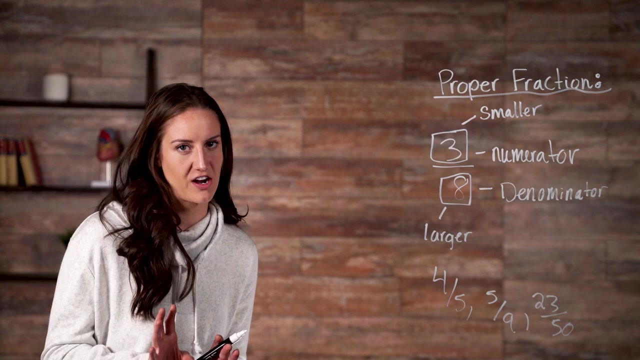 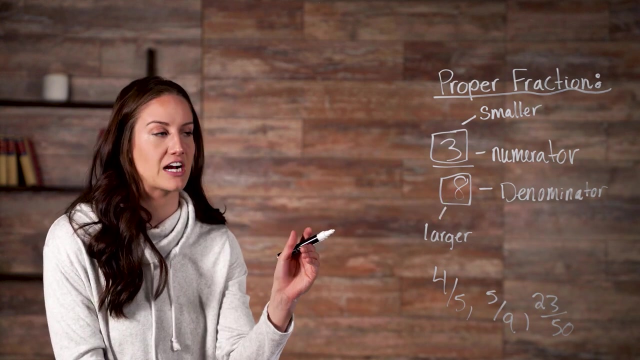 So our numerator 3, is smaller than our denominator 8.. Some other examples of proper fractions include 4 fifths. An improper fraction is the opposite of a proper fraction, in that the numerator is larger than the denominator. So while 3 over 8 is a proper fraction, 8 over 3 is an improper fraction because the 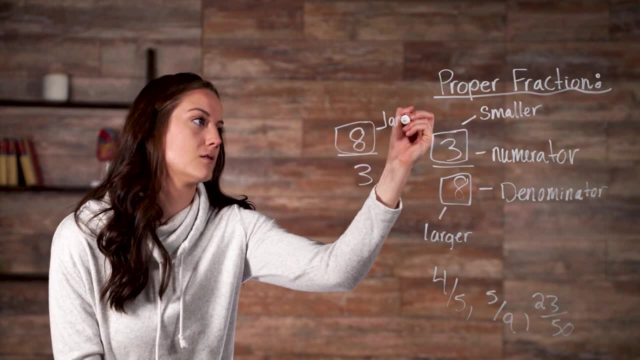 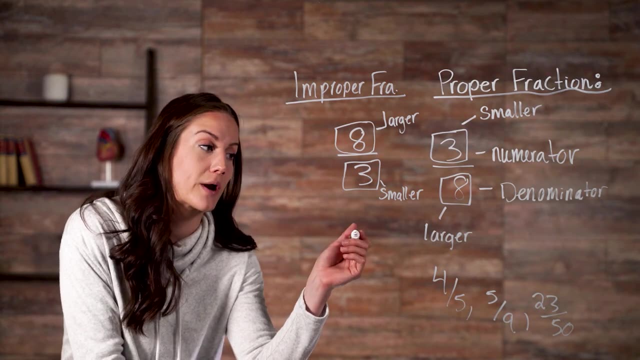 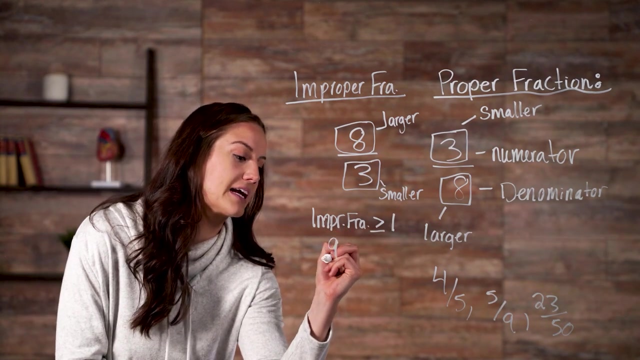 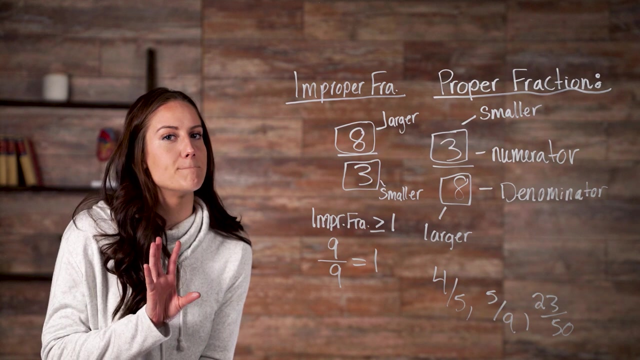 numerator is larger than the denominator, Improper fractions are always equal to or greater than 1.. That means that 9 over 9 is an improper fraction, since it is equal to 1.. There are also mixed fractions, which contain a whole number in a proper fraction. 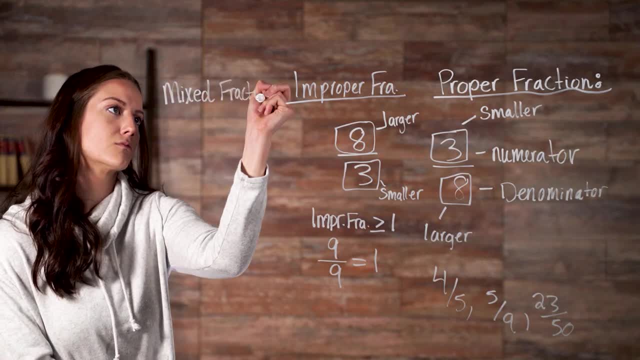 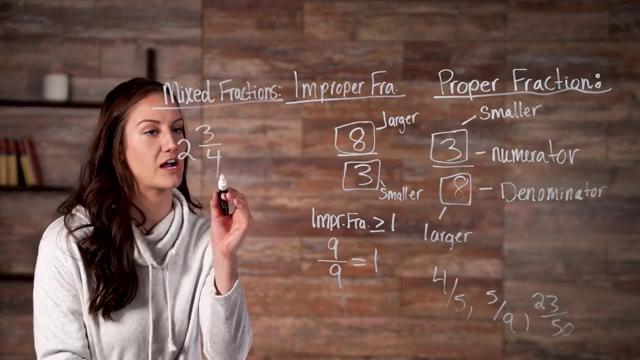 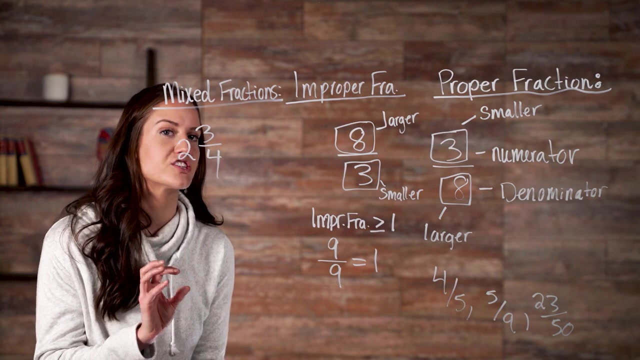 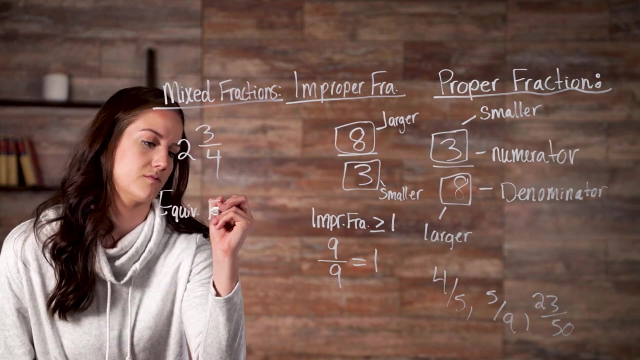 Here is an example. Note that the whole number 2, is followed by the proper fraction, 3 over 4.. We also have equivalent fractions. Equivalent fractions are two different fractions that name the same number. For example, 6 eighths and 3 fourths look the same. 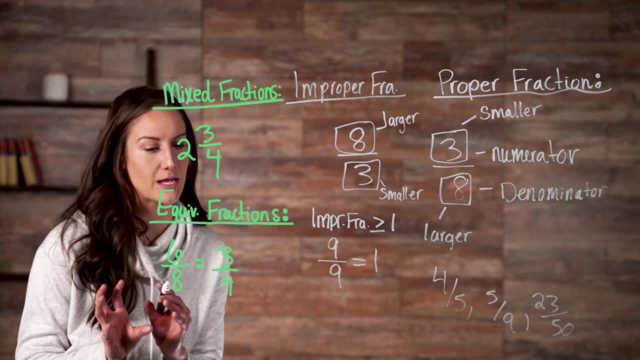 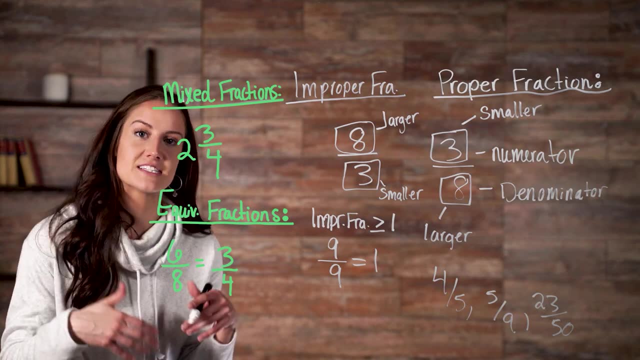 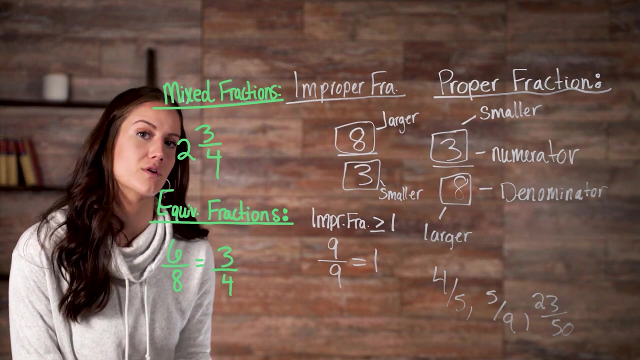 3 fourths is just a simplified or reduced version of 6 eighths. You just divide the numerator and the denominator by 2 to get 3 fourths. Now that we know the different types of fractions, we can explore how to add them. 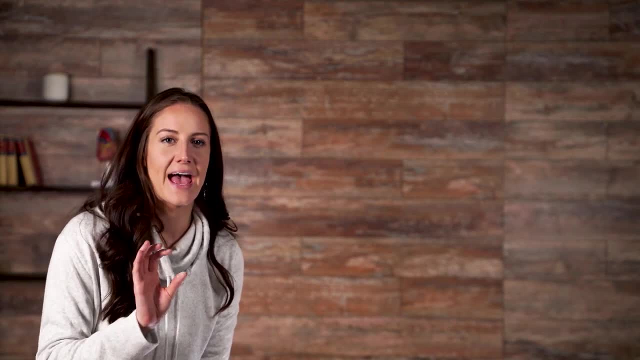 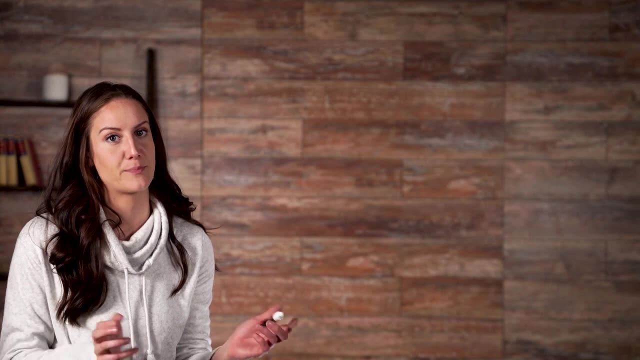 If two fractions have the same denominator, adding is a breeze. You just add the numerators together and that gives you the answer. For example, P2 and L2 have the same denominator. So notice what we did to get 3 fourths. 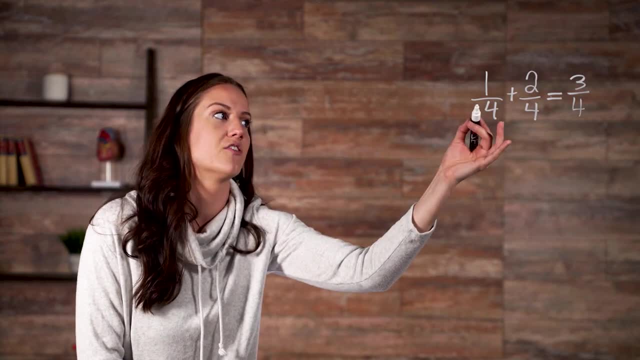 We added a numerator and the denominator together. If 2 fractions have the same denominator, adding is a breeze- Just add the numerators together and that gives you the answer. For example, All we had to do was add from our first fraction the 1 from our numerator and from our second fraction the 2 from our numerator. 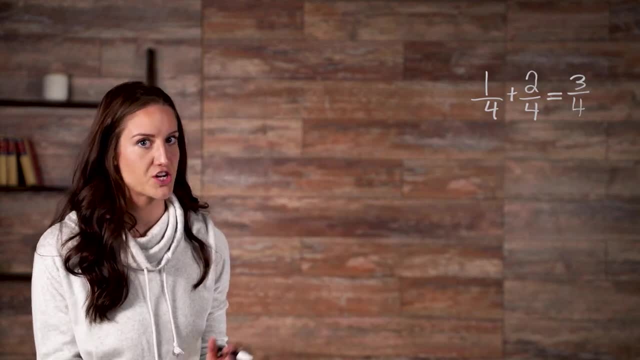 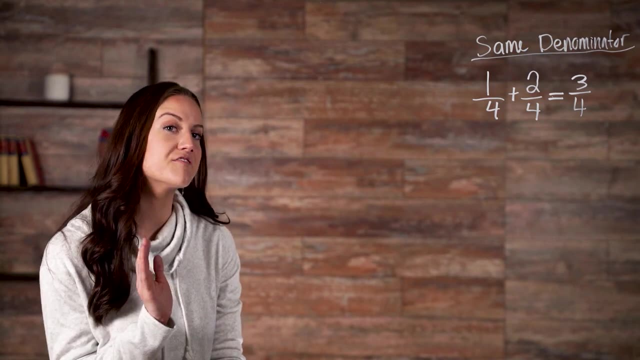 Add them together to get 3, and we just bring over our 4 from the denominator. Simple. But what happens if the denominators are different? Well, in that case you have to convert the denominators to be the same. 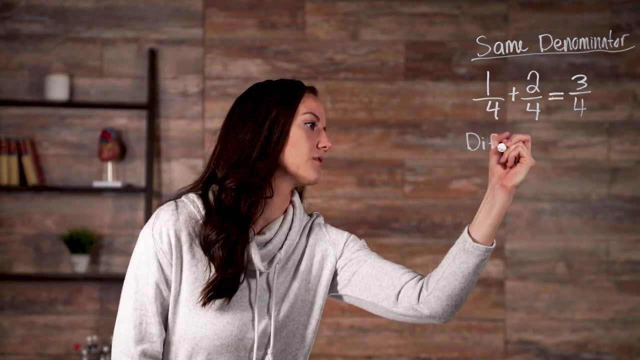 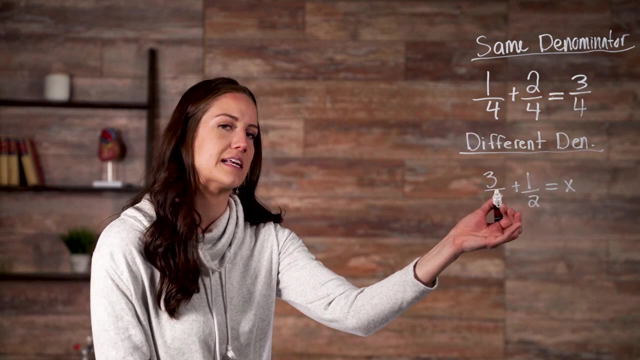 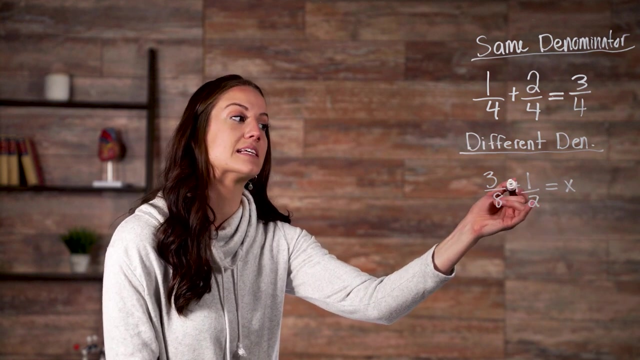 So let's take a look at an example. You can't really simplify 3 eighths into anything that would easily add with 1 half. But we can do something with 1 half that we could easily add with 3 eighths, and that's multiplying 2 by 4, which would give us 8.. 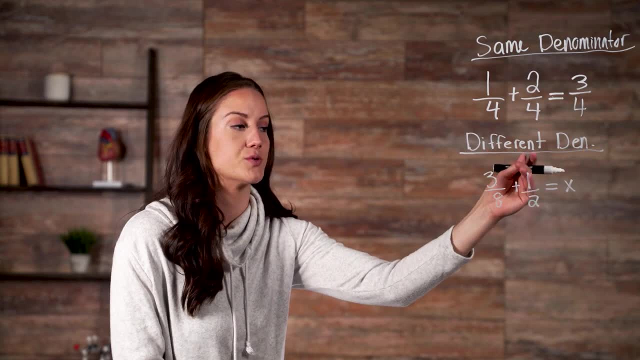 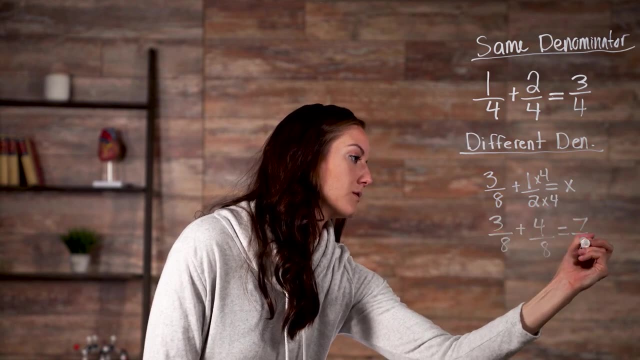 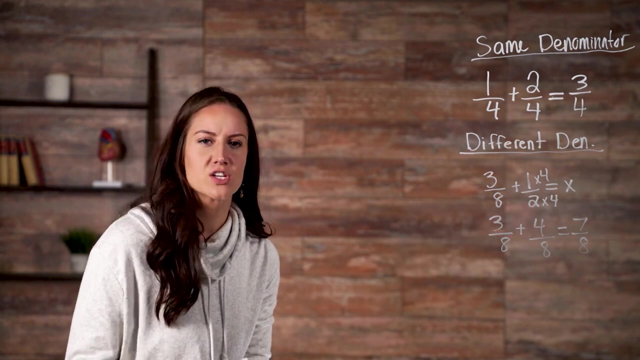 But whatever we do to our denominator, we also have to do to our numerator, So that would look like this. So our equation now becomes: 3 eighths plus 4 eighths equals 7 eighths. Subtraction works the same way. 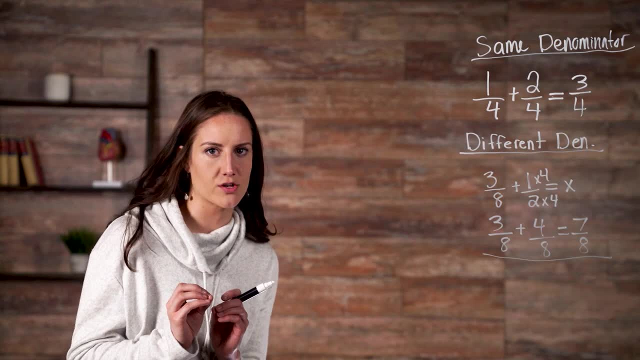 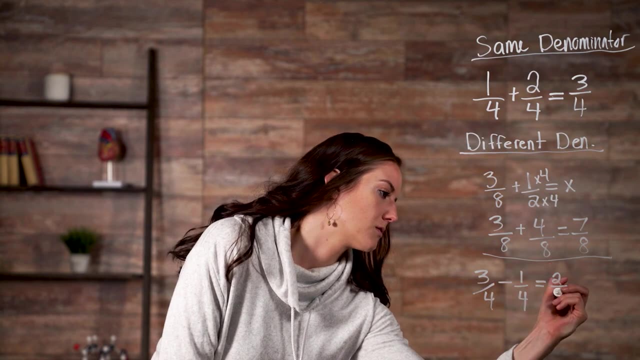 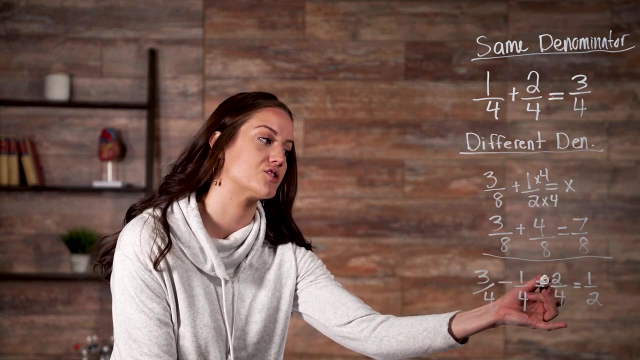 If you're subtracting fractions with the same denominator, you can just subtract the top numbers, like in this example. So in this example, all we had to do was subtract our top numerators here, which gave us 2 fourths. 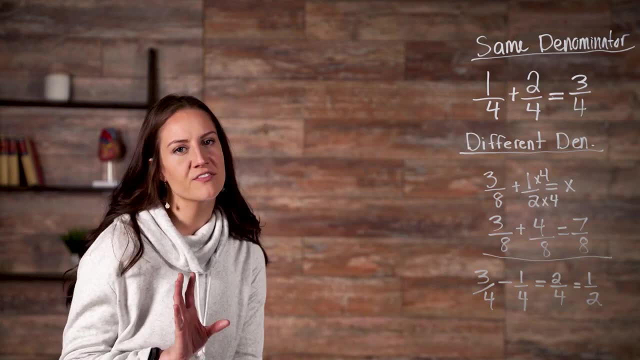 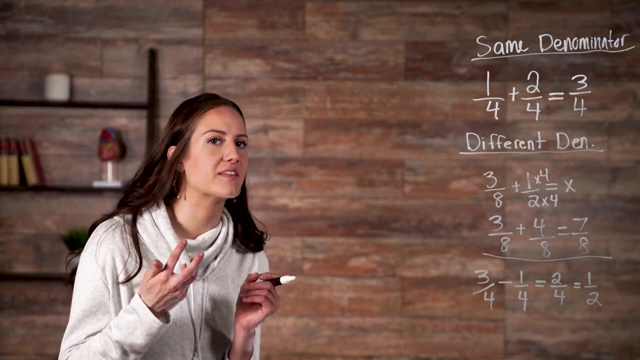 So we have 1 third of the denominator. Now we're going to be subtracting them with the denominator. We're going to be subtracting the denominator by 1 half, which simplifies to 1 half. Simplifying numbers just makes them easier to work with. 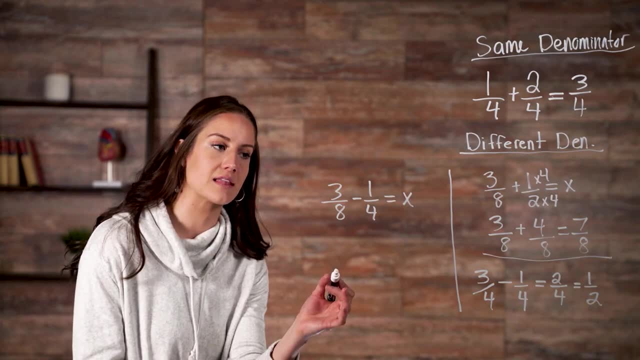 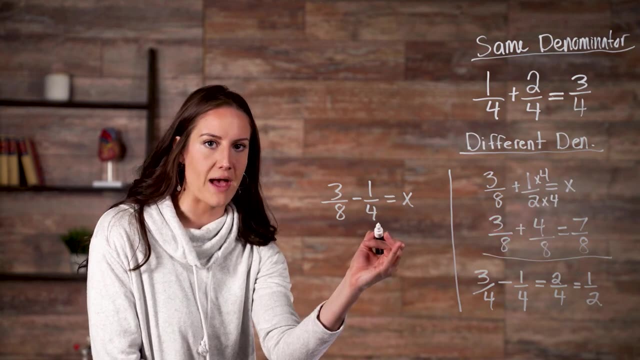 But if you're subtracting with a different denominator, you have to make the denominators match, For example. So in this example, 3 eighths minus 1 fourth is equal to x. We're kind of looking at the same issue like we did over here. 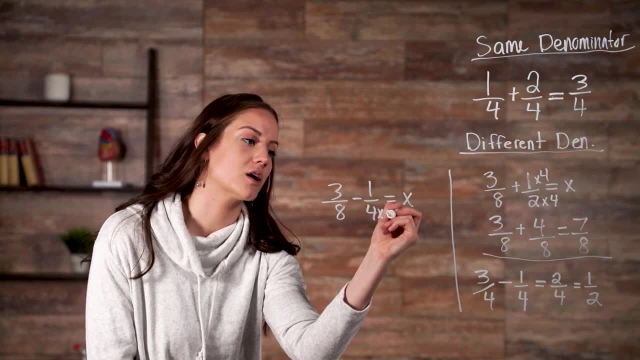 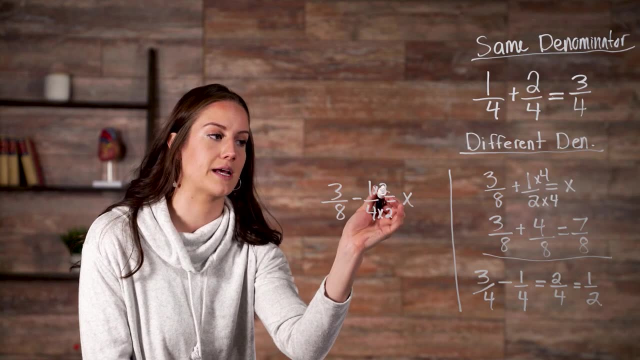 We need our denominators to match. In this case, we can multiply 4 times 2, but remember, we have to do the same thing that we do to the denominator, we must do to our numerator. So we can multiply it times 2, and then here's what we get. 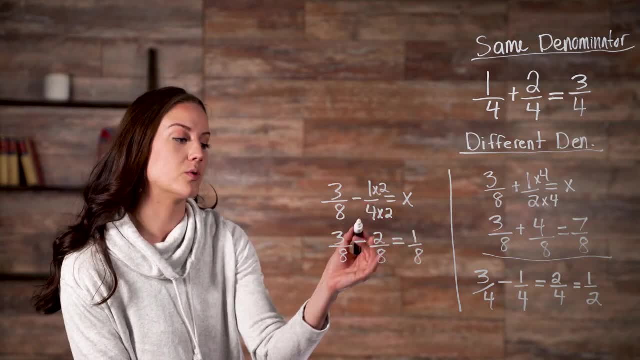 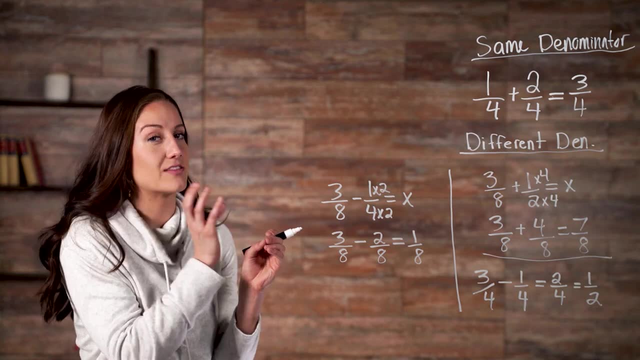 So once we multiply our second fraction here by 2, we get 3 eighths minus 2 eighths, which gives us 1 eighth. So these problems were pretty easy because they had either the same denominator or were just really easy to convert. 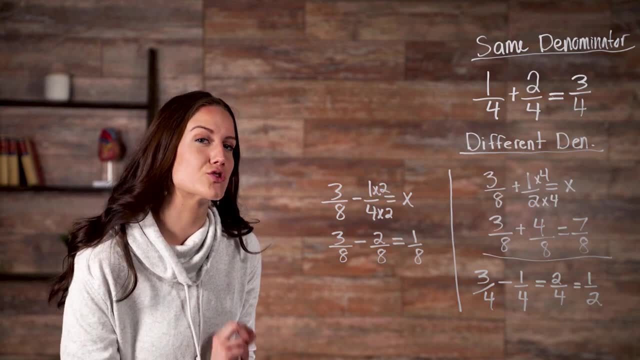 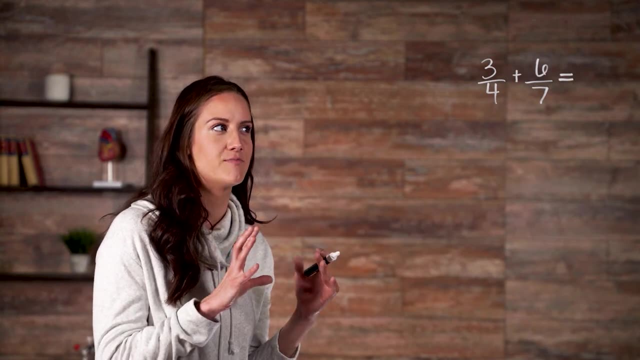 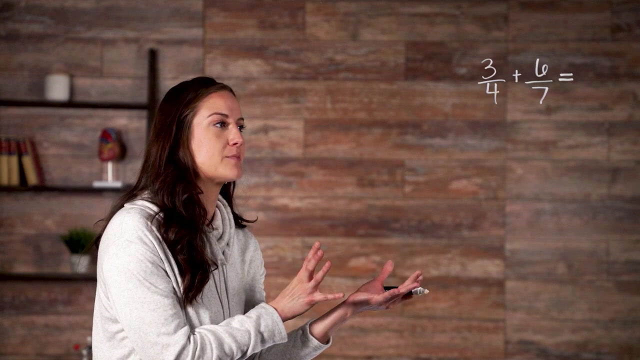 But let's look at one more equation that's a little trickier. So at first glance it doesn't look like these numbers have much in common, such that we would be able to multiply or divide 4 by anything to get 7, or 7 by anything to get 4.. 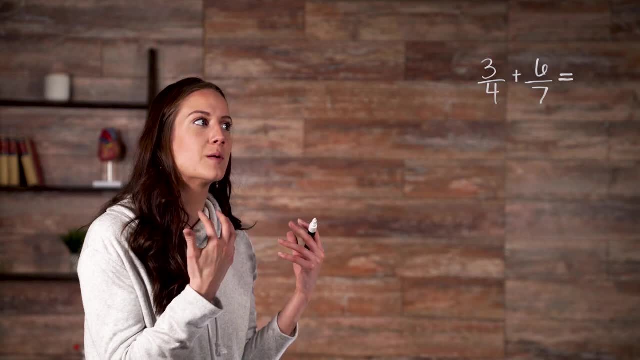 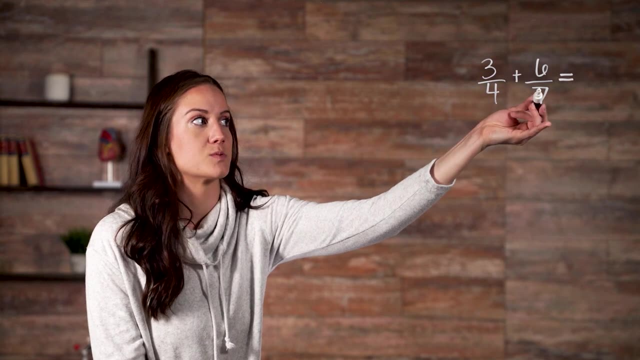 So, a lot of the times when you have problems like this, what you end up having to do is multiplying this fraction by the denominator of the other fraction, And likewise, We would multiply this fraction by the denominator of this fraction. So here's what that looks like. 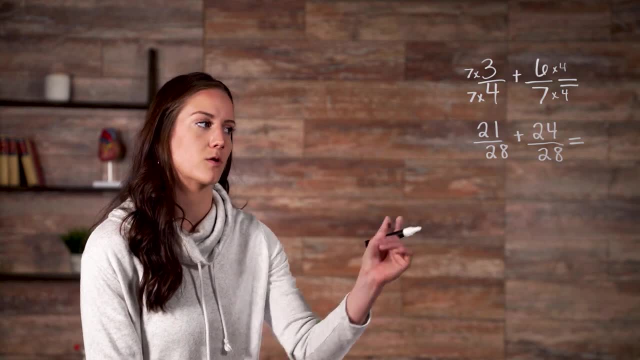 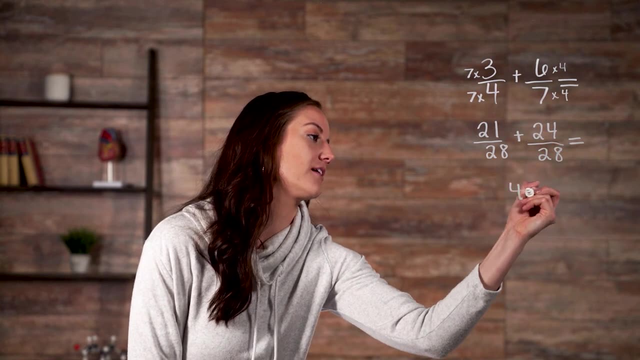 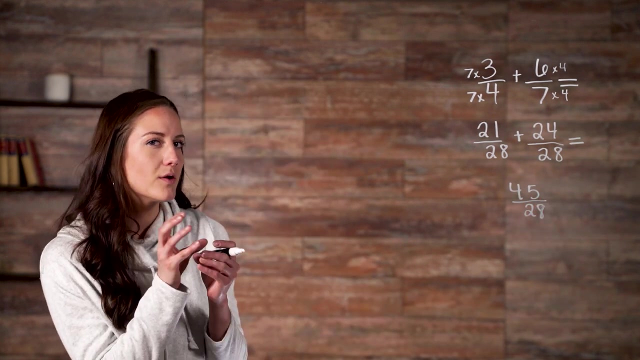 So after our multiplication, we end up getting a common denominator, which is 28.. So now all we have to do is add our numerators together, which that gives us 45 over 28.. And that's our answer. With this calculation, we found that the denominator of the denominator is 28.. 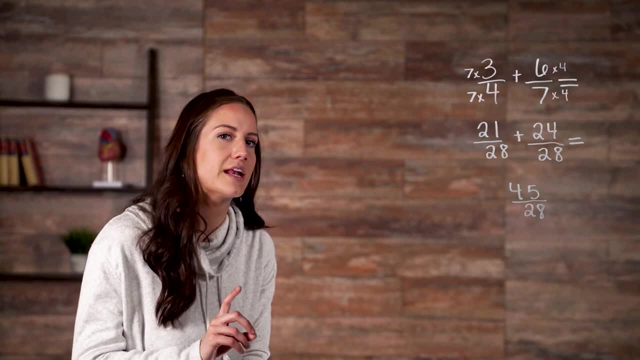 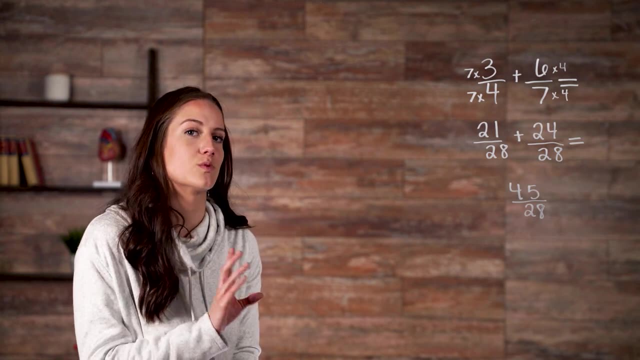 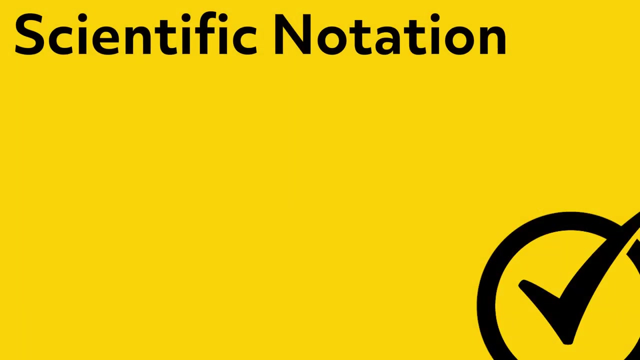 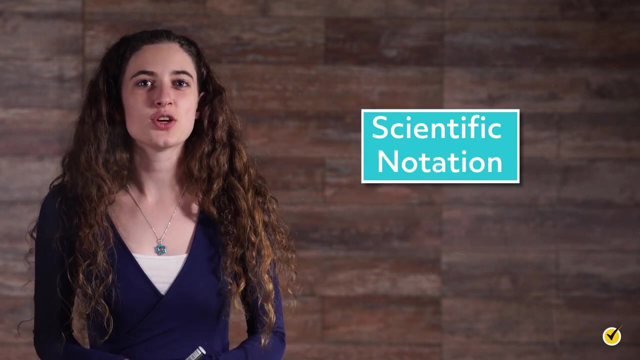 And the least common denominator is the smallest common number between denominators. Any time you perform a calculation with different denominators, you must find the least common denominator to solve the problem. Hi and welcome to this video about scientific notation. In this video we will explore what scientific notation is and how to write and compare. 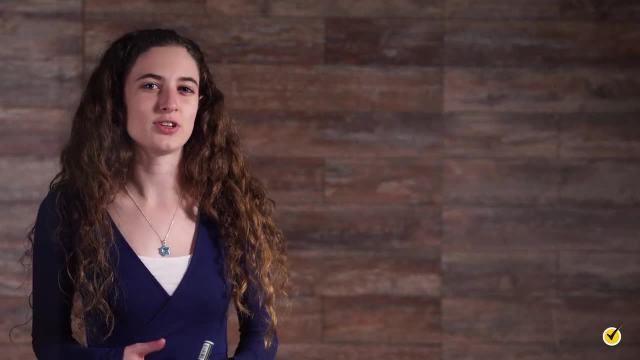 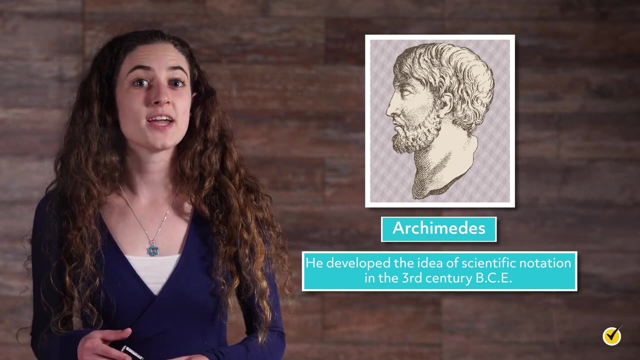 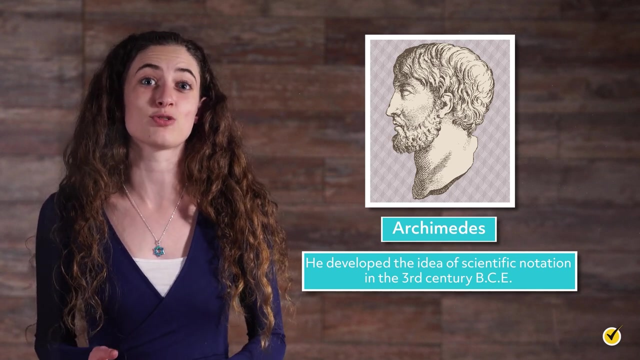 numbers in scientific notation. First, what is scientific notation? The idea of scientific notation was developed by Archimedes in the 3rd century BCE, where he outlined a system for calculating the number of grains of sand in the universe, which he found to be 1, followed by 63 zeros. 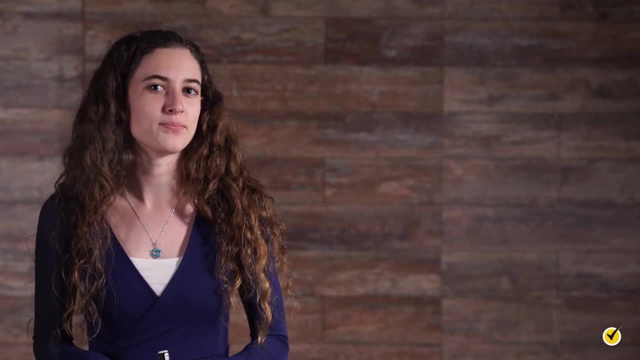 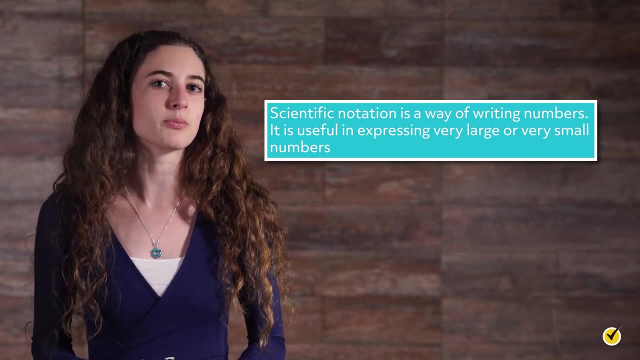 His work was based on place value, a novel concept at the time. Scientific notation is simply a way of writing numbers. It is especially useful in expressing very large or very small numbers because it is shorter and more efficient and it shows magnitude very easily. 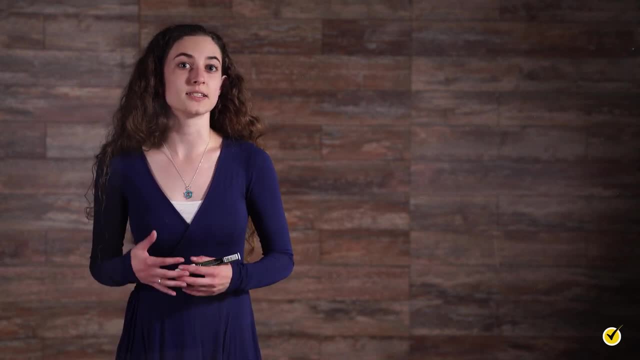 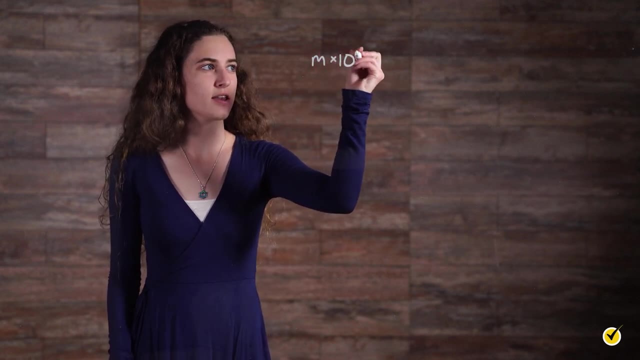 Every real number can be written as a product of two parts: a decimal part times an integer power of 10.. M times 10 to the n where 1 is less than or equal to m which is less than 10,. and. 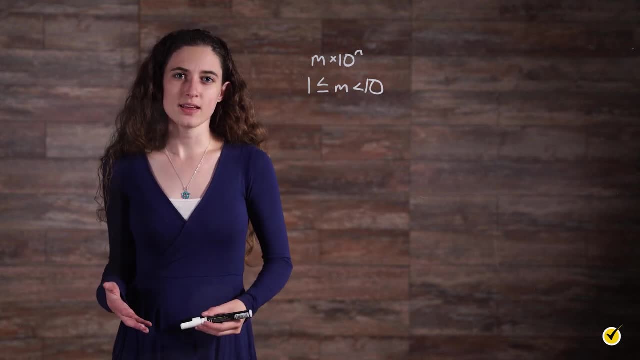 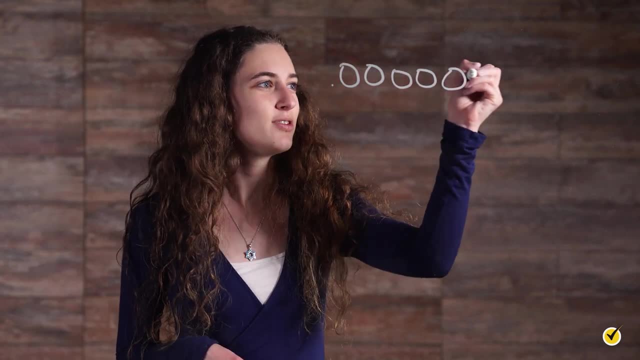 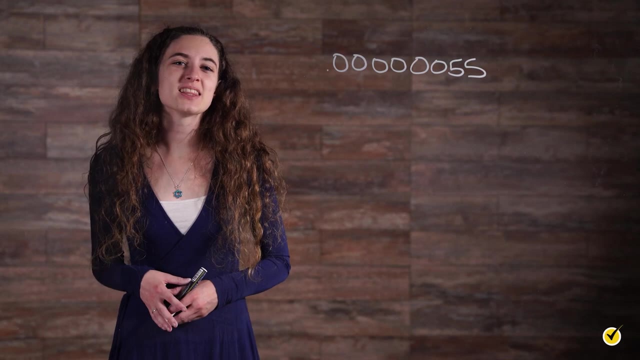 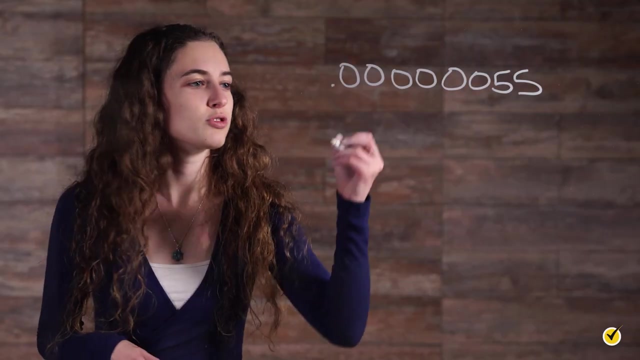 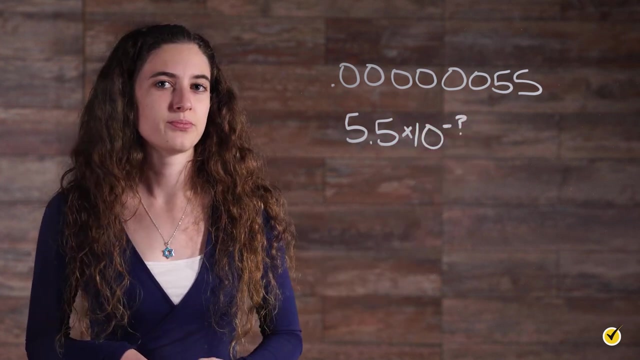 zero, zero, zero, zero, zero, five, five meters. Let's see this in scientific notation. We begin the same way as with large numbers: creating the decimal from the chunk bookended by non-zero numbers. Our result will resemble 5.5 times 10 to the negative something power. 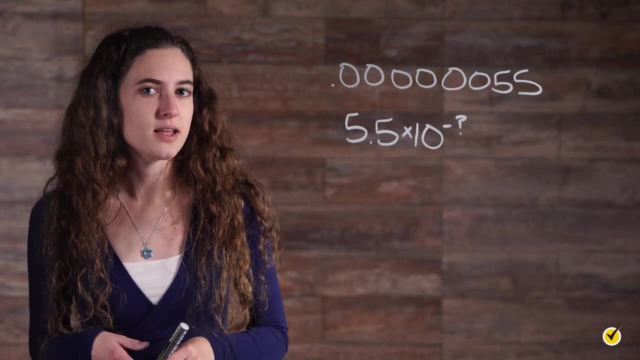 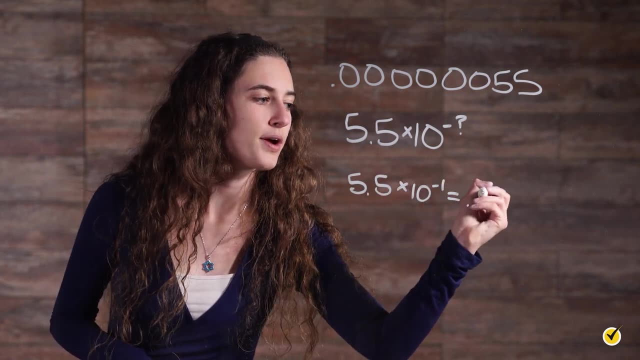 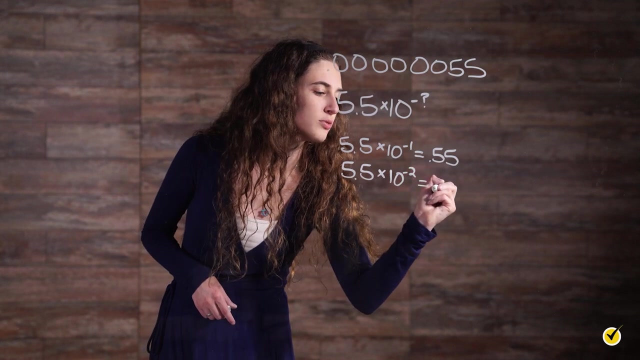 Now we count the number of times our decimal is divided by 10.. 5.5 times 10 to the negative, 1 is equal to 0.55.. 5.5 times 10 to the negative, second power is equal to 0.055.. 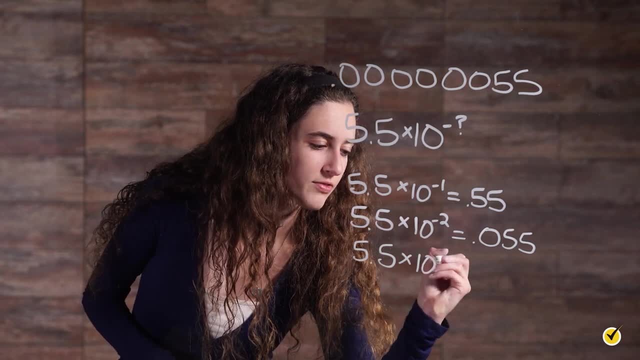 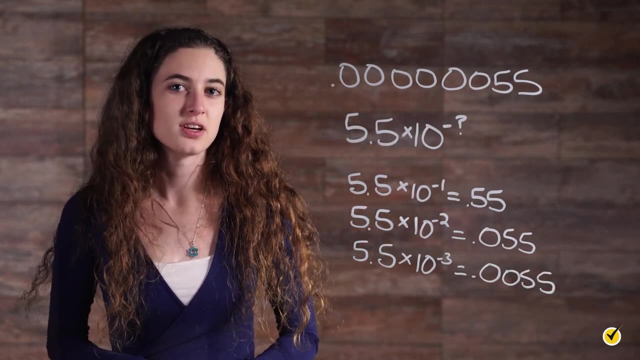 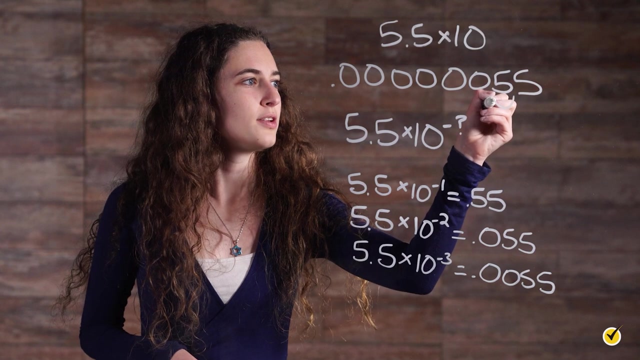 5.5 times 10 to the negative third power is equal to 0.0055.. And 6.5 times 10 to the negative third power is equal to 0.0055.. And so on and so on, until we reach 5.5 times 10 to the 1,, 2,, 3,, 4,, 5, 6, 7 negative seventh. 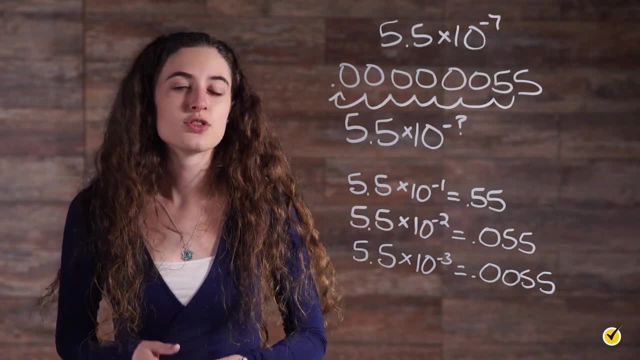 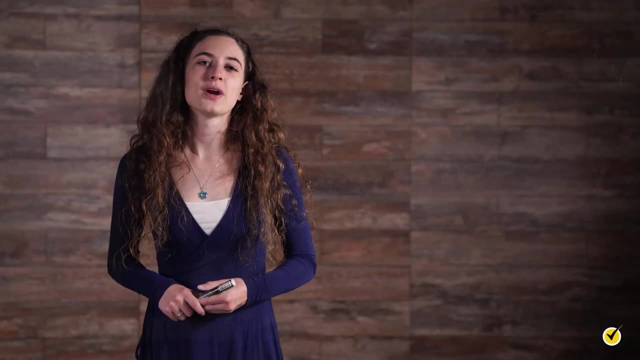 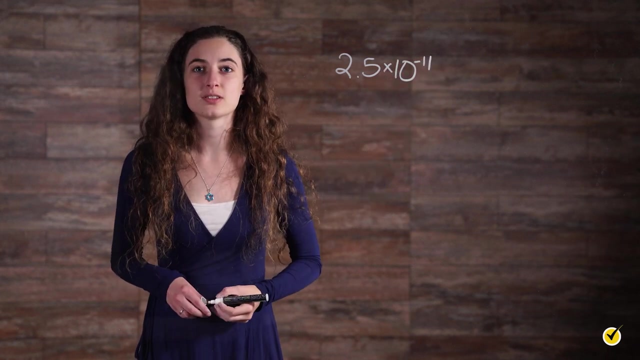 power. So in scientific notation the wavelength of green light can be expressed as 5.5 times 10 to the negative seventh meters. The radius of a hydrogen atom is 2.5 times 10 to the negative seventh meters. We can express this in standard form by starting with the decimal part 2.5 and dividing by 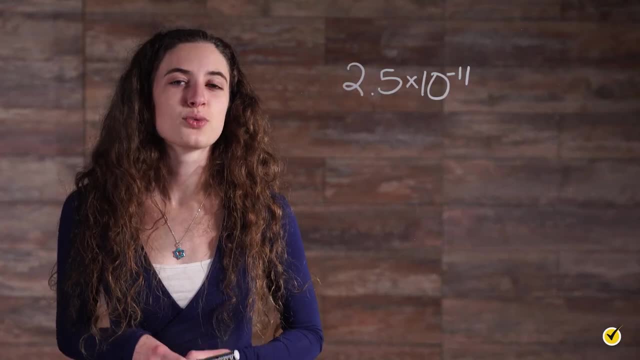 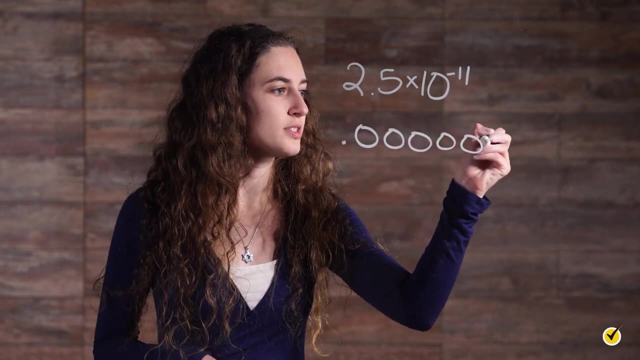 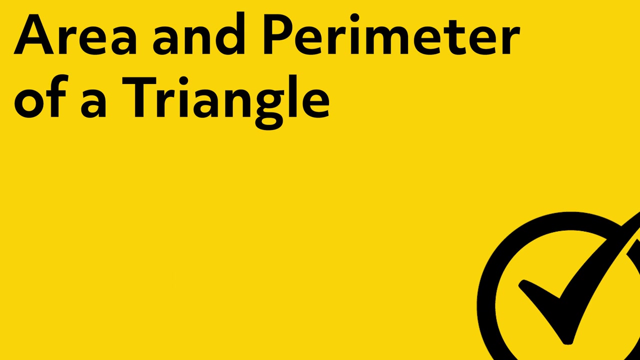 10, a total of 11 times. This tells us that the radius of a hydrogen atom is 0.00000000000025 meters. To get started, we will first have to find the value of the value of the value of the number of times. the value of the number of times. the value of the number of times. the 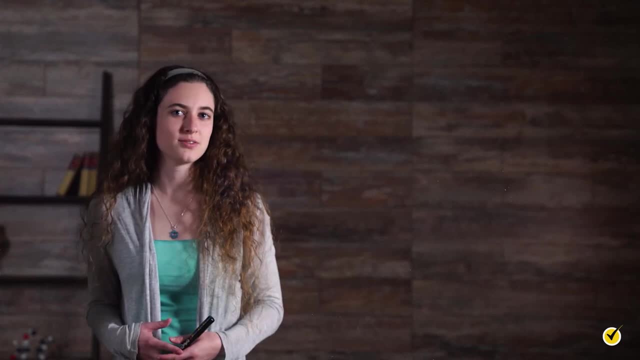 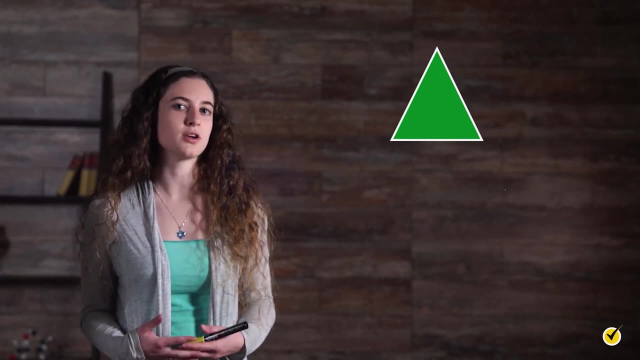 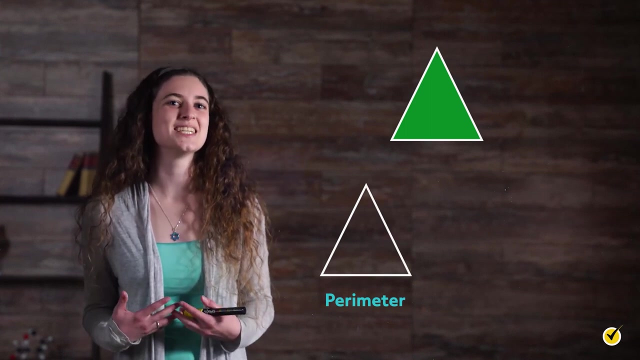 To get started, let's quickly review what perimeter and area measure. Imagine we have a triangular shaped yard. If we wanted to build a fence around our yard, we'd need to know the distance around the yard. This is the perimeter. If we wanted to buy sod for our yard so that we could have a lovely green space, we'd 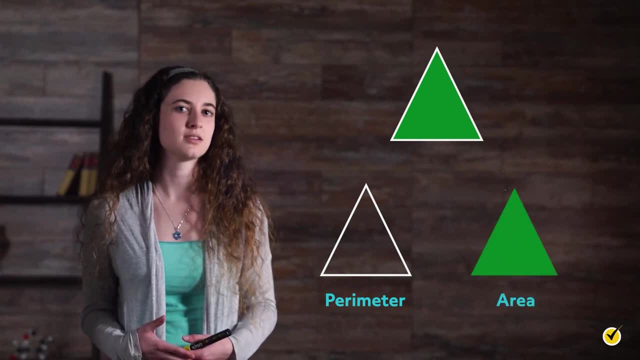 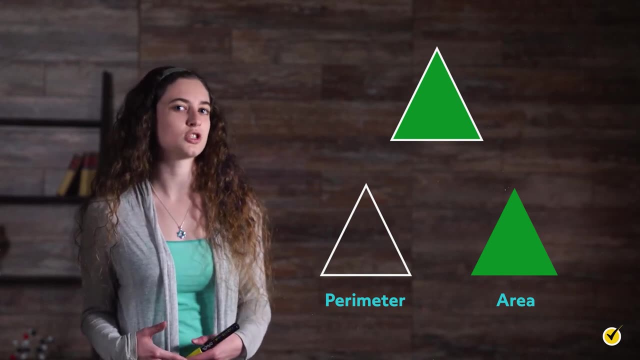 need to know the area of the yard so that we could buy the correct amount, And while it might be a bit unusual to have a yard that is the shape of a triangle, you might have part of a yard that you want to fence or sod shaped like a triangle. 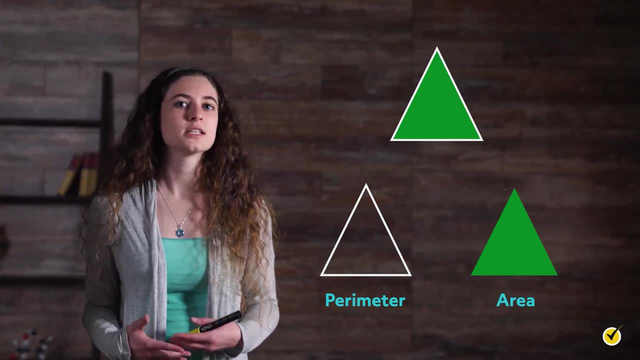 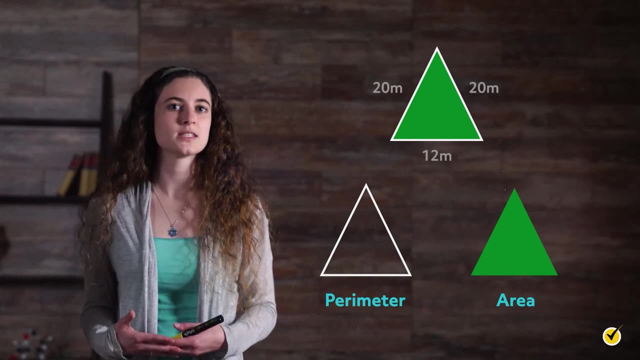 Okay, now that we know what perimeter and area are, let's figure out how to find the perimeter. We don't need any fancy formula or anything. All we need to do is add the length of the sides together. So if we know all the sides of our yard, we can easily find the perimeter. 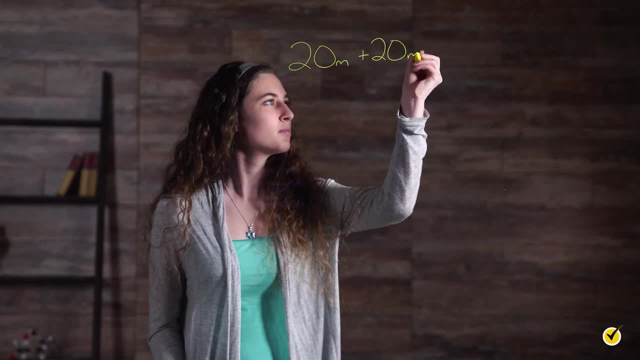 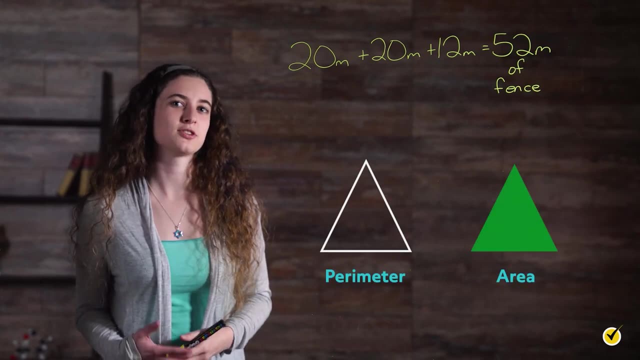 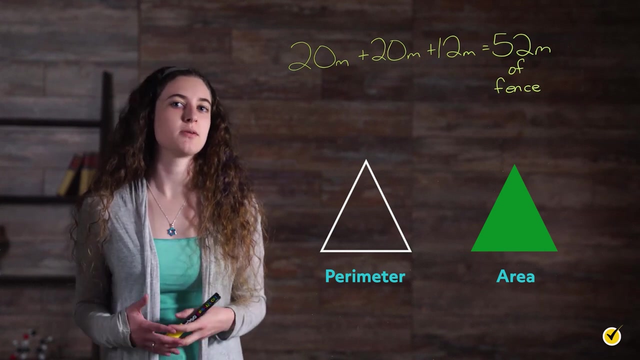 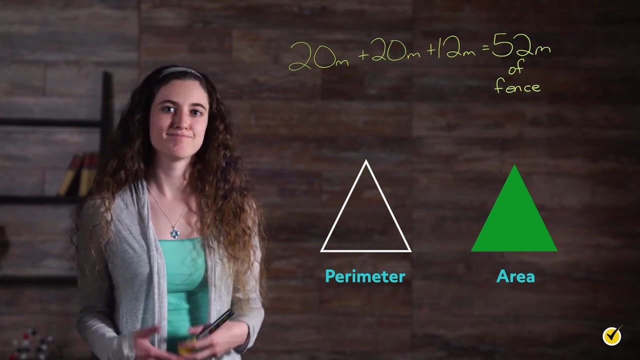 20 meters plus 20 meters plus 12 meters gives you 52 meters of fence. Not much to that one. Notice that the answer is given in meters. That's because perimeter is a distance. Walking around the yard would mean walking 52 meters. 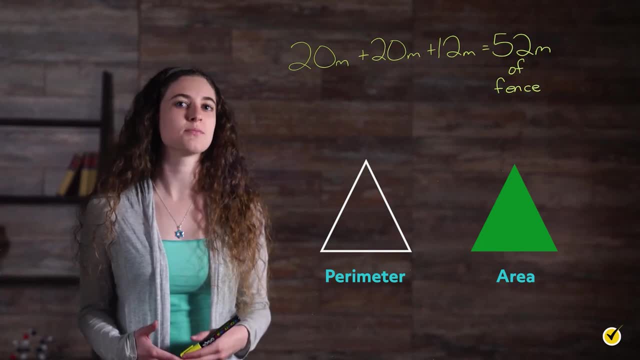 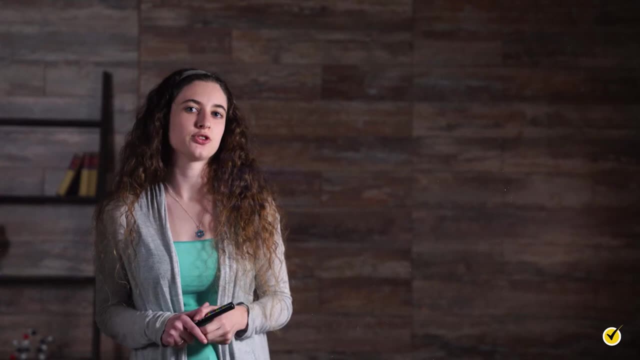 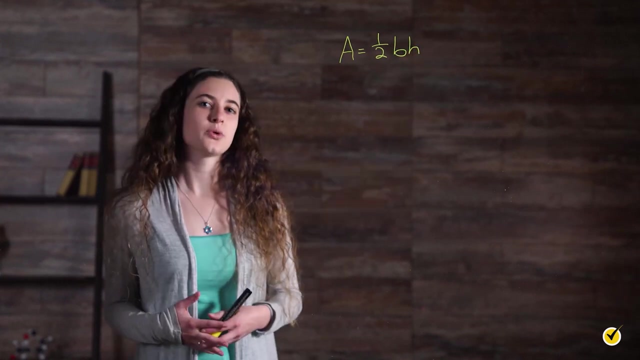 That's all there is to it. No matter what type of triangle you have, just add up the length of the sides and the perimeter. Now let's deal with area. There is an actual formula for finding the area of a triangle. The formula is: area equals one half base times height. 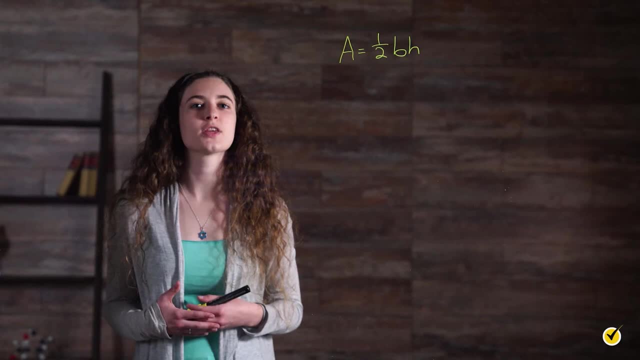 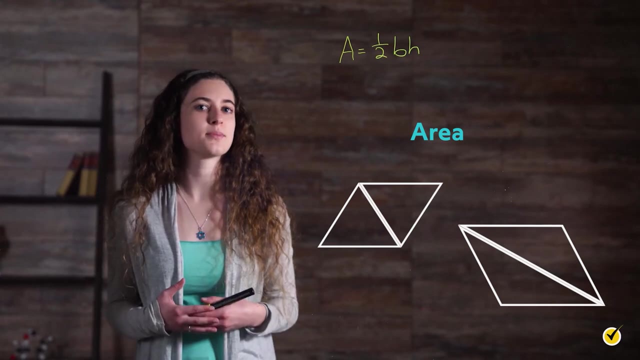 Let's quickly explain where that one half comes from. The formula for the area of a parallelogram is: area equals base times height. If we compare the two shapes, we can see that a parallelogram can be made by two equal sized triangles. 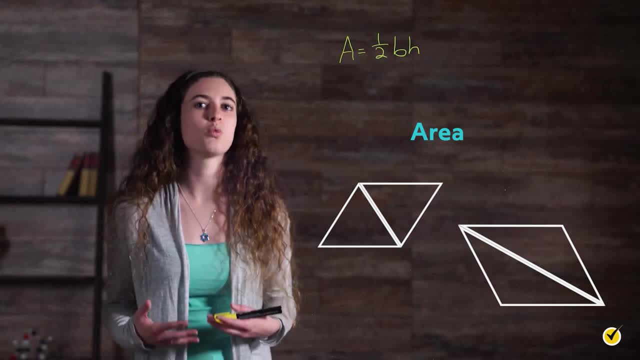 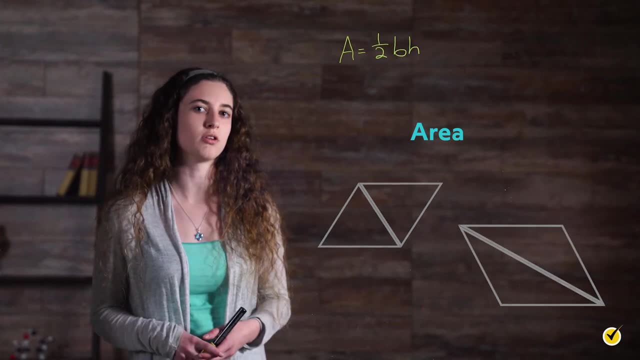 So we can say that a triangle is half a parallelogram, Which is where the one half comes from in the formula For triangles. the formula for area does work a bit differently depending on the type of triangle. Let's start with the right triangles. 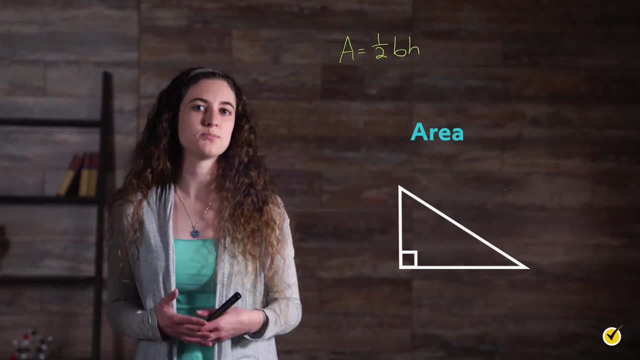 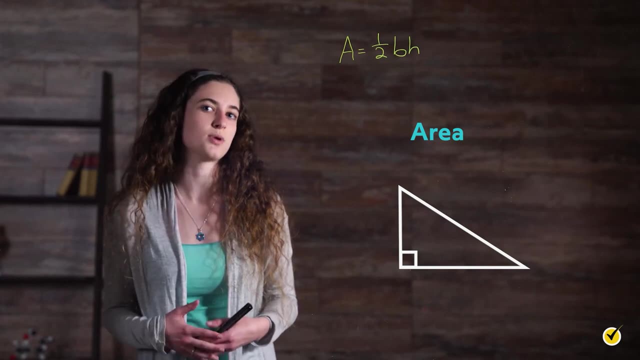 We have our formula, but the question we need to answer is which side is B and which side is H? For a right triangle like this one, B and H are the two sides adjacent or next to the right angle. It doesn't matter which is which. so let's say that B equals 6 centimeters and H equals. 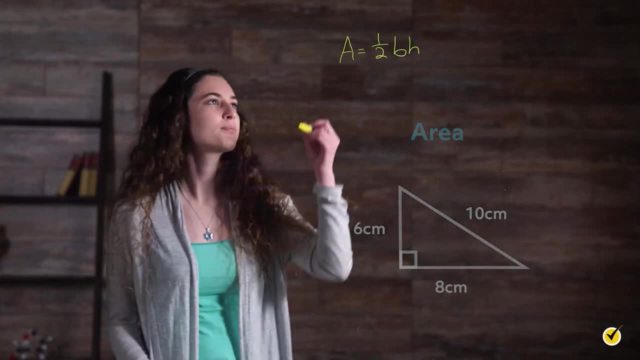 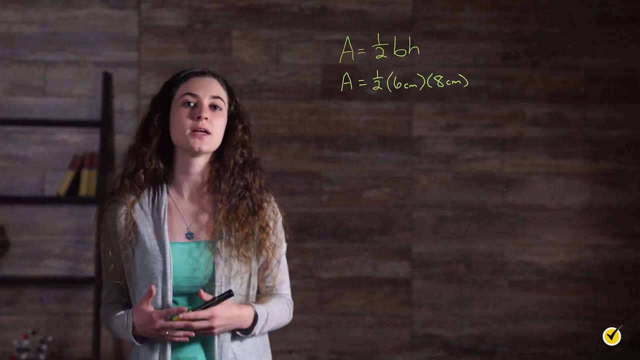 8 centimeters. Now we can plug in the right triangle And we can plug them into our formula. It's always a good idea to substitute with parentheses to help keep things organized. We've even left the units in so that we can see what will happen with them. 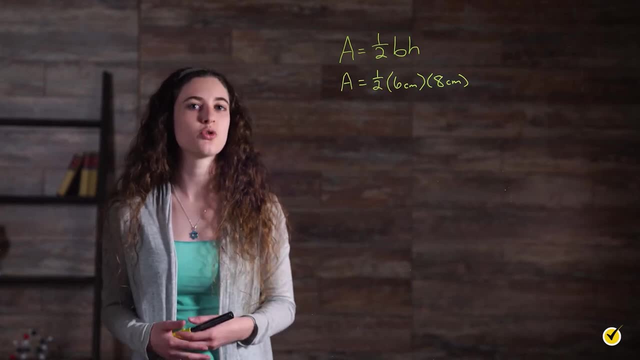 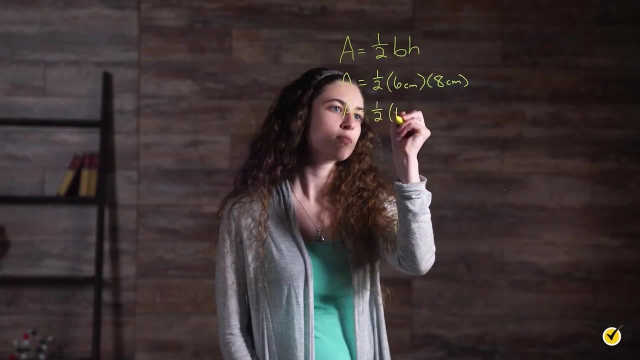 At this point, we only have multiplication left to do So, according to the commutative property of multiplication, we can rearrange before multiplying. Now let's solve this. Okay, We're done. We're done, Let's look at what's left. 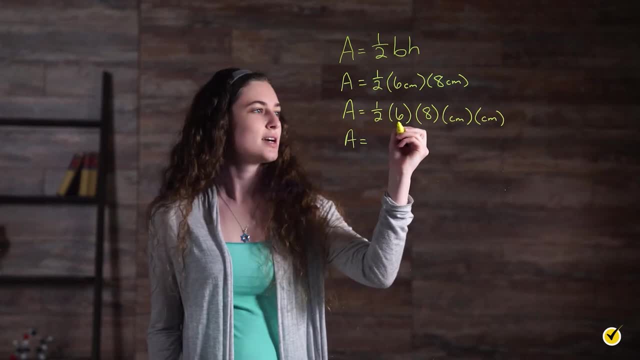 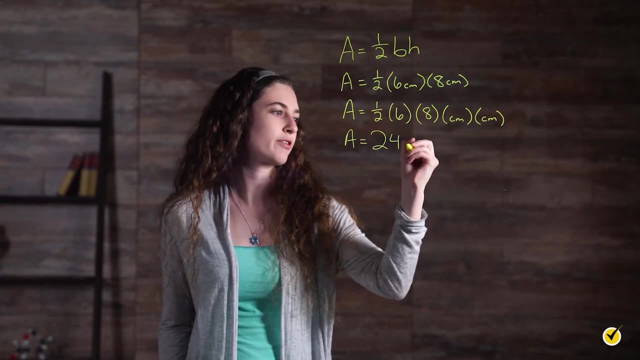 So we have our area Area equals 1 half times 6,, which is 3.. 3 times 8 gives you 24.. And centimeters times centimeters gives you centimeters squared. So we end up with our area as 24 centimeters squared. 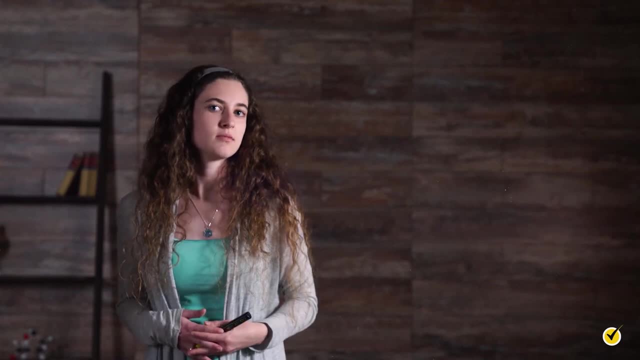 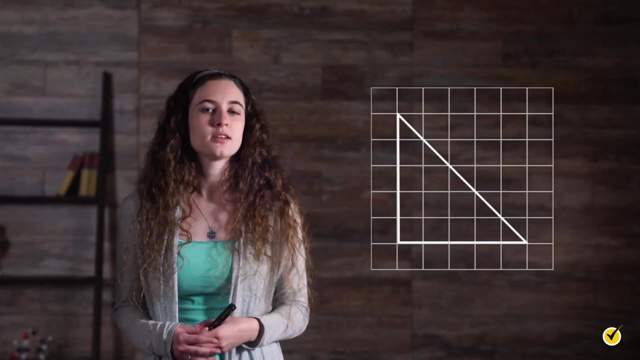 For area problems, the answer will always be in square units. That's because we're trying to determine how many square centimeters will fit in our triangle. We can see that clearly by looking at an isosceles right triangle that has legs measuring five units on some graph paper. 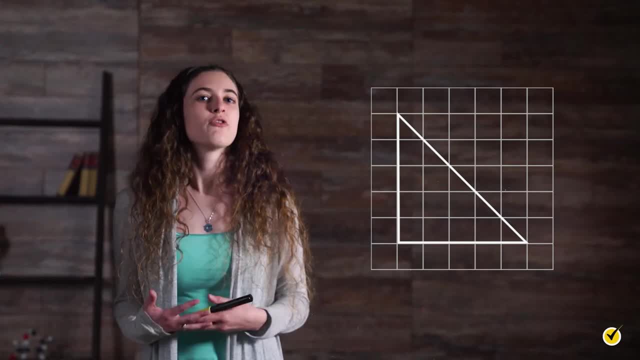 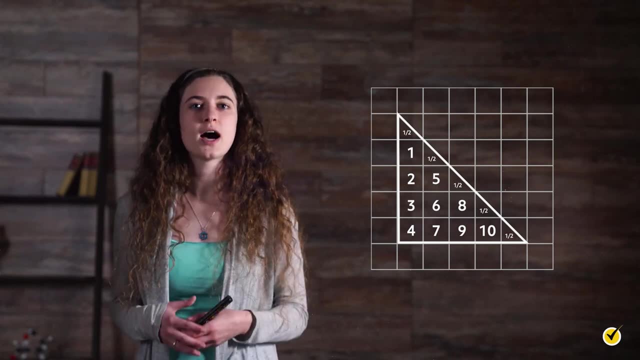 How many squares will be inside the triangle? We can count them First. we'll count the whole squares that fit inside, then we'll add the half squares. There are 10 full squares plus five half squares, for a total of 12.5 squares. 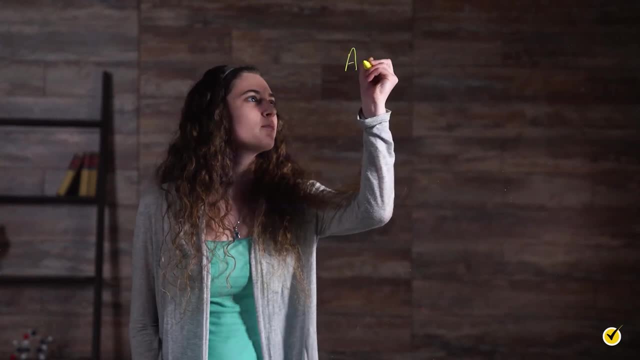 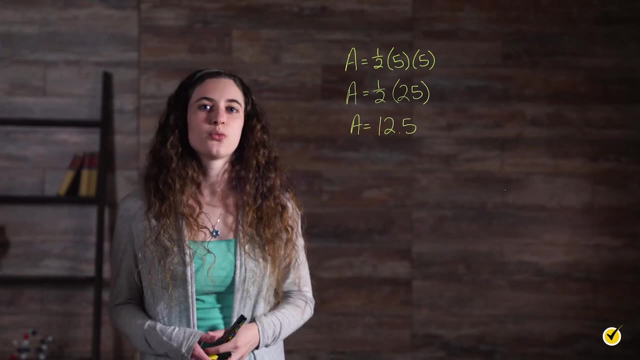 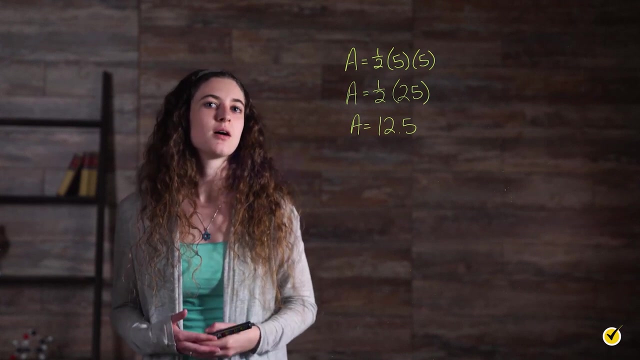 If we use our formula, we'll find the same thing. Now we've seen the formula work and gained a better understanding of why the units are squared. All we have left to do is find the area of acute and obtuse triangles. Let's start with an acute triangle. 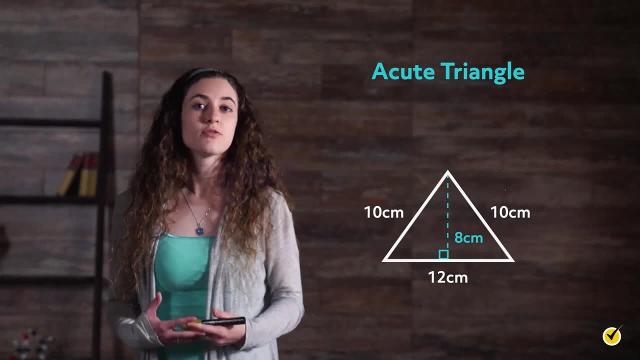 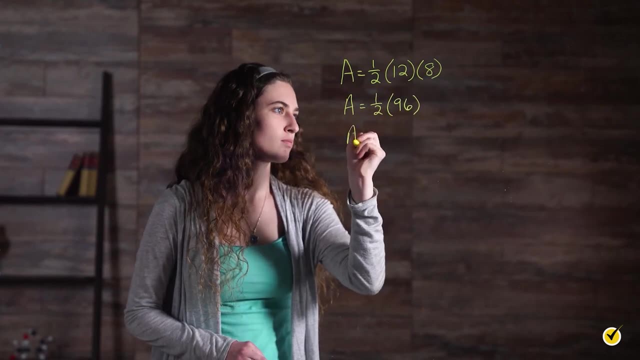 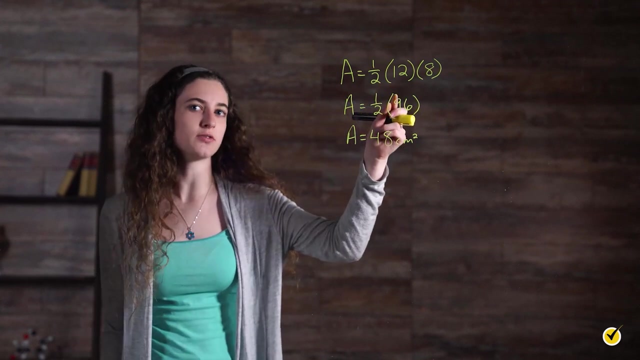 Note that the height is always perpendicular to the base. From here we can find the area Here we have. our area equals one half times the base, which in this case is 12 centimeters, times the height, which is eight centimeters. 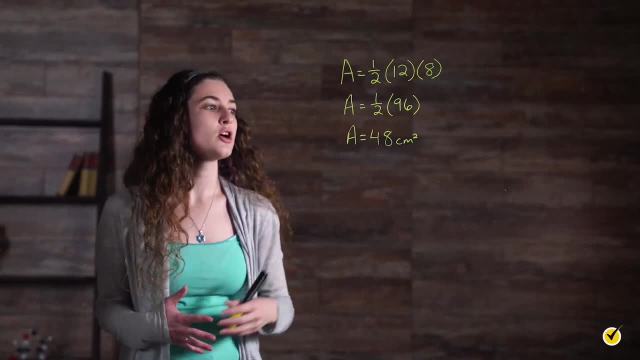 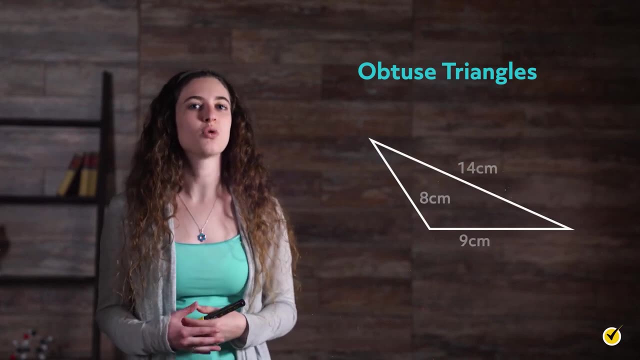 So we get one half times 96 from 12 times eight, which gives us 48 centimeters squared. The same thing applies to obtuse triangles, except the height or altitude will often appear outside of the triangle. like this, We can see that the height of the triangle is six centimeters. 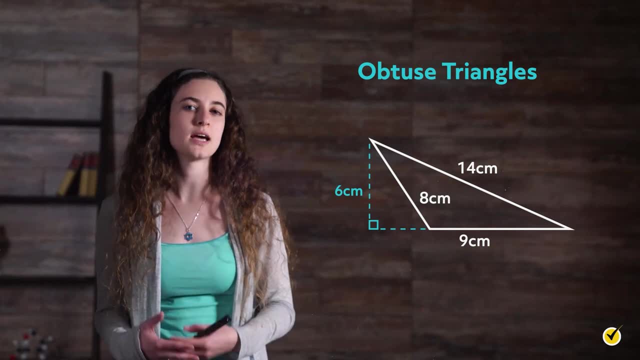 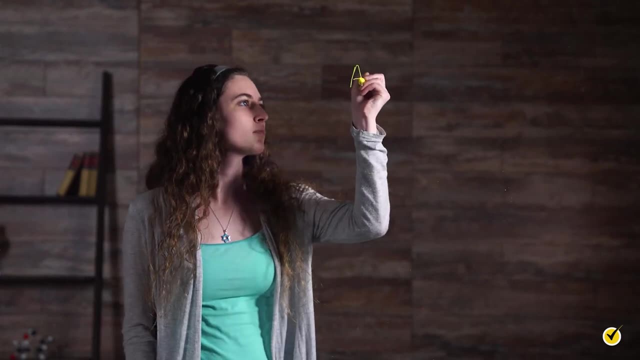 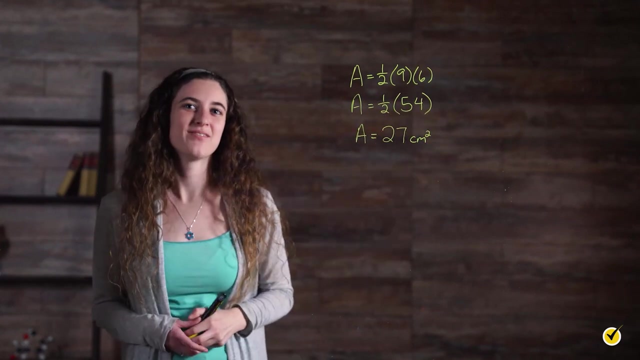 and the side it is perpendicular to is the base, which measures nine centimeters. We don't need the other two numbers at all, so let's plug in the base and the height. That's all there is to it. Here's one more for you to solve on your own. 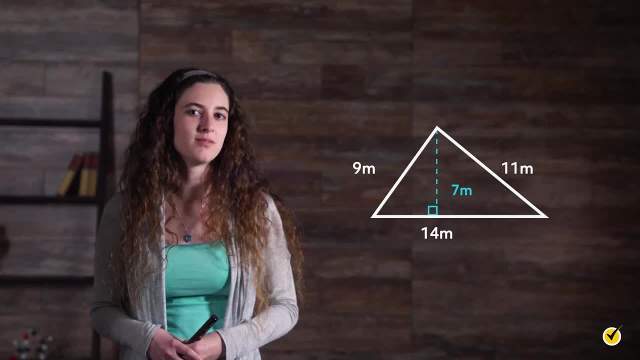 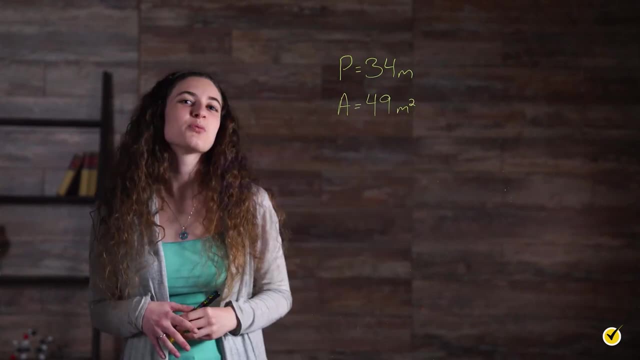 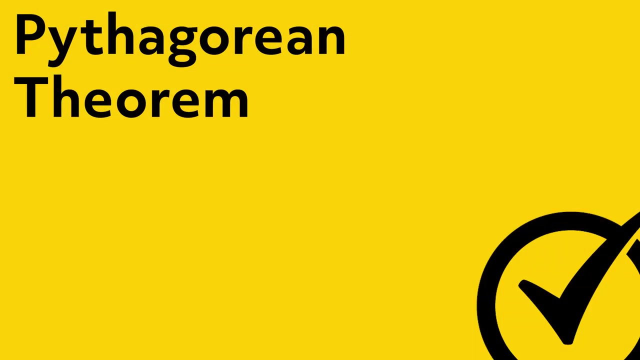 Try pausing this video and then finding the perimeter and area of this triangle. Think you got it. The perimeter is 34 meters and the area is 49 meters squared. Hi and welcome to this review of the Pythagorean theorem. We're going to go over how to use it properly. 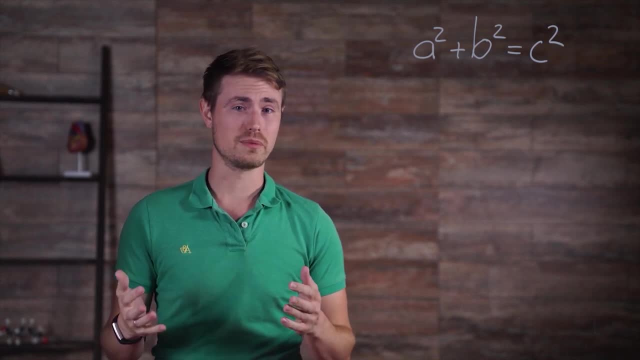 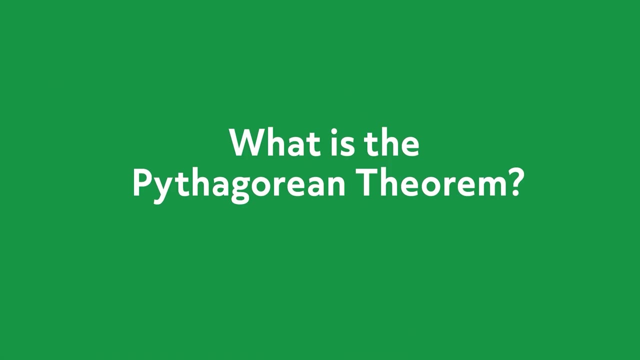 and also go over some special triangles called Pythagorean triples. that could save you some time when taking tests. So let's get started. First things first. what is the Pythagorean theorem? The Pythagorean theorem is a squared plus b squared. 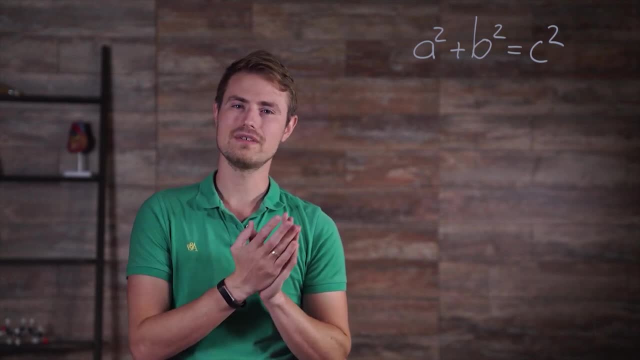 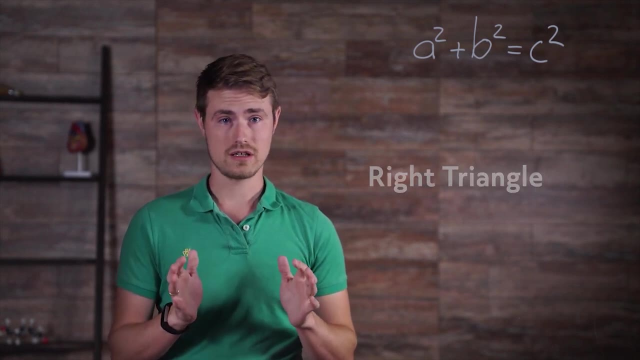 is equal to c squared. Now this is used to find the length of a side of a right triangle. when we know the length of the other two sides, The triangle has to be a right triangle, which means that it has an angle that measures. 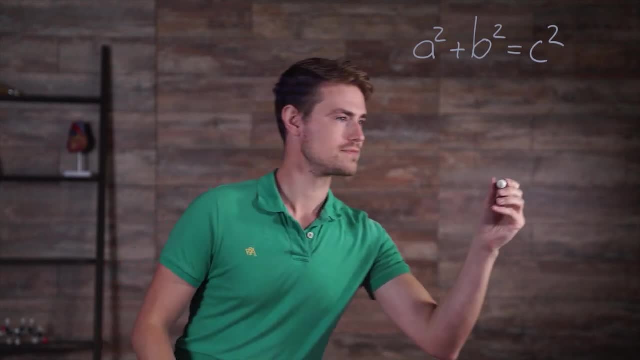 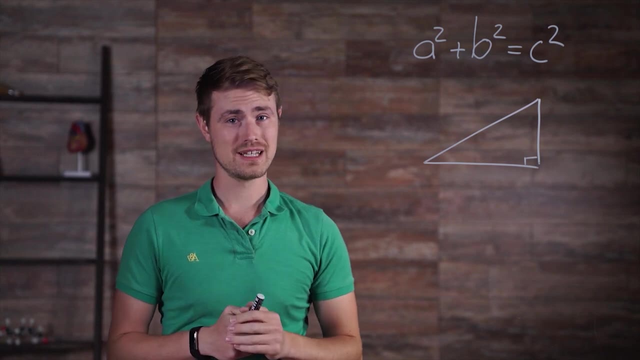 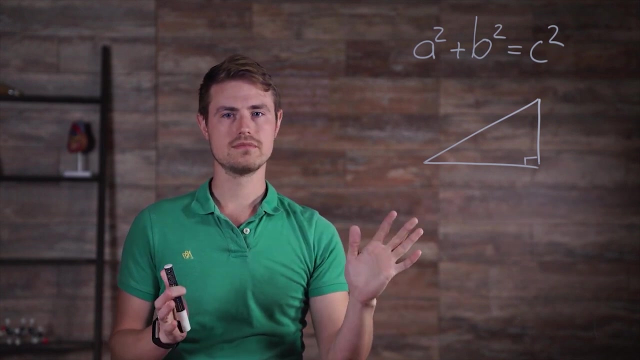 exactly 90 degrees like this one. The theorem is very easy to remember and just as easy to use. In the theorem, a, b and c are the lengths of the three sides of the triangle. But which is which? Let's start by figuring out where to find a, b and c. 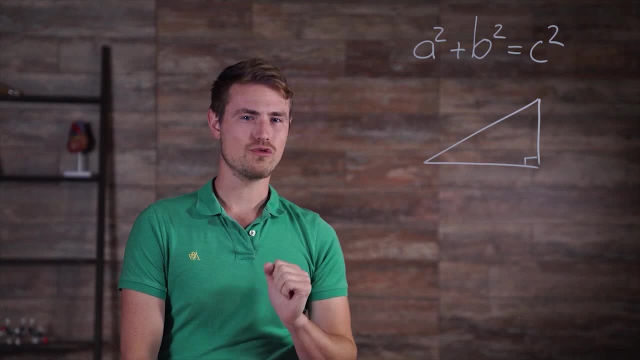 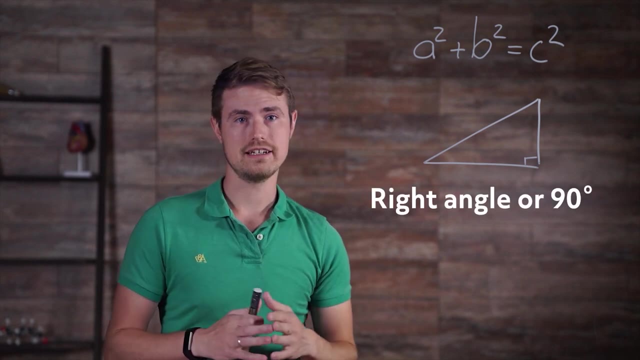 in a triangle. To start, you can tell that you're dealing with a right triangle because you see this little square in one of the angles. That's the symbol for a right angle, or 90 degree angle And any triangle that has a right angle. 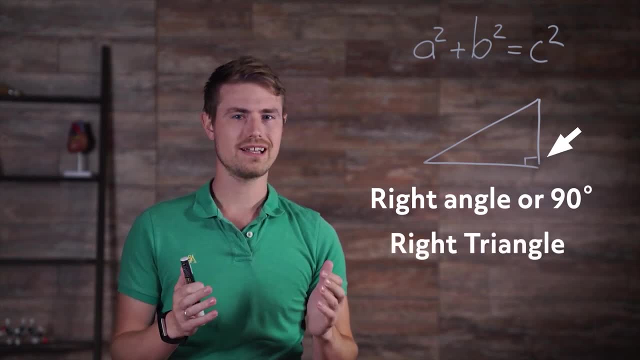 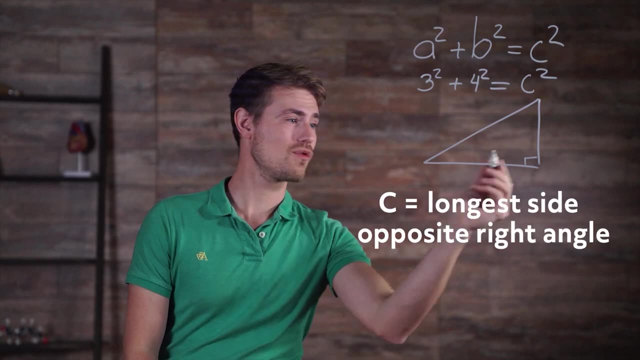 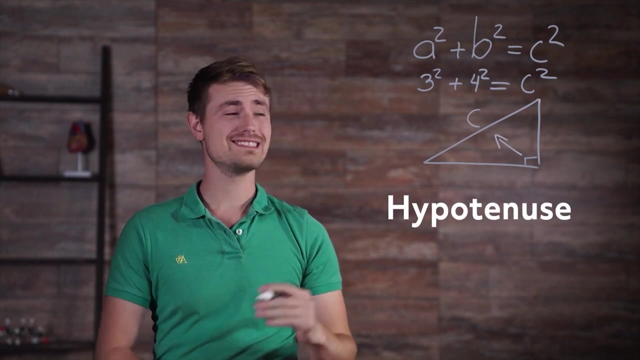 must be a right triangle. So now we have to decide where to put the three side lengths. The key is to start with c, which is always on the side across from the right angle. This is called the hypotenuse, and it's always the longest. 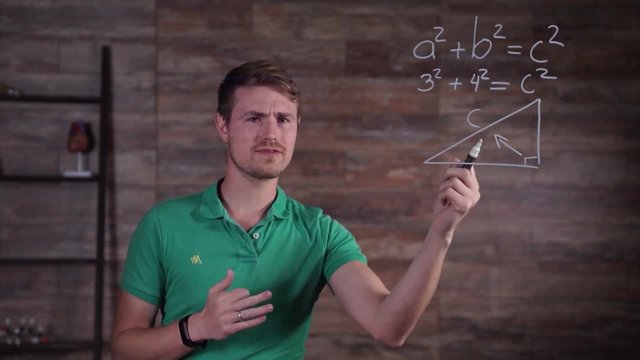 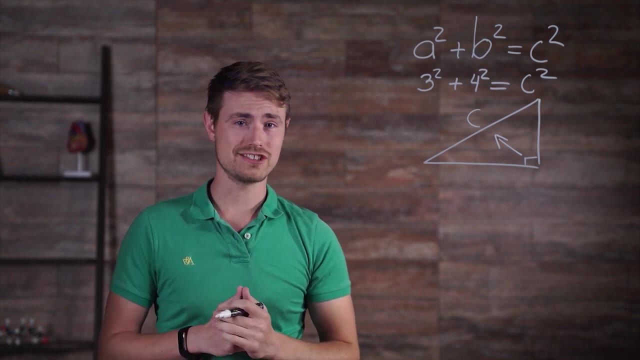 side. You may be asking yourself: If c is always across from the right angle, how do I tell which of the other two is a and which is b? It's a good question and the answer is: it doesn't matter Either of these two sides, which are called legs. 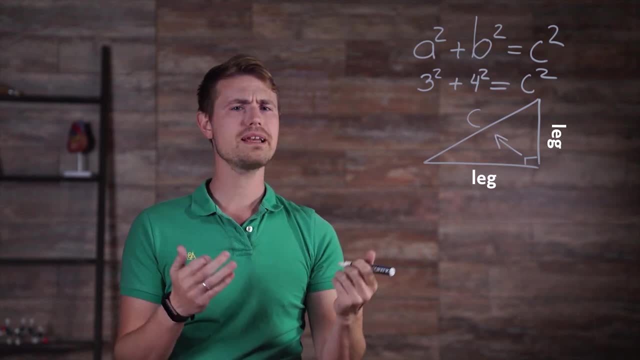 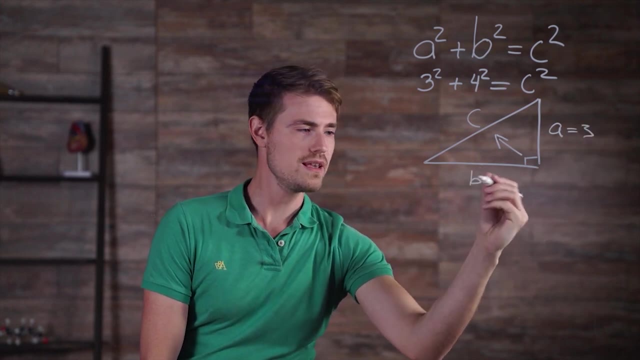 can be used as a and then just use the other one for b. Let's pick 3 centimeters for a and our b will be down here and we know that's 4 centimeters. So this is what our theorem looks like. 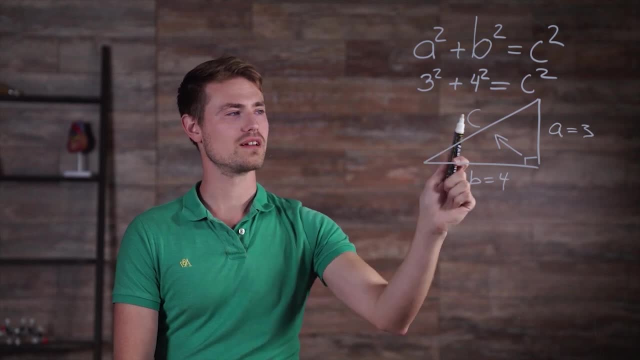 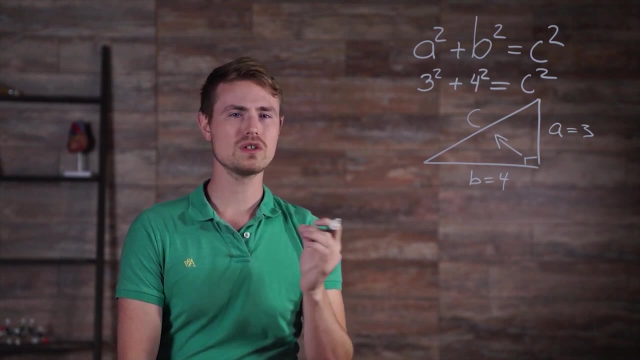 When we have it filled in, 3 squared plus 4 squared is equal to c squared. Now we can just evaluate 3 squared and 4 squared, which means multiplying 3 times 3 and 4 times 4 to get the following: 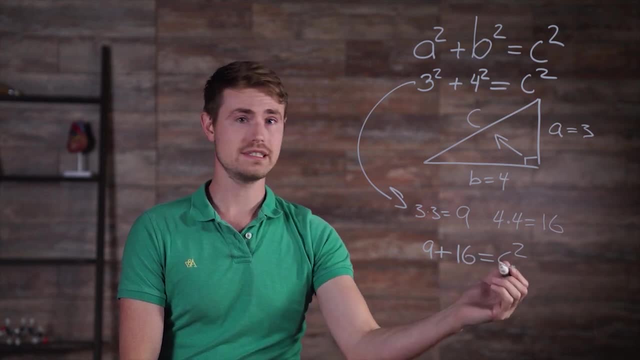 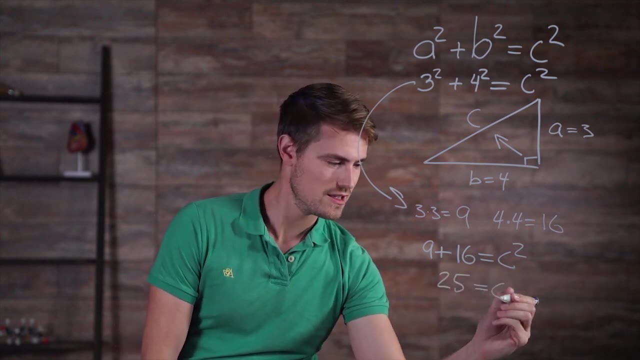 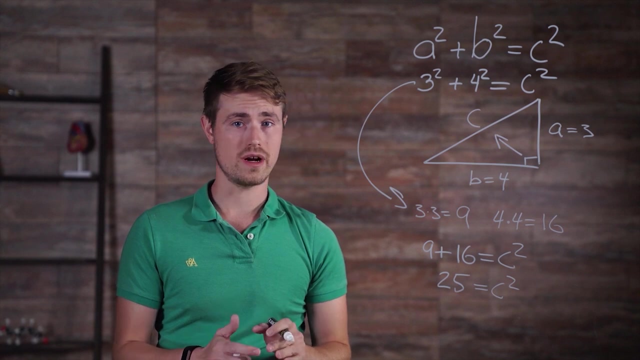 So now we have: 9 plus 16 is equal to c squared. So what's that? A little addition tells us 25 is equal to c squared. Now here's where it gets a little tricky. We know that c squared is equal to 25,. 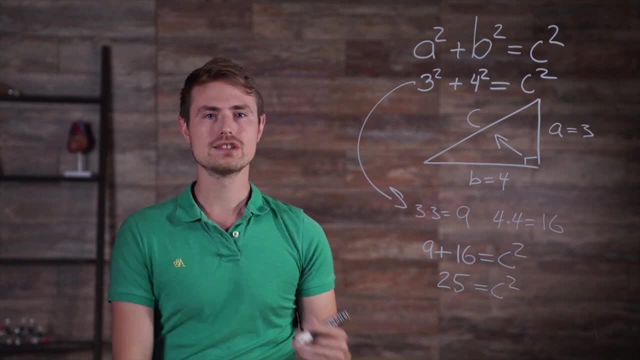 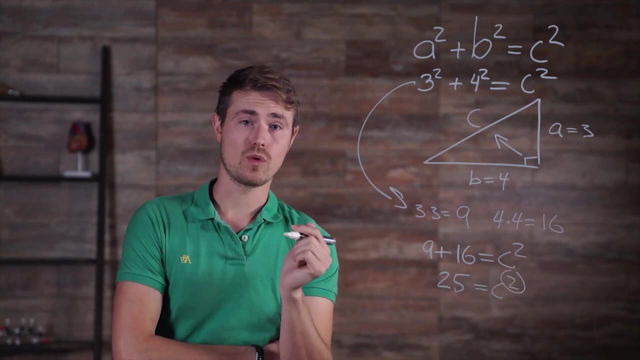 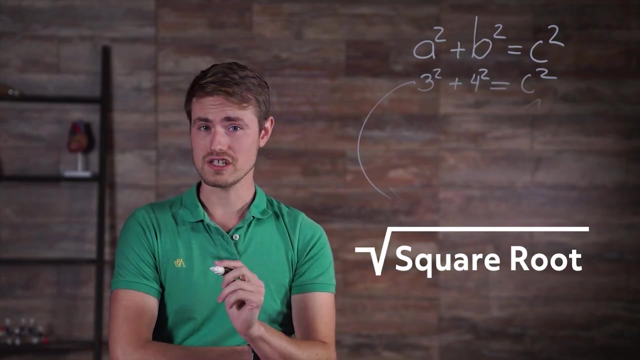 but we want to know what c is, not what c squared is. So how can we get rid of that little 2?? Well, we use the inverse or opposite operation of squaring something, and that inverse operation is the square root. Since it's an equation, whatever we 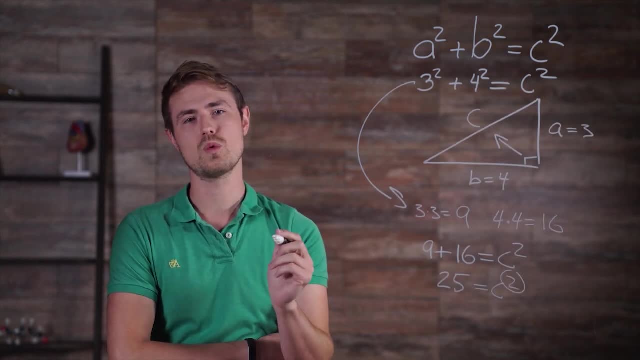 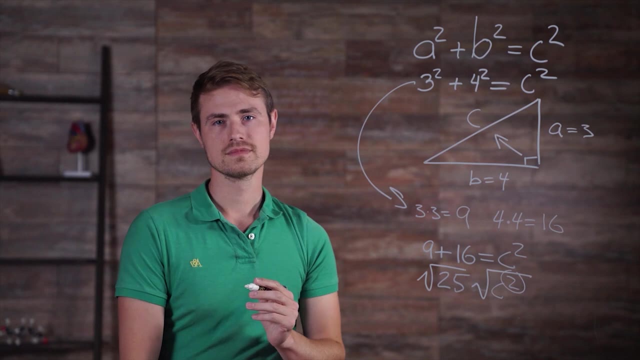 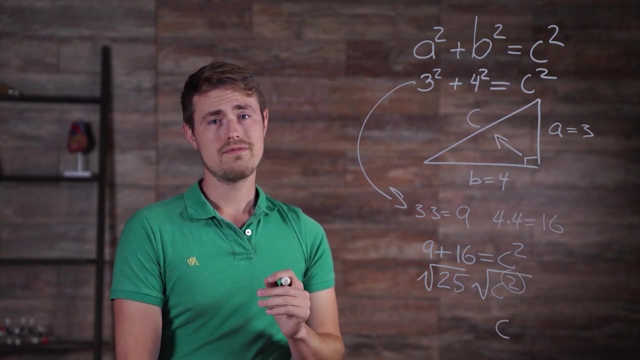 do to one side of the equation, we must do to the other. So I'm going to take the square root of both sides. The square root of c, squared is c, And the square root of 25 just happens to be 5.. 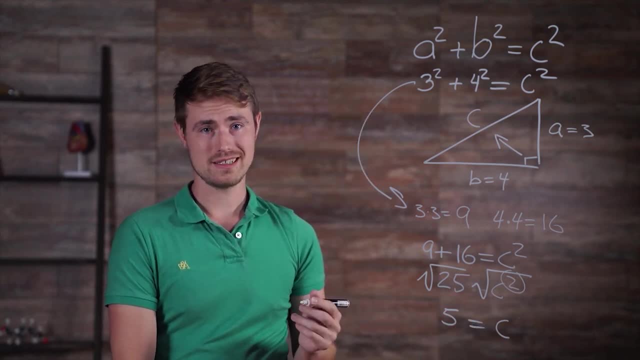 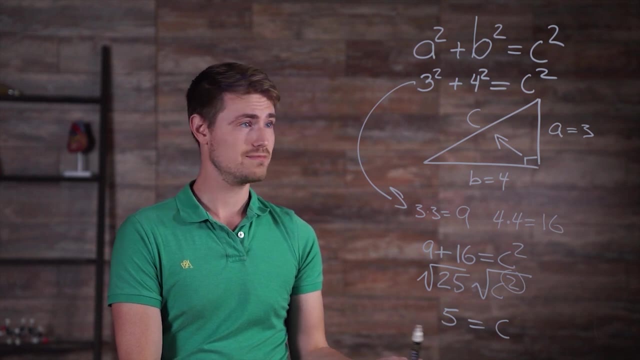 Look at that. It's always good to check our answer to see if it makes sense. Since we're finding c, it should be 5. longer than any of the other two sides, and 5 is greater than both 3 and 4. Also. 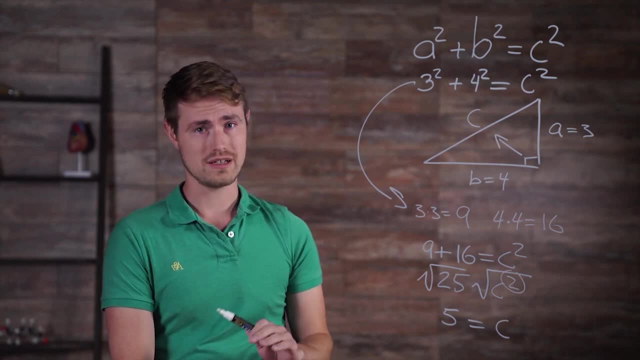 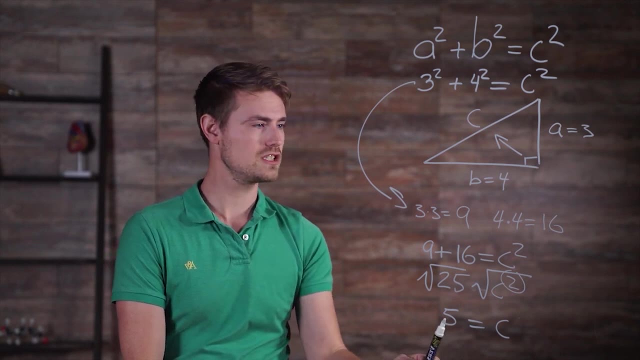 because of the triangle inequality theorem, which is something we'll get to in a later video, the hypotenuse must be less than the sum of the other two sides, which means 5 has to be smaller than 3 plus 4, which it is, So you might have. 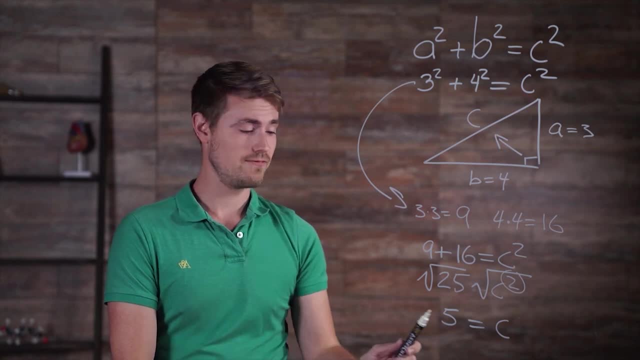 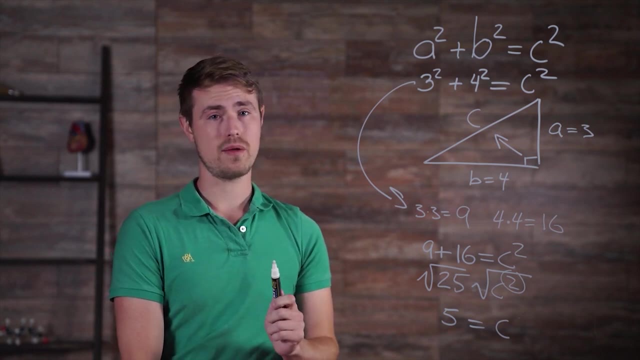 noticed that the answer to this problem was a nice neat integer 5.. This is actually kind of rare if we look at random triangles, but it's not rare in a math problem. you might see on a test It happens whenever a problem uses a. 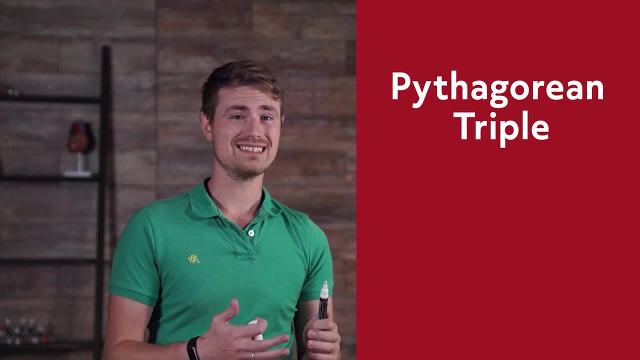 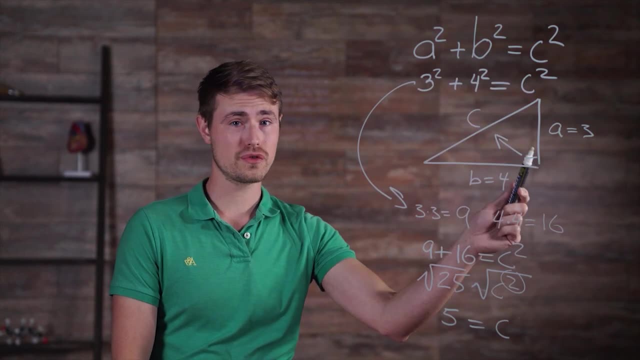 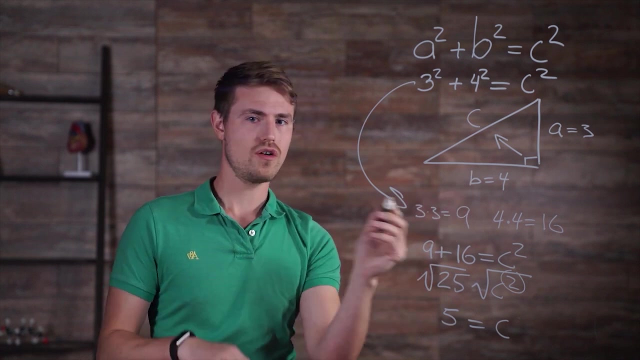 Pythagorean triple. The triangle we just looked at is the most common kind of a 3,, 4, 5 right triangle. The legs measure 3 and 4 and the hypotenuse is 5.. Sometimes it will be disguised by multiplying all the numbers by 2, which means we would 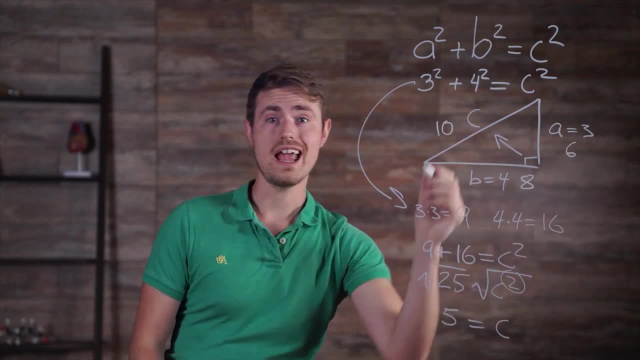 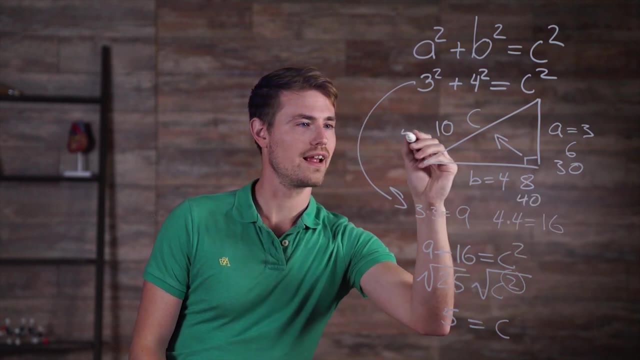 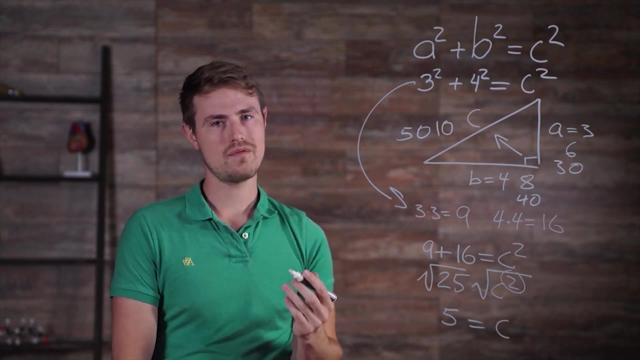 get a 6,, 8, and 10, or multiplied by 10,, which means we would have a 30,, 40, and 50 lengths, or maybe any other number. You don't need to know this to solve a. 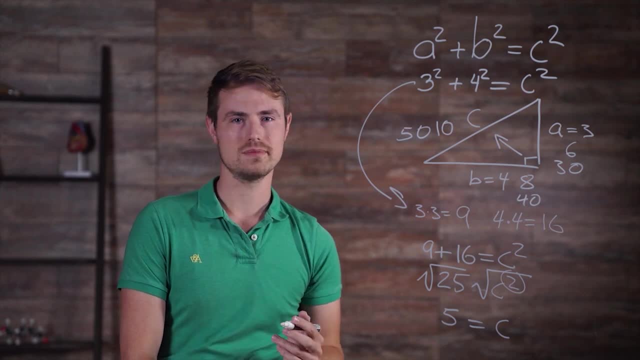 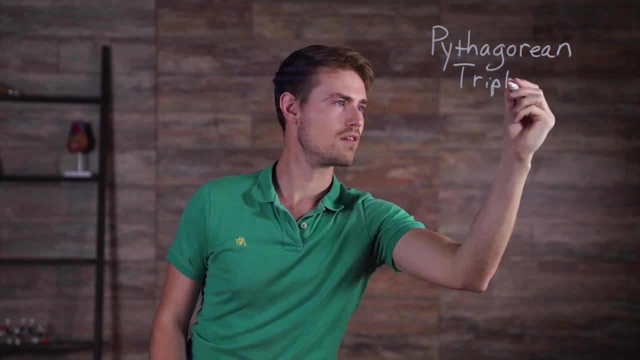 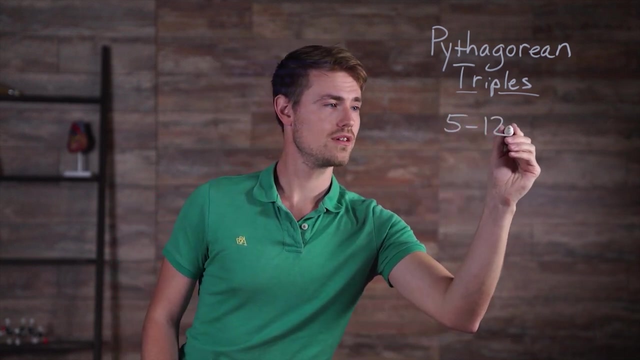 Pythagorean theorem problem, but it's a nice shortcut to save you some time or allow you to check your answer another way. Other Pythagorean triples include 5,, 12,, 13,, 8,15, and 17,, and 7,, 24, and 25.. 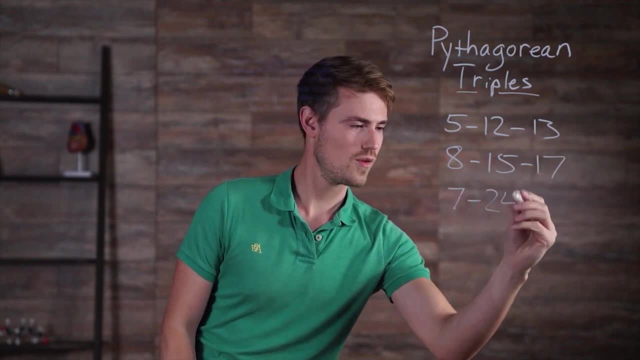 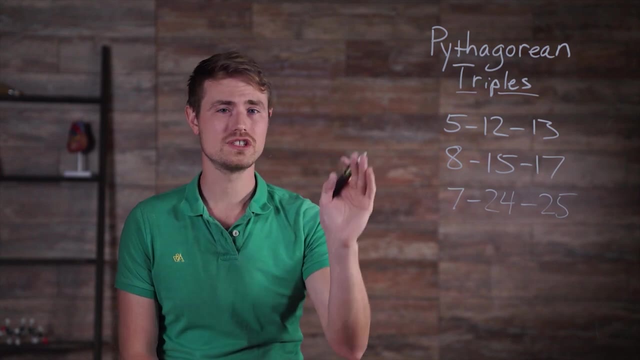 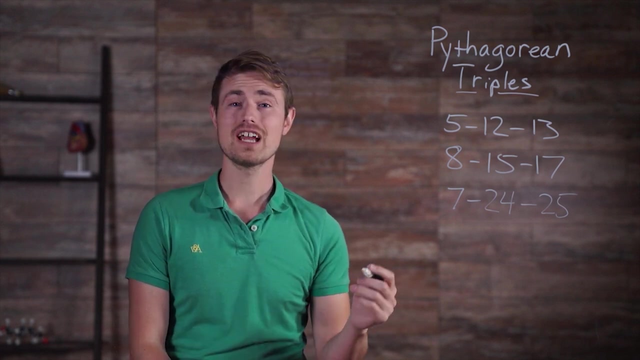 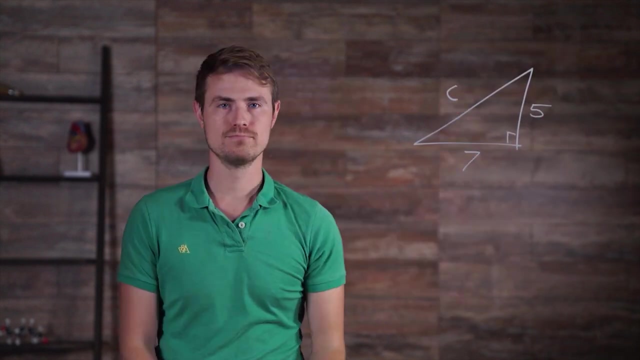 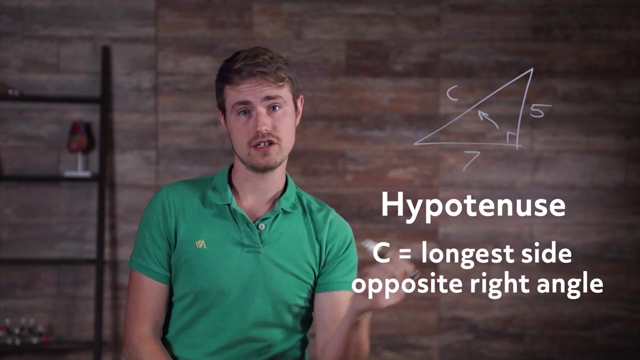 There are many more, but these ones are the ones you will see most often. Of course, there are right triangles that aren't Pythagorean triples. Let's look at one just so you can see what the answer will look like. Once again, we're solving for the hypotenuse the longest side, which is opposite the 90 degree or right angle. 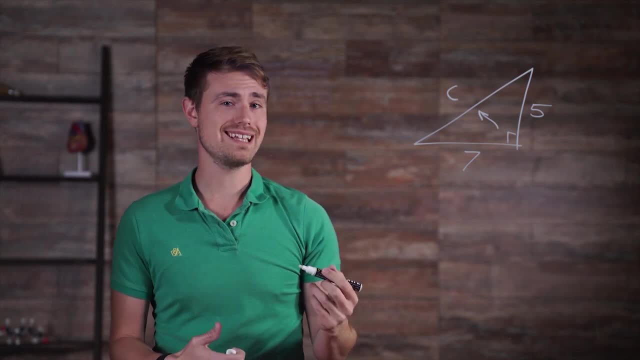 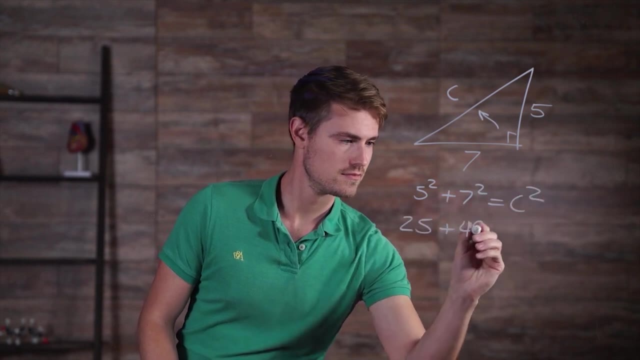 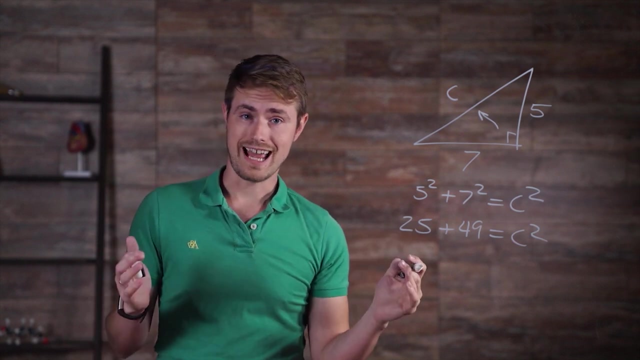 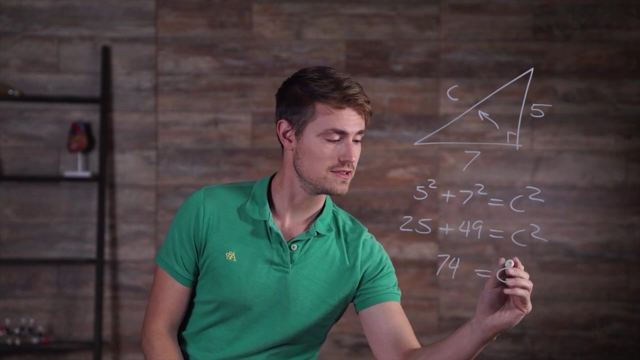 This is length C. When we plug in 5 and 7 for A and B, we get this. We get 25 plus 49 is equal to C squared. So let's add 25 and 49 to get 74, which is equal to C squared. 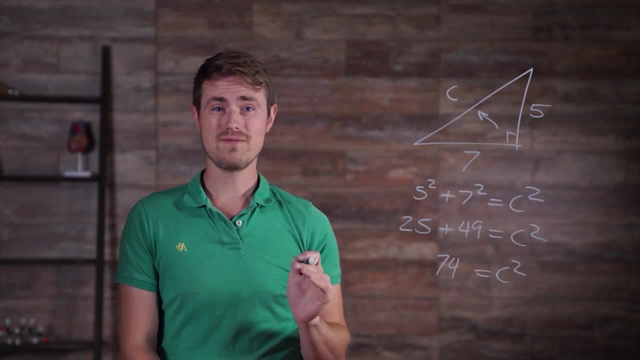 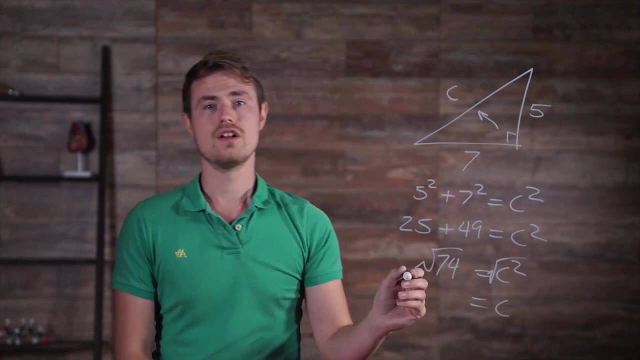 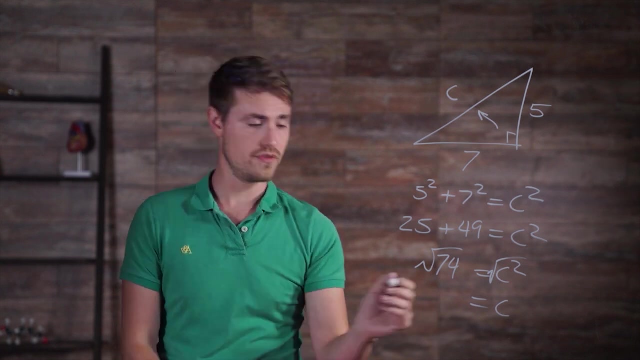 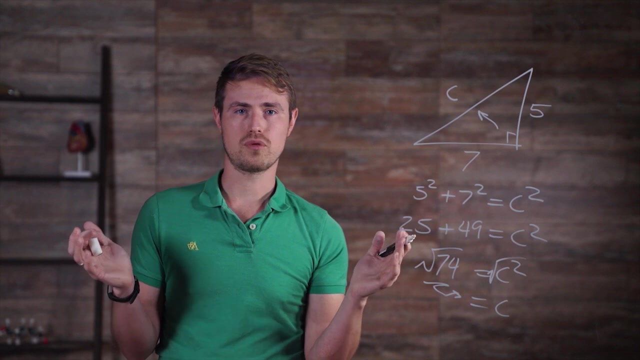 Then we take the square root of each side and find out that the square root of 74 is equal to C. Now, even though 74 isn't a perfect square, this is the answer. If you take the square root on a calculator, you only get an approximation of the answer. 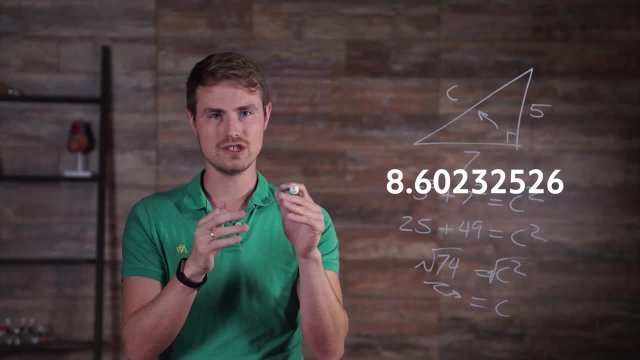 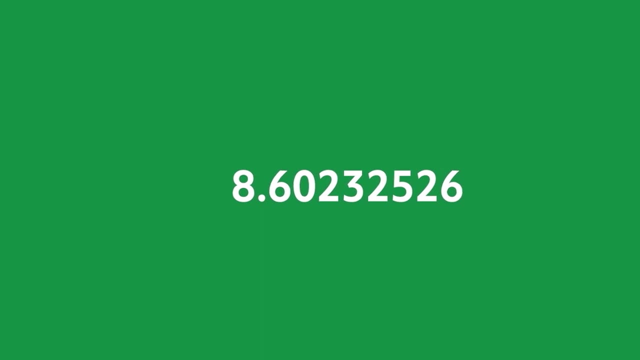 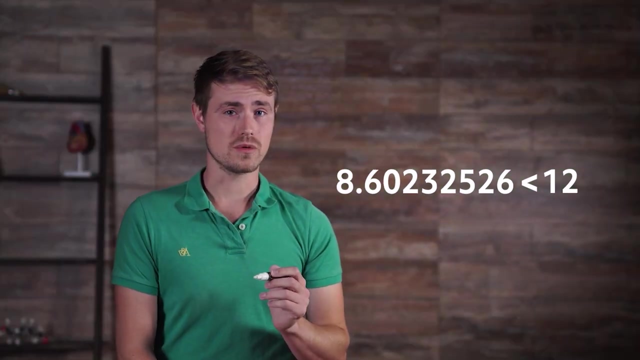 which is about 8.60232526. forever. We can do this approximation to do our checks. It's greater than either of the other two sides and it's less than the two sides added together, But when writing the answer we should use the square root form. 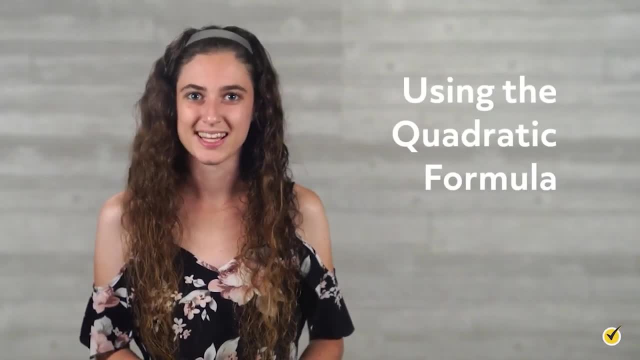 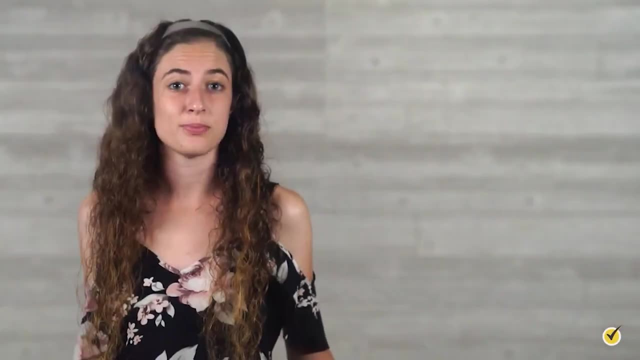 Hello and welcome to this video about using the quadratic formula. Today we'll learn what the quadratic formula is, when you use it and how it's applied to find roots in quadratic equations. Let's start by talking about quadratic equations. A quadratic equation in standard form is written as: 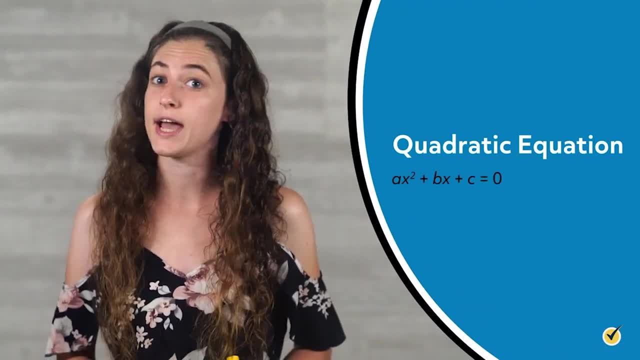 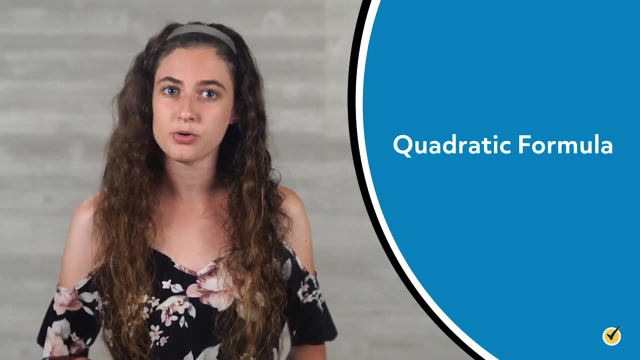 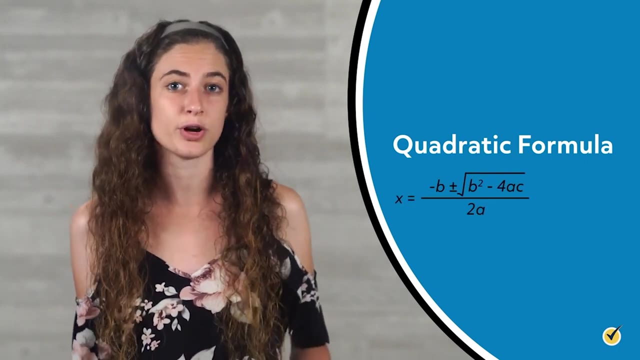 ax squared plus bx plus c equals zero. where a doesn't equal zero and a, b and c are all real numbers. The quadratic formula is an algebraic equation that helps solve any quadratic equation. The formula is: x is equal to negative, b plus or minus the square root of b squared minus 4ac. 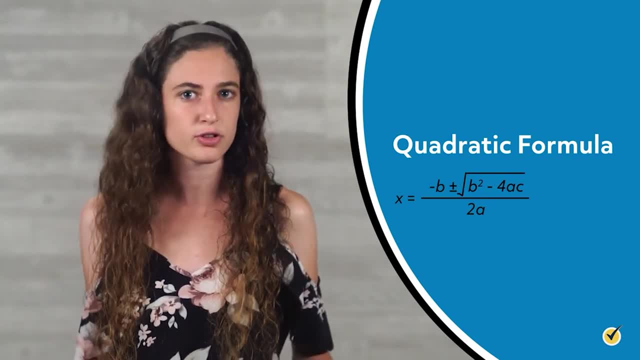 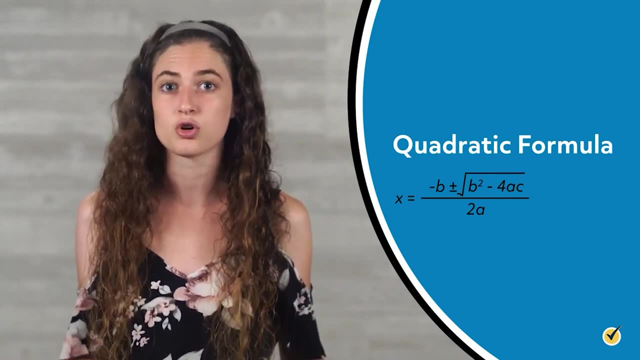 all over 2a. By substituting in given values for the variables a, b and c, you can solve for x using the quadratic formula. Solving for x gives us solutions for the quadratic equation. These solutions are also called roots. 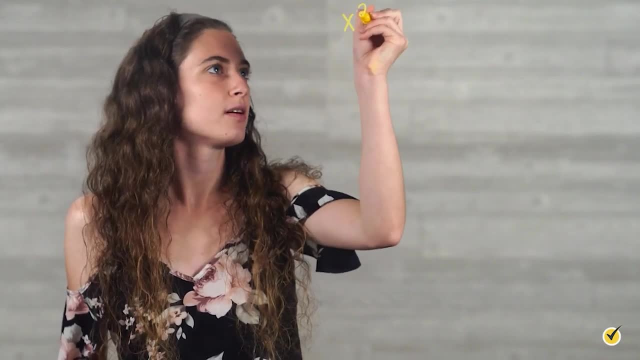 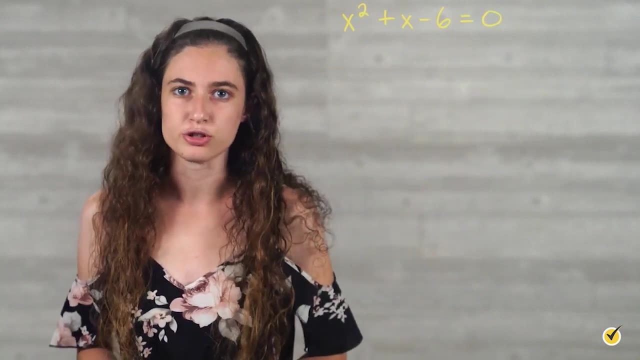 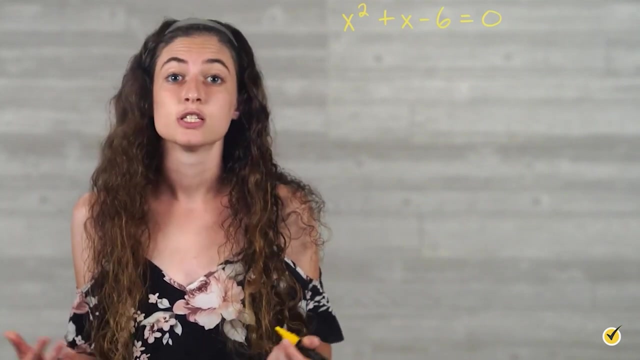 Let's consider the quadratic equation x squared plus x minus 6, equals 0, and use the quadratic formula to find solutions for x. First, identify the values for the variables a, b and c in the quadratic equation, Since the first term, x squared, is the same as 1x squared. 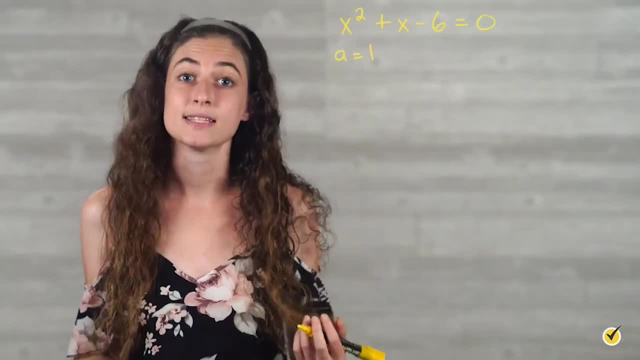 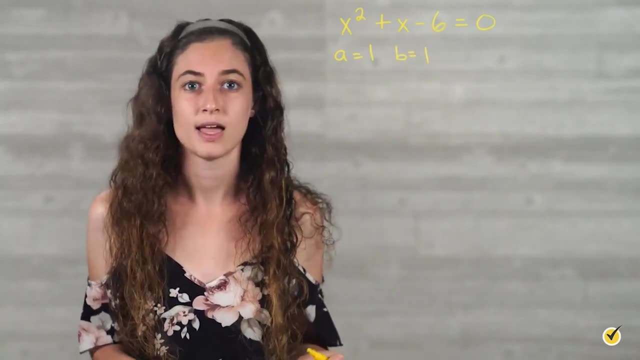 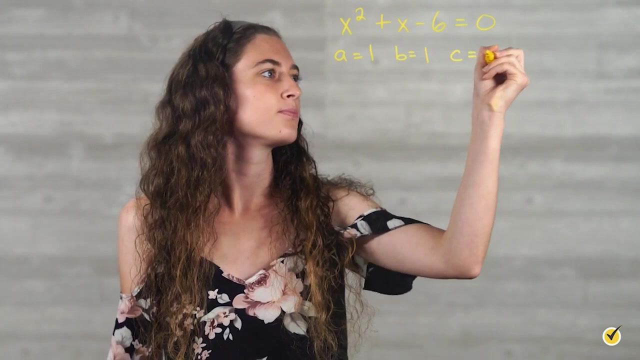 the value for a is equal to 1.. In the second term, x, the value for B is also equal to the coefficient of 1 and since the last term is negative 6 or minus 6, the value for C is equal to negative 6. next substitute: 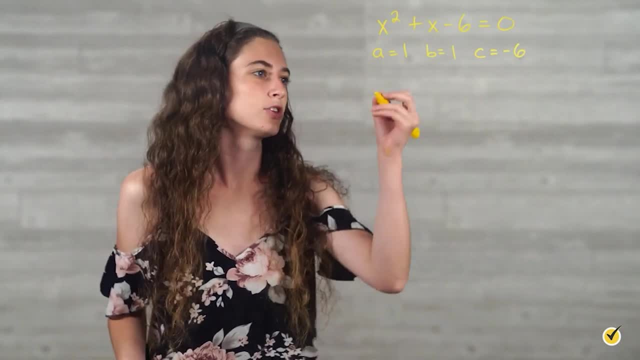 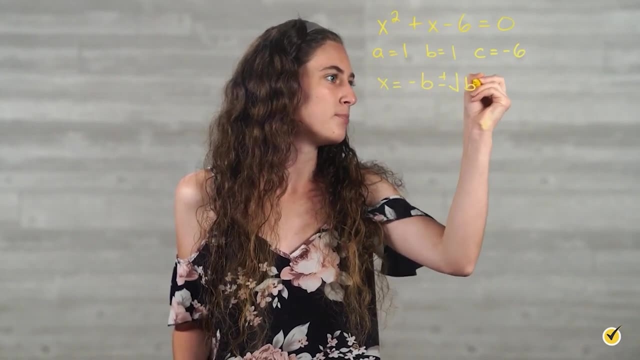 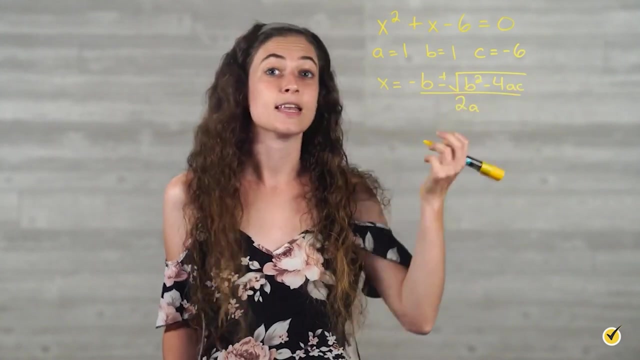 the values for a, B and C into the quadratic formula. so let's write out our quadratic formula again so that we remember it: X is equal to negative, B plus or minus the square root of B squared minus 4ac, all over 2a. and now. 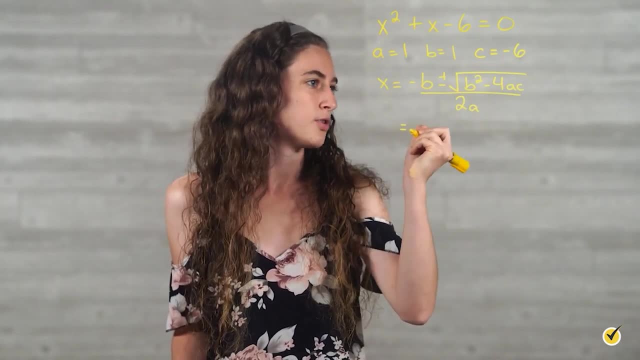 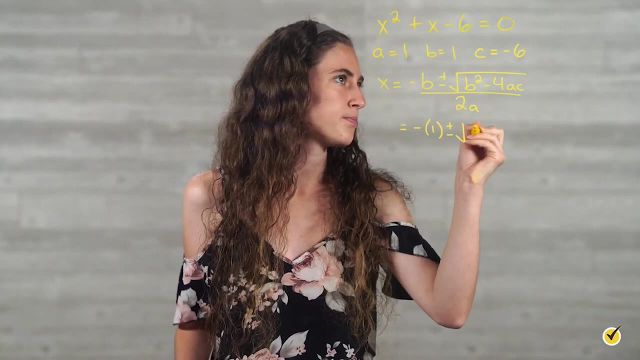 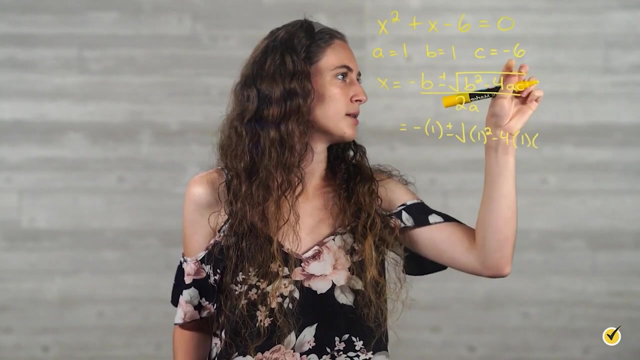 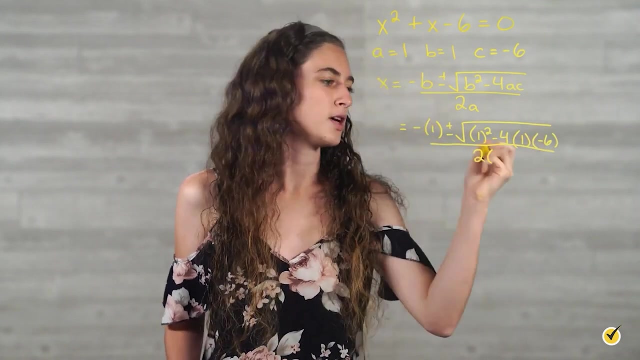 we're going to plug in our a, B and C into this equation. so X is equal to negative 1 plus or minus the square root of 1 squared minus 4 times 1 times negative 6, all over 2 times 1. from here, solve for X using the quadratic formula. so all we 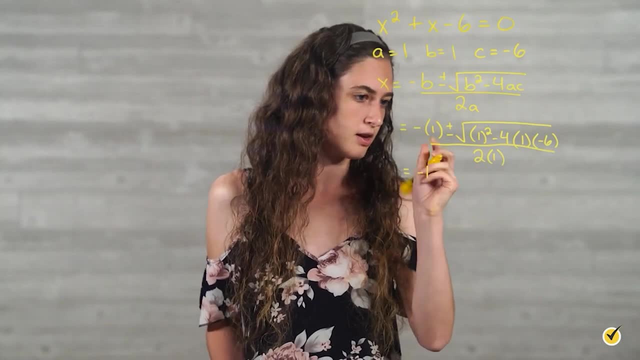 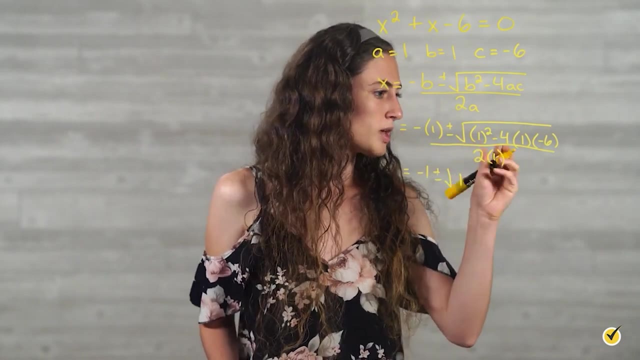 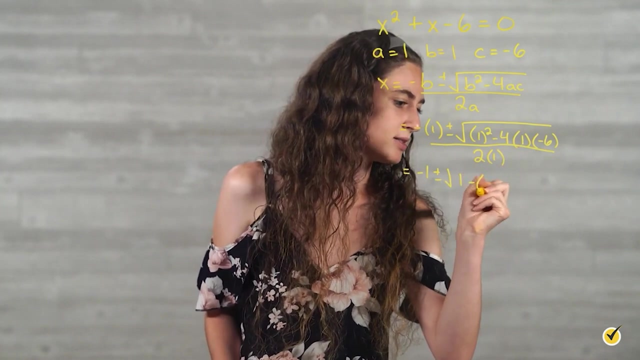 have to do is simplify, so we're going to leave the negative 1 right here for now and move on to this part. so we have the square root of 1. squared is 1 minus 4 times 1 times negative. 6 is negative 24. so minus negative 24. 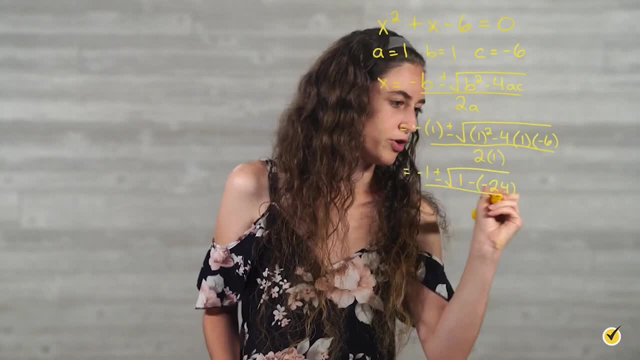 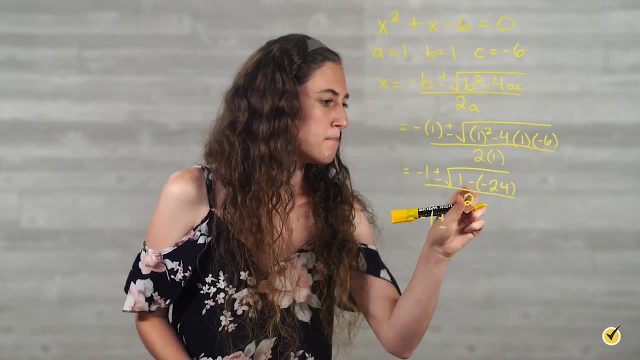 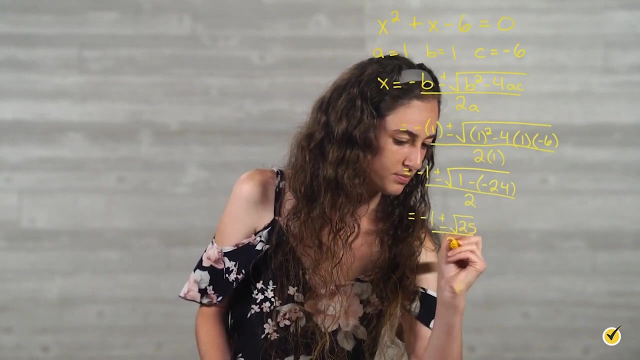 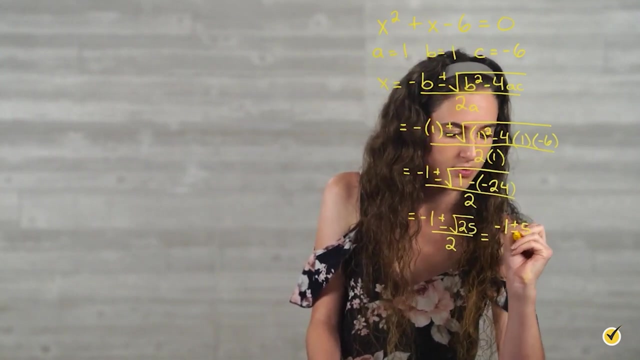 you over 2 times 1 is 2. 1 minus negative 24 is the same as saying 1 plus 24, which is 25. the square root of 25 is 5. so we have negative 1 plus or minus 5 over 2. and now 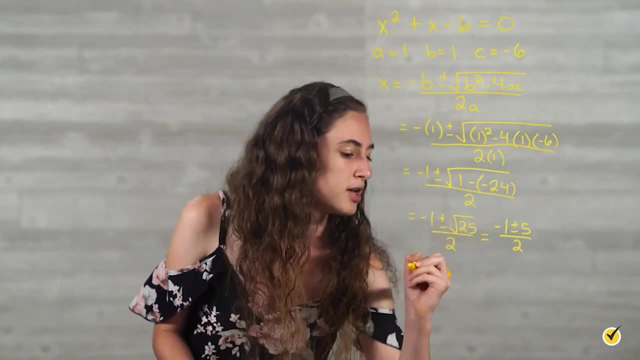 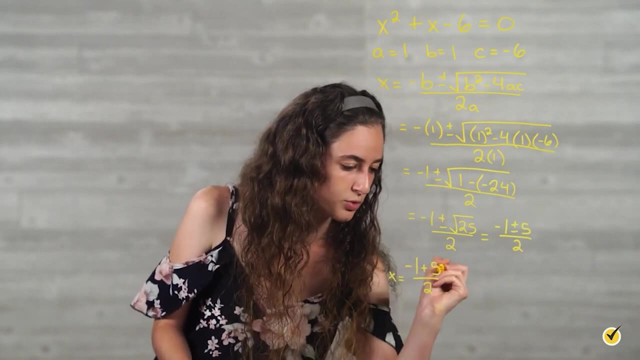 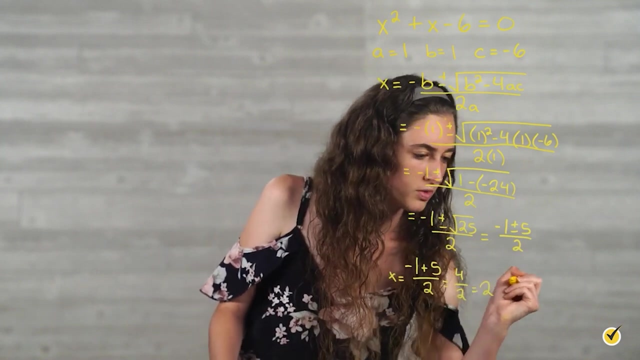 we're going to break this part into two different equations. so we're going to have negative 1 plus 5 over 2. remember X is equal to this. so this is one of our values for X. so negative 1 plus 5 is 4 over 2 is 2, and then for our other value: 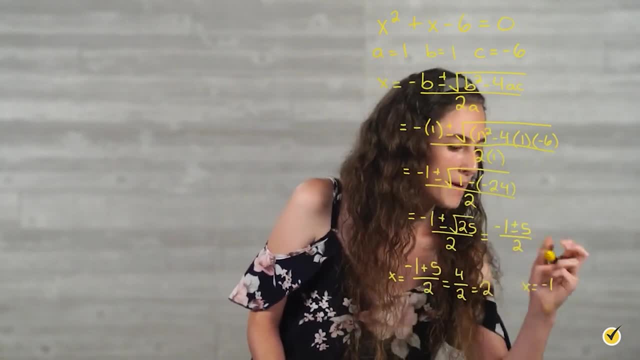 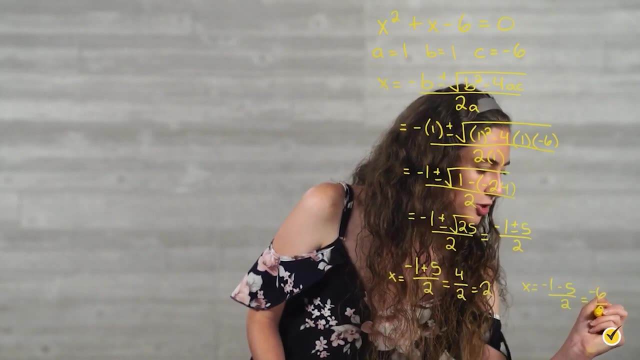 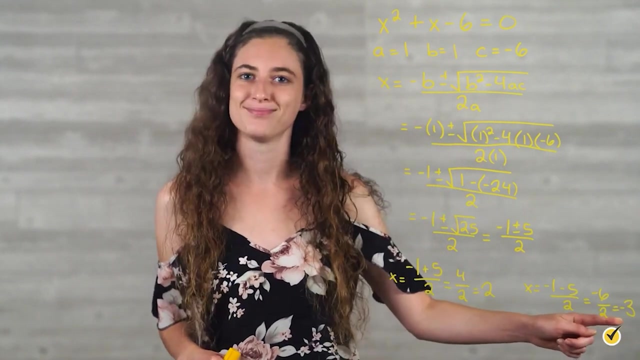 of X we're going to do. X is equal to negative. 1 minus 5 over 2. negative 1 minus 5 is negative. 6 over 2 is negative 3. so the roots for this quadratic equation are 2 and negative 3 in the 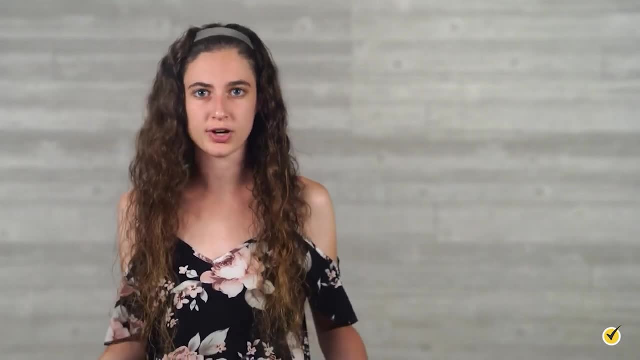 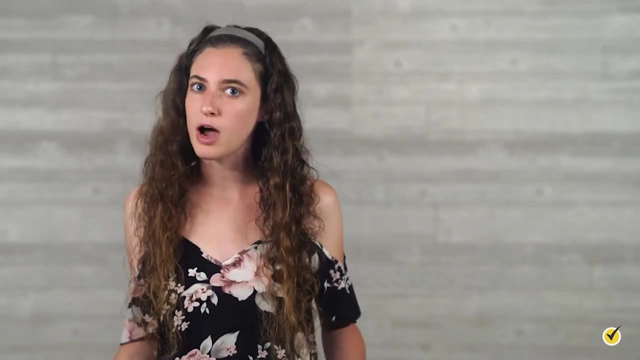 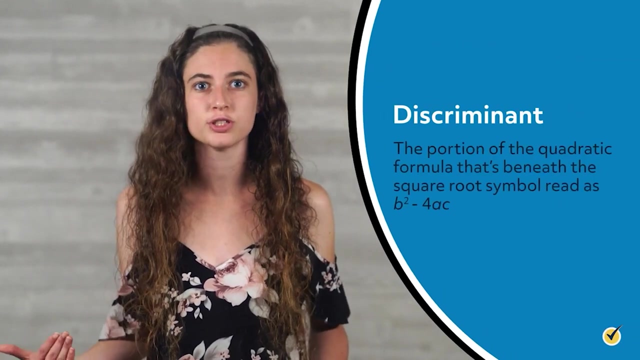 example we just looked at, there were two possible solutions or roots for X. quadratic functions can have two solutions: one solution or no real solutions for X. to figure out how many solutions a quadratic equation has, look at the discriminant in the quadratic formula. the discriminant is the portion. 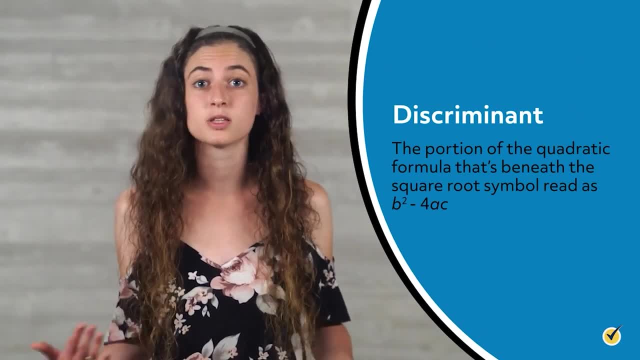 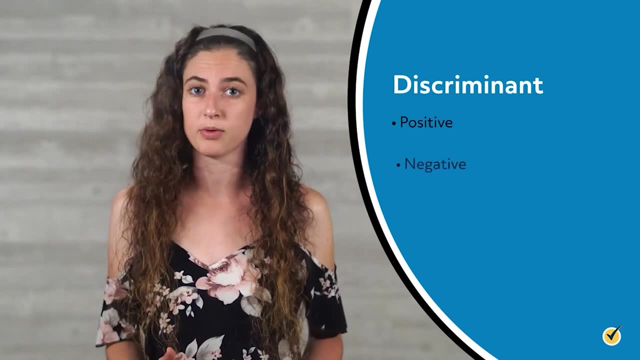 of the quadratic formula that's beneath the square root symbol. it's the part that's read as b squared minus 4ac. When simplified, the discriminant can be a positive number, a negative number or zero, And its sign tells us how many solutions the quadratic equation has. 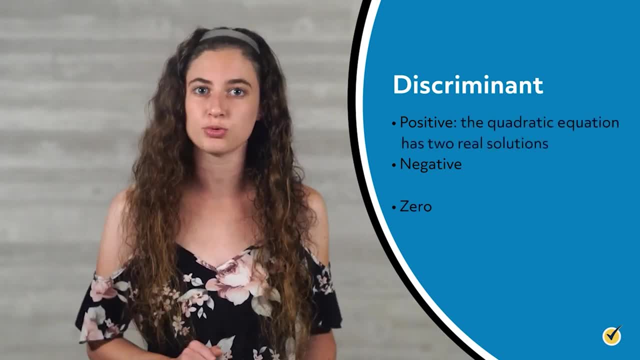 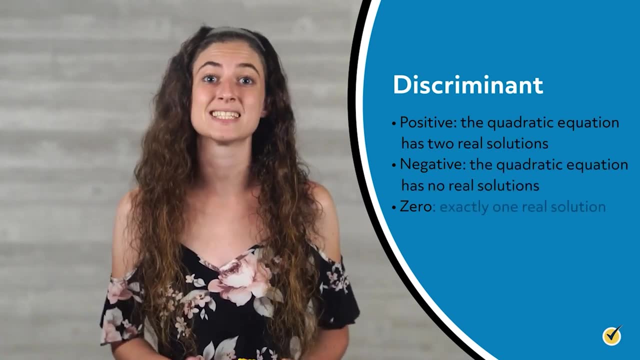 When the discriminant is positive, then the quadratic equation has two real solutions. When it's negative, then it has no real solutions. And when the discriminant is zero, then the quadratic equation has exactly one real solution. In the previous example, the discriminant was 25.. 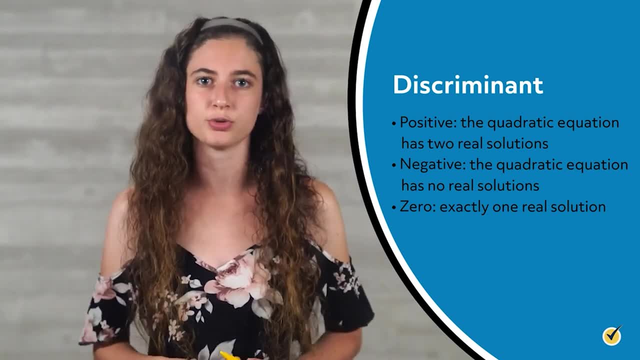 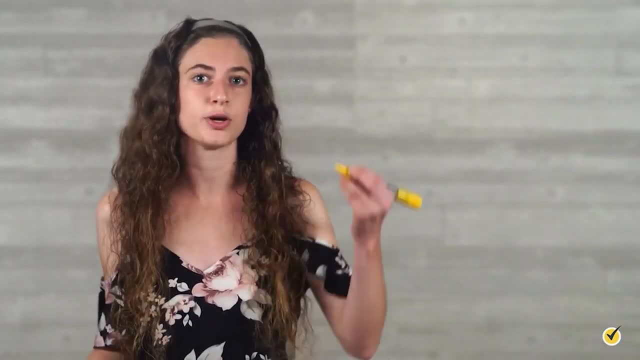 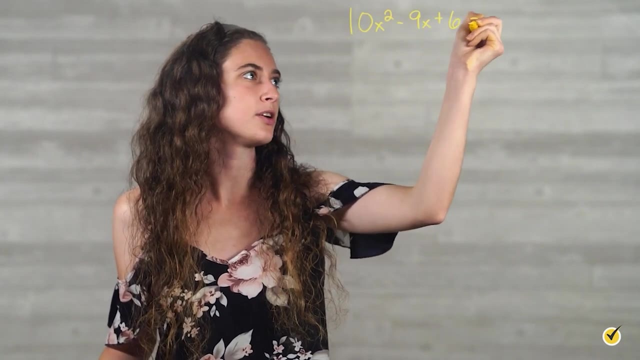 Since it's a positive number, we know that the quadratic equation has two real solutions, which is what we found when we worked it out. Let's look at another example. Consider the quadratic equation: 10x squared minus 9x plus 6 equals zero. 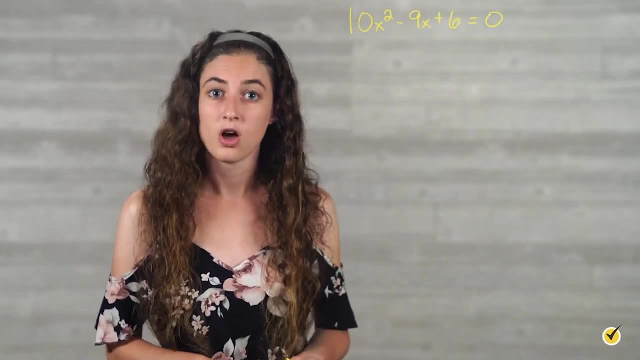 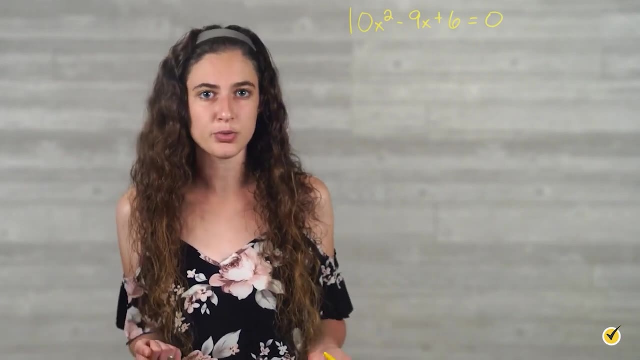 And let's use the quadratic formula to find the solutions for x. First, we need to identify the values for the variables a, b and c in the quadratic equation. Our first term, 10x squared, tells us that a is equal to 10.. 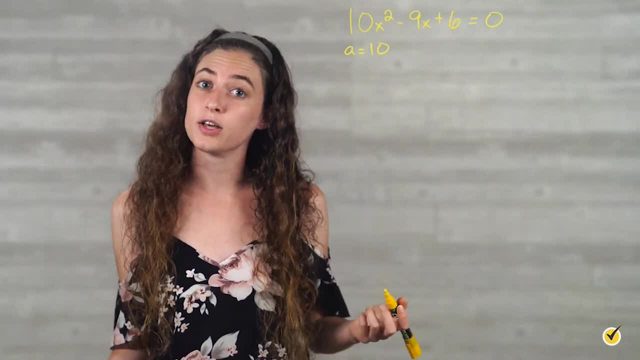 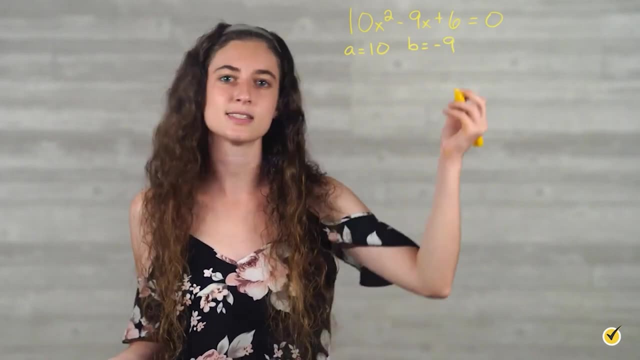 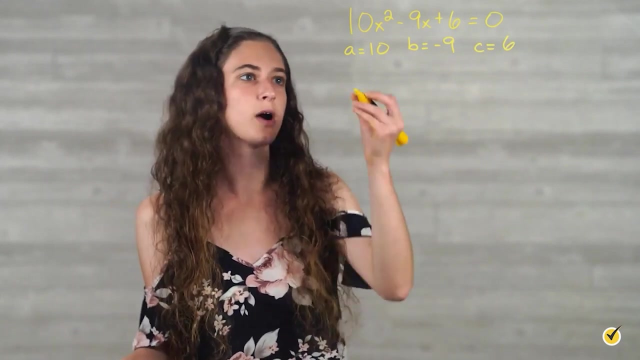 Our second term, negative 9x, tells us that the value of b is negative, 9.. And our third term, plus 6,, tells us that c is equal to 6.. Now we're going to use the quadratic equation to solve this problem. 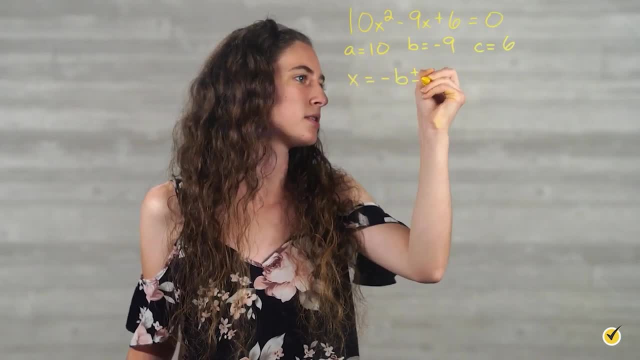 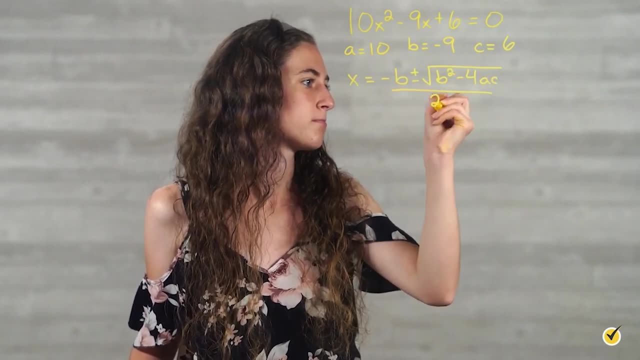 So our formula is: x is equal to negative, b plus or minus the square root of b squared minus 4ac, all over 2a. Now remember: writing out formulas helps you remember it, So whenever you can, it's a really helpful thing to do. 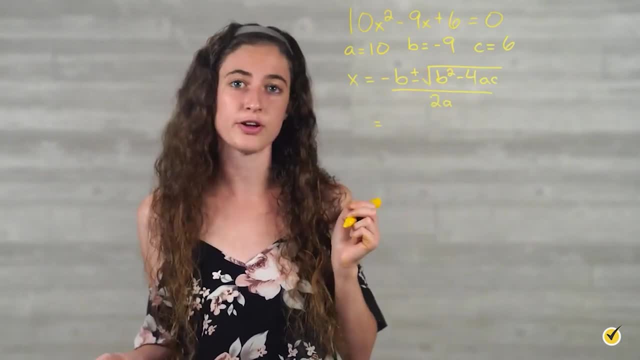 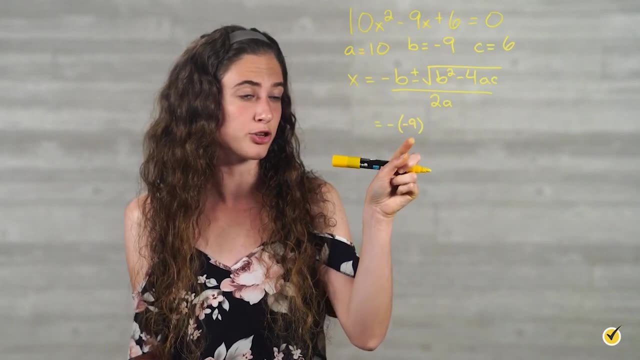 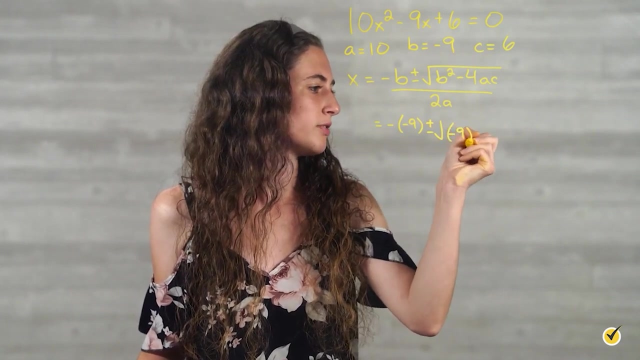 Now all we have to do is plug in our numbers for our variables. So negative b b is negative 9, so be careful when plugging it in. You need to make sure you have the negative negative 9.. Plus or minus, the square root of b squared is negative 9. squared minus 4 times a is 10, times c is 6.. 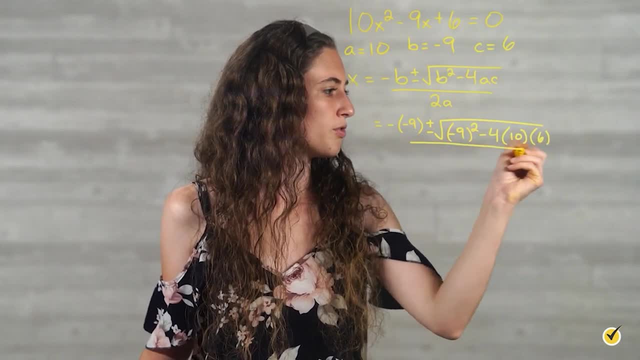 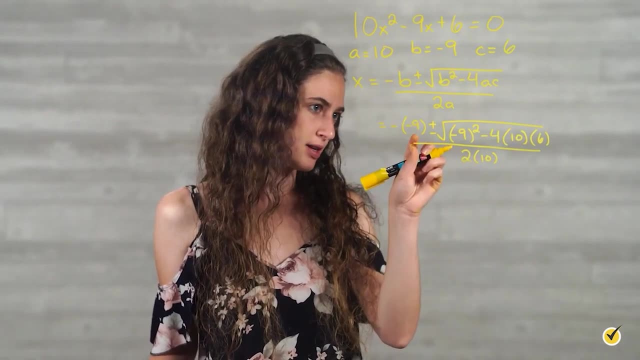 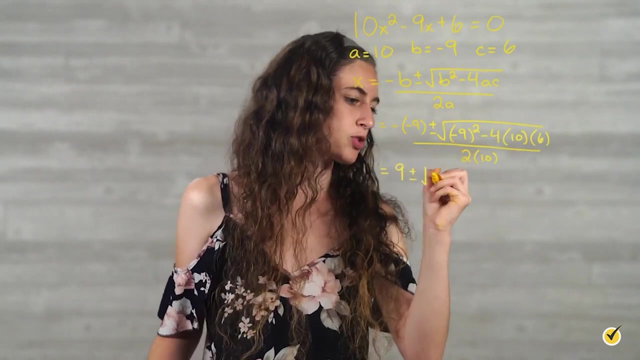 All over 2 times 10.. Which is equal to minus. a negative is equal to a positive, So we're going to have positive 9 right here, Plus or minus. the square root of negative 9 squared is 81.. And then 4 times 10 times 6 is 240.. 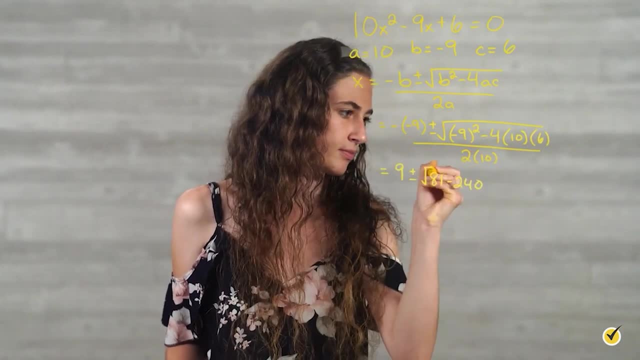 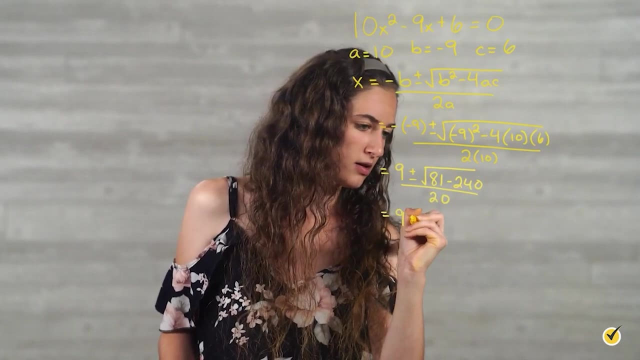 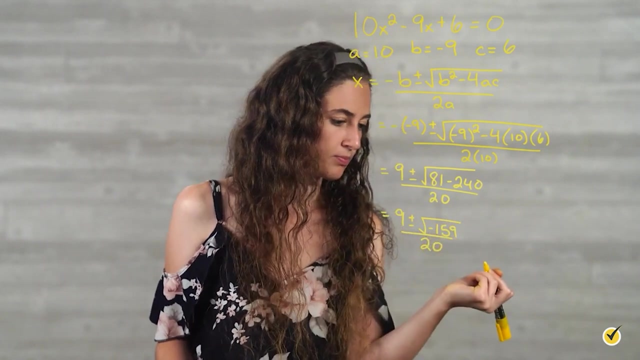 So we have minus 240.. All over 2 times 10 is 20.. So this gives us 9 plus or minus negative 159 over 20.. And we can stop right here because we see our discriminant is negative 159.. 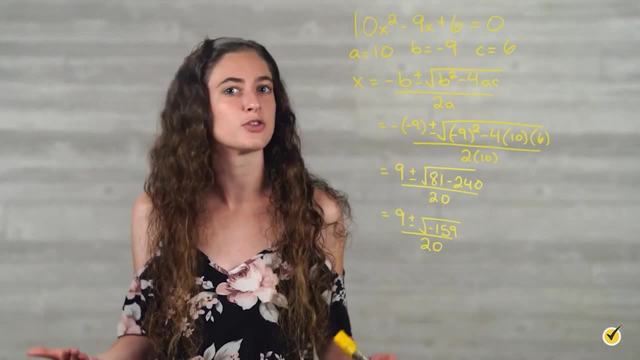 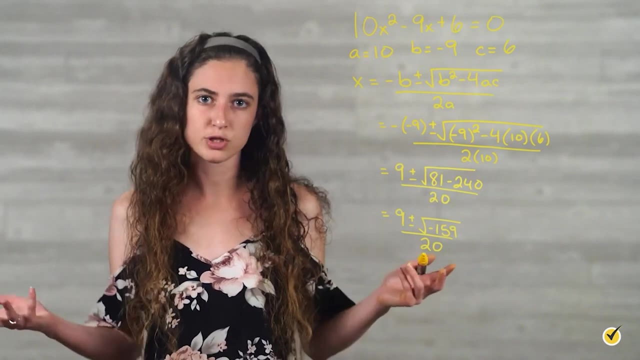 Negative numbers don't have real square roots, because a square is either positive or zero. So remember: if the discriminant is negative number, then there are no real solutions to the equation. So we can stop right here. Our answer is that there is no real solutions for x. 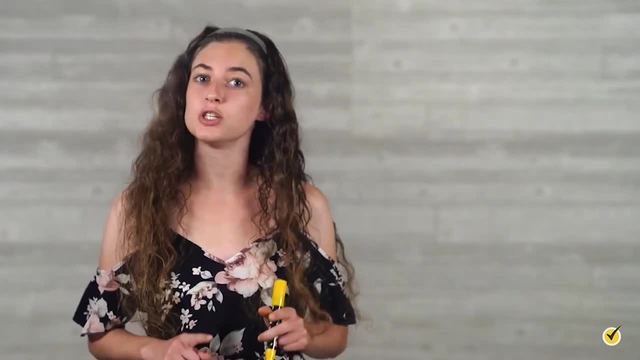 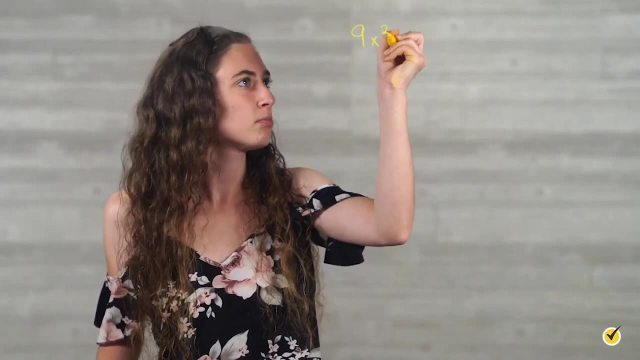 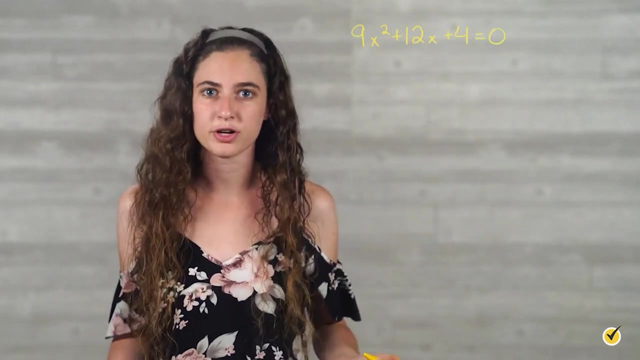 Now it's your turn. I'm going to give you a quadratic equation and you need to use the quadratic formula to identify the possible roots for x. 9x squared plus 12x plus 4 equals 0.. Pause the video here and try it yourself. 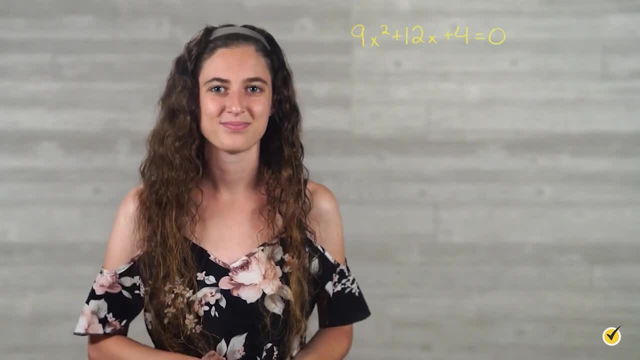 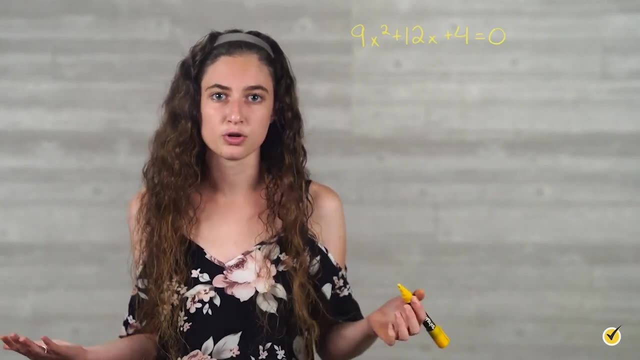 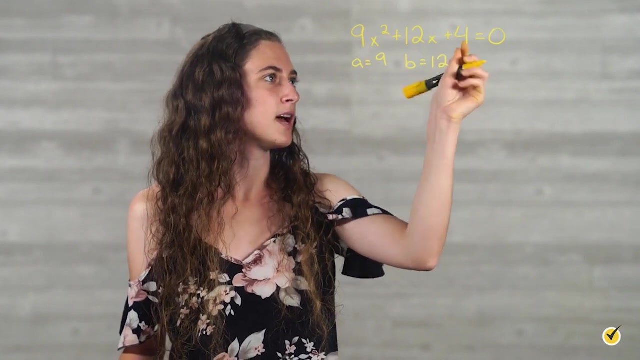 And, when you're done, resume the video and we'll go over everything together. Let's take a look at this one together. Start by identifying the values for a, b and c. Based on the equation, we can see that a is equal to 9,, b is equal to 12, and c is equal to 4.. 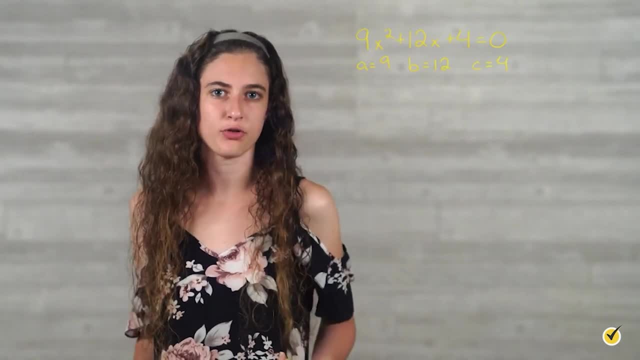 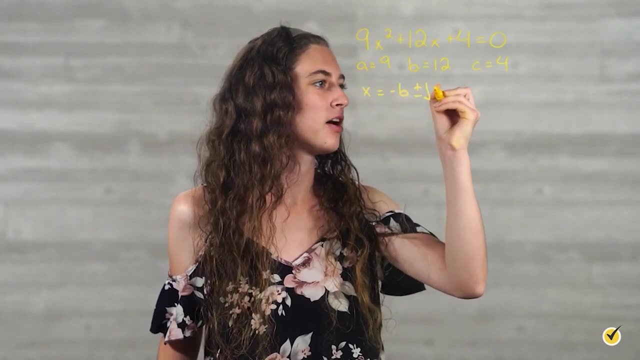 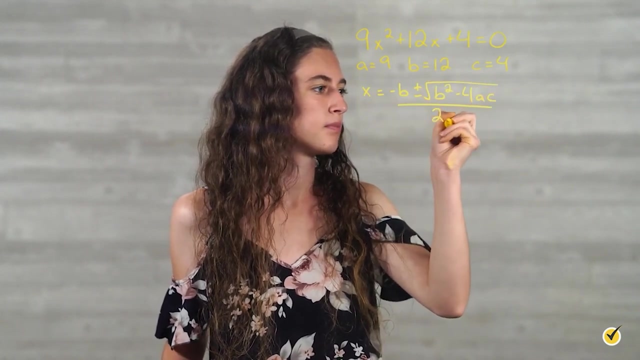 Next substitute the values for a, b and c into the quadratic formula. So remember: the formula is: x is equal to negative b plus or minus the square root of b, squared minus 4ac, All over 2a. And then we just take our numbers up here and plug them in for all our variables. 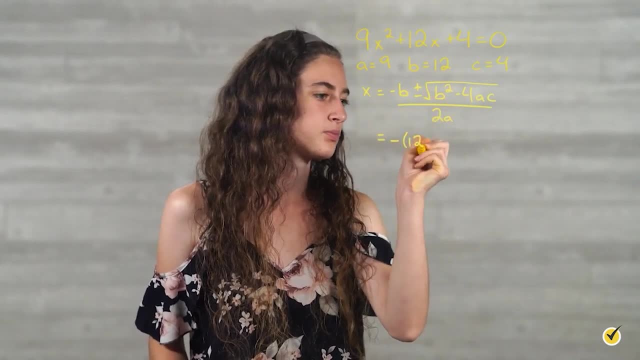 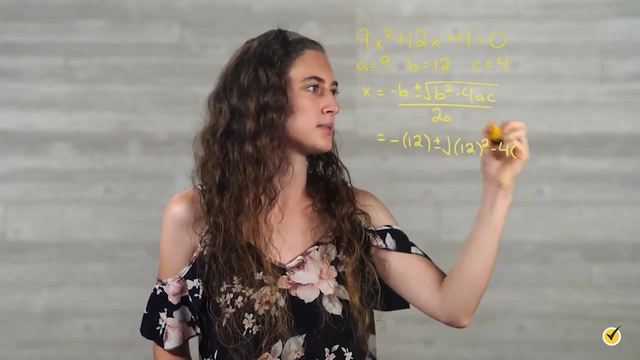 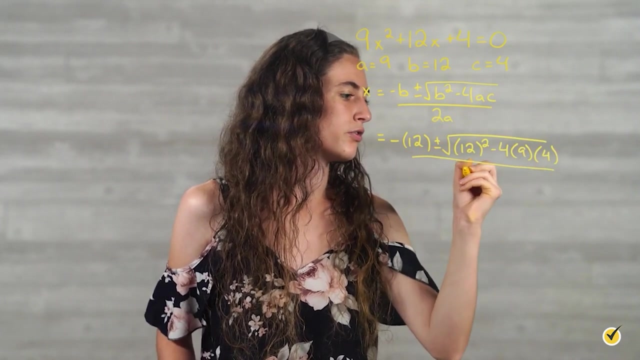 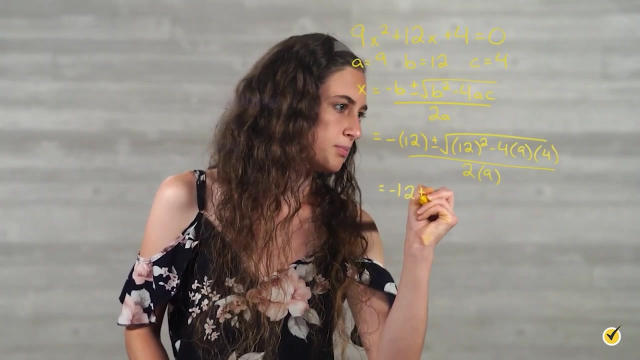 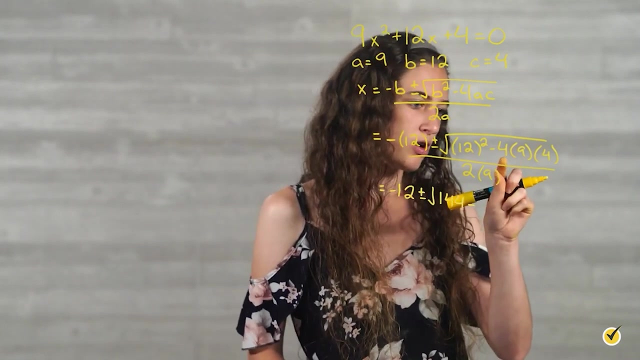 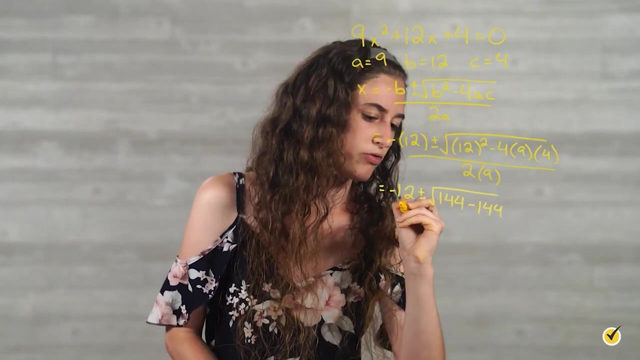 So we have negative 12 plus or minus. the square root of 12 squared minus 4 times 9 times 4, all over 2 times 9.. So this simplifies to negative 12 plus or minus. the square root of 12 squared is 144 minus 4 times 9 is 36 times 4. is 144. all over 2 times 9 is 18.. 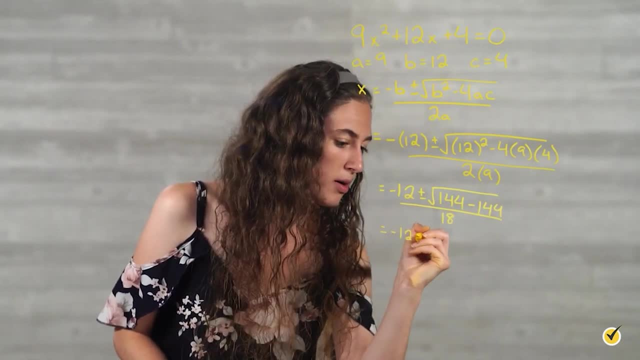 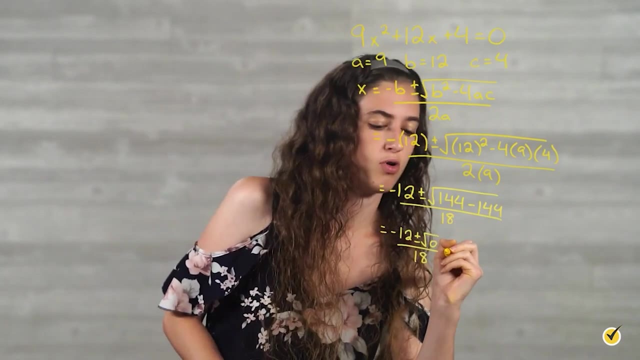 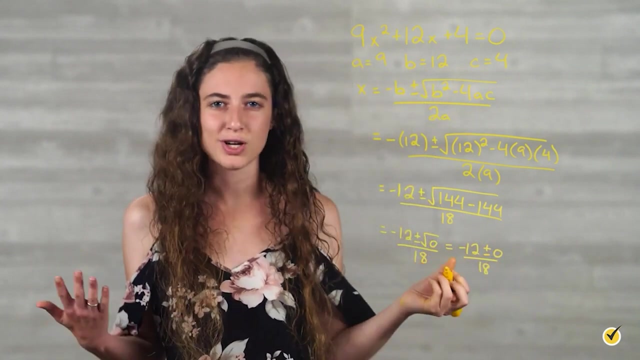 So then we have negative 12 plus or minus the square root of 0 over 18.. The square root of 0 is 0. So all we have is negative 12 plus or minus 0 over 18.. And if you add or subtract 0, that's not going to change your number at all. 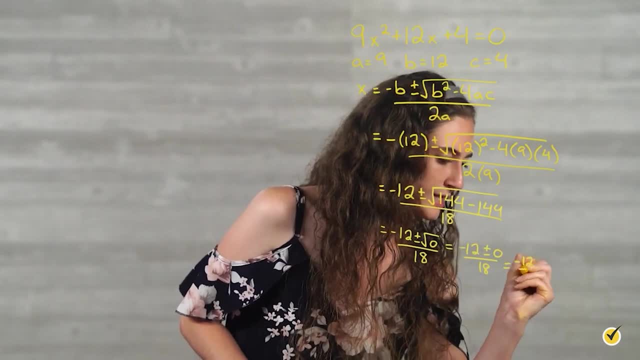 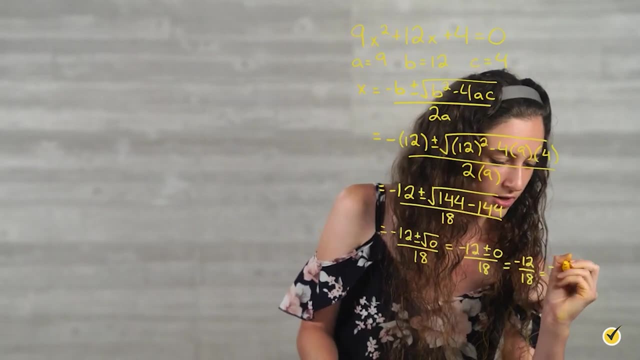 So this is really the same as negative 12 over 18.. Which we can then simplify by dividing both the numerator and denominator by 3.. So that'll give us negative 4 over 6.. And we can simplify that one more time by dividing both by 2.. 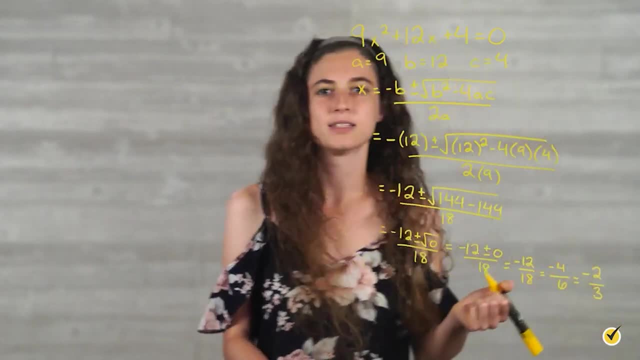 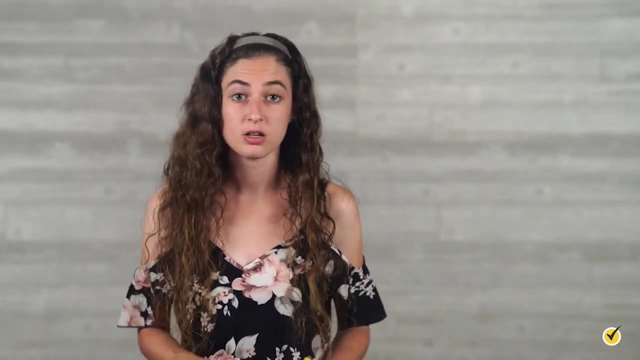 To get negative 2 thirds. So x is equal to negative 2 thirds, And that's our root for this equation. Quadratic functions occur in many real world situations. One example is shooting a cannonball out of a cannon. When you do this, it goes up and then it comes back down in the shape of a parabola. 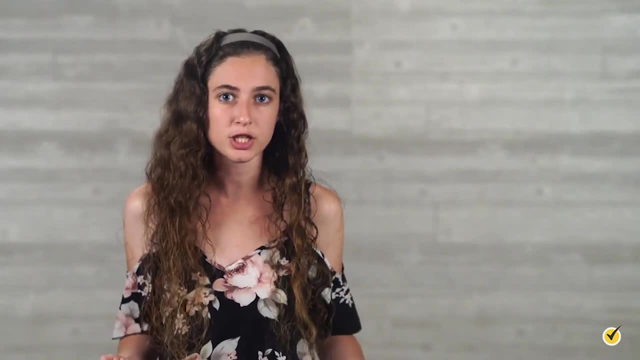 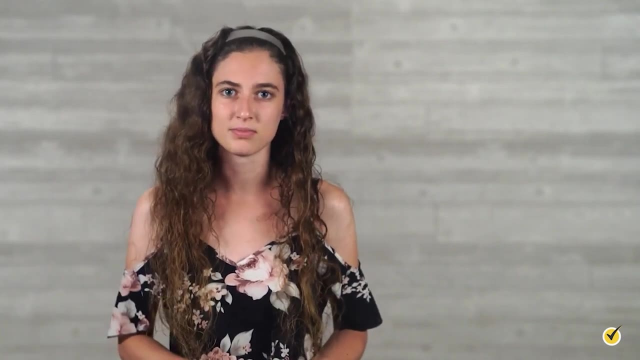 Since a parabola is the graph of a quadratic function, you can use the equation for the path the cannonball follows to answer questions about its time, speed and distance. There are lots of other problem solving instances in which quadratic equations are helpful. 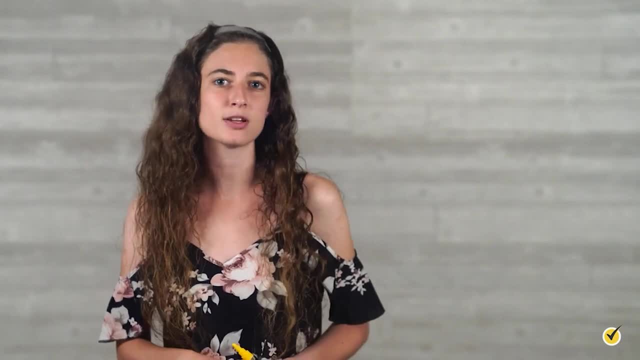 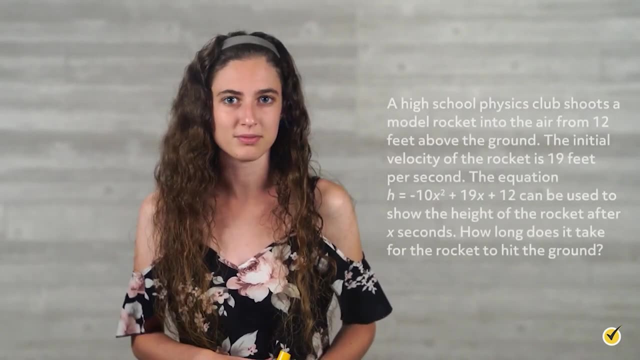 Understanding them helps us apply mathematical concepts in the real world. I have one more problem for you to try. Let's take a look at a word problem that we can solve by using the quadratic formula. A high school physics club shoots a model rocket into the air from 12 feet above the ground. 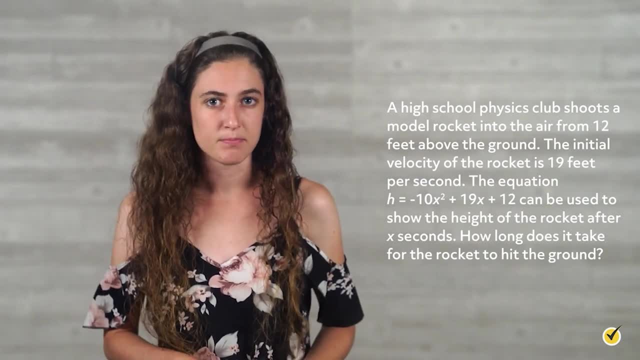 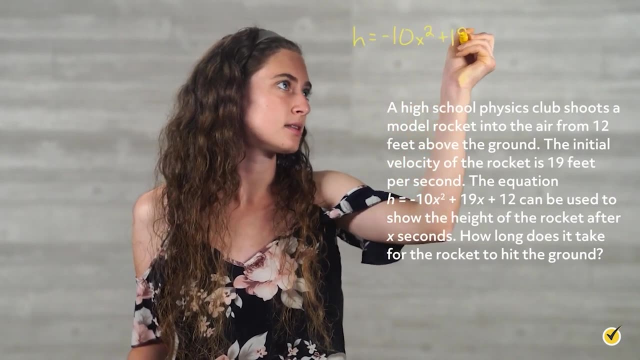 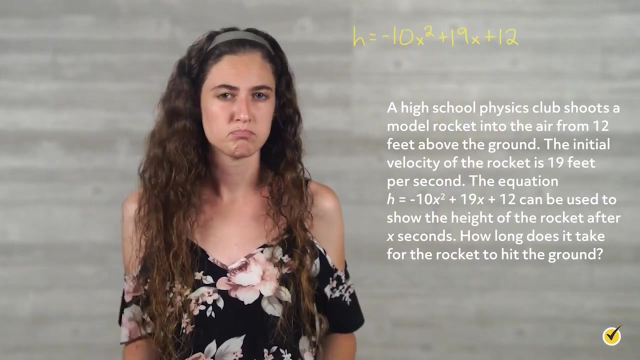 The initial velocity of the rocket is 19 feet per second. The equation h equals negative 10x squared plus 19x plus 12.. Can be used to show the height of the rocket. after x seconds. How long does it take for the rocket to hit the ground? 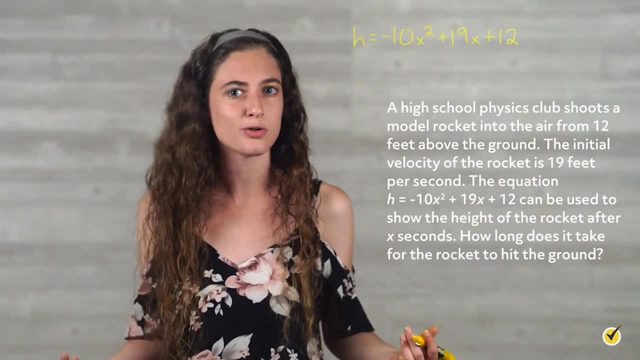 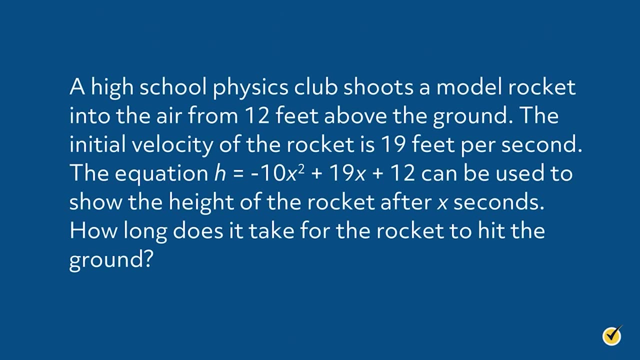 We can solve this problem by applying the quadratic formula to the equation given in the scenario. This problem is a little bit more challenging, but I know you can handle it. Pause the video here and try it yourself, And when you're done we'll go over it together. 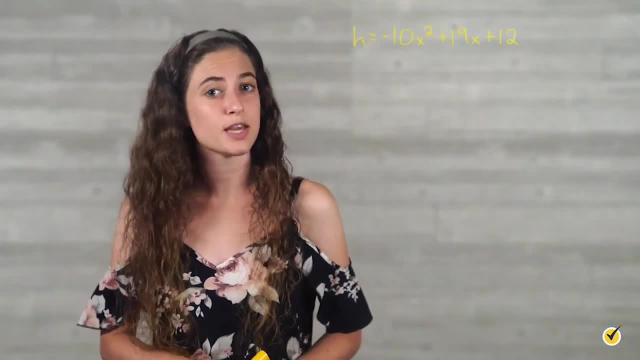 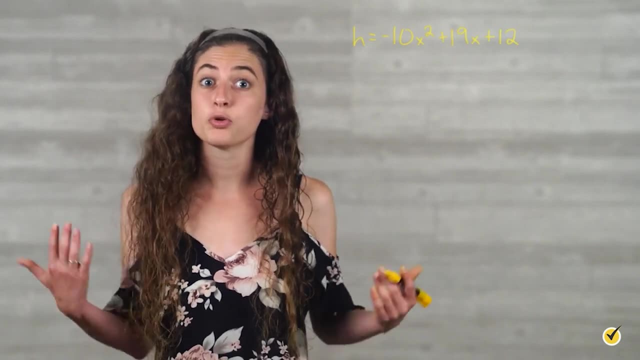 Let's take a look at this one. In this scenario, we are looking for the amount of time it takes for the rocket to reach the ground. The height h at ground level is 0 feet. Therefore, we can replace 0 for h in the equation. 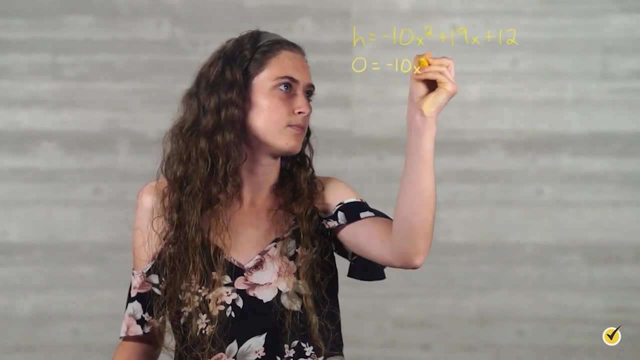 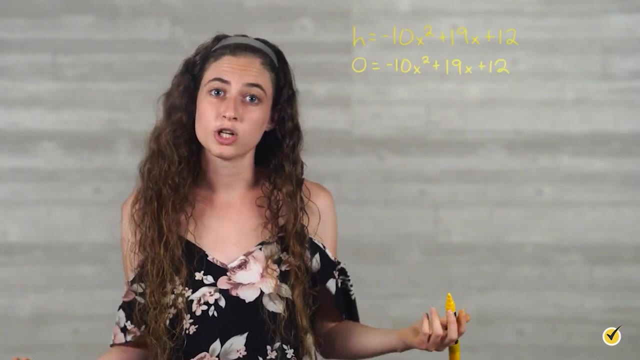 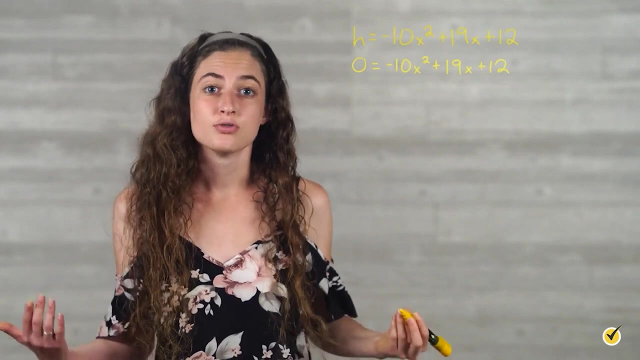 So we can rewrite it as: 0 equals negative 10x squared plus 19x plus 12.. And now it looks like our quadratic equation in standard form, just with our 0 on the left side instead of the right side. So now that we understand that our equation is really just in standard form, 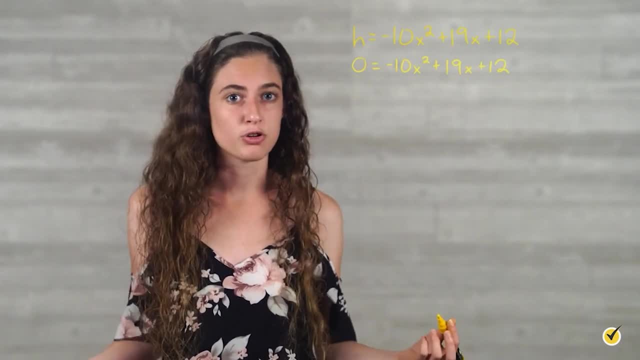 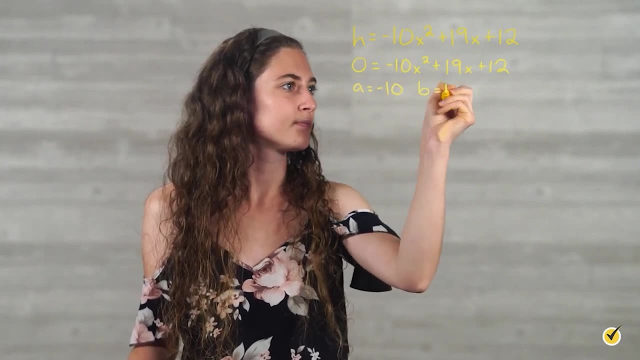 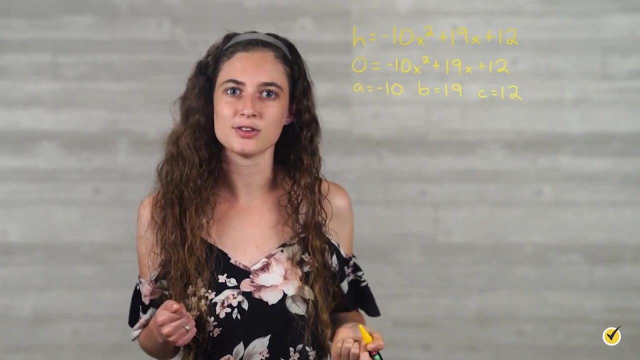 we can identify the values for a, b and c Based on our equation. we see that a is equal to negative 10.. b is equal to 19. And c is equal to 12.. Now we can substitute these values into our quadratic formula. 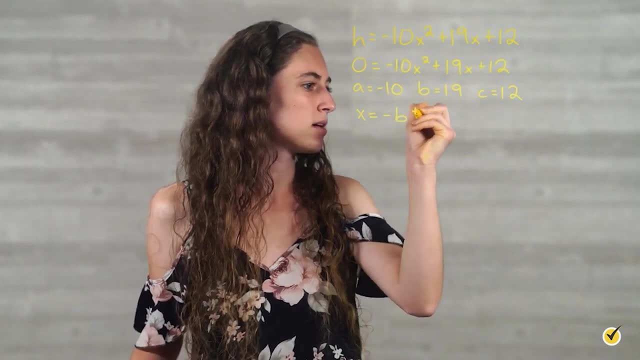 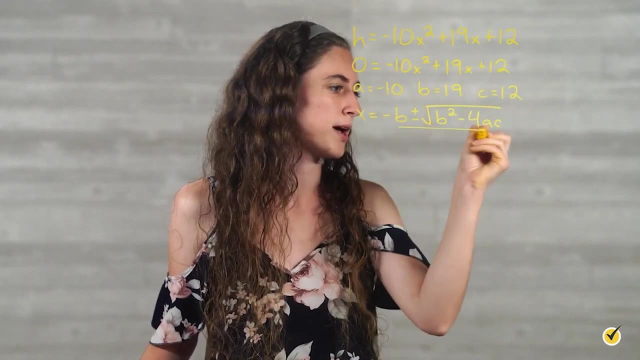 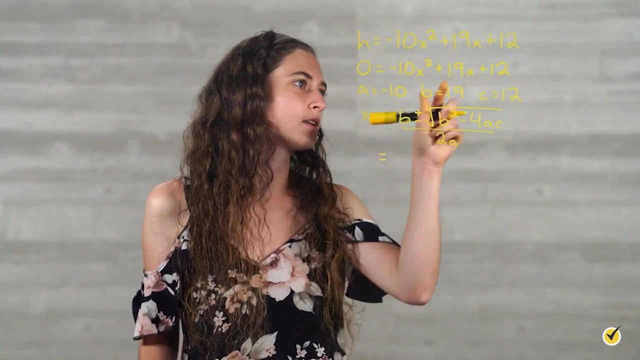 So we have the formula again: is: x is equal to negative b, plus or minus the square root of b squared minus 4ac, All over 2a. Now we can plug in our numbers. So we have: x is equal to negative b, so negative 19.. 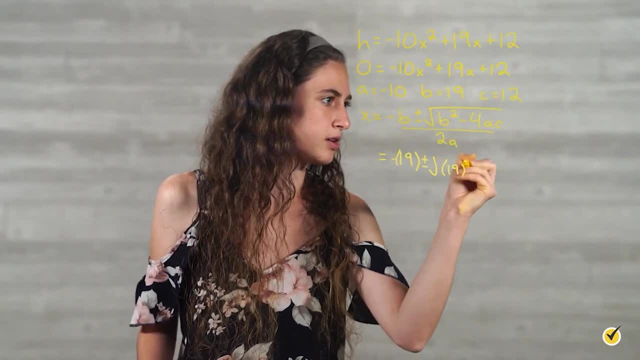 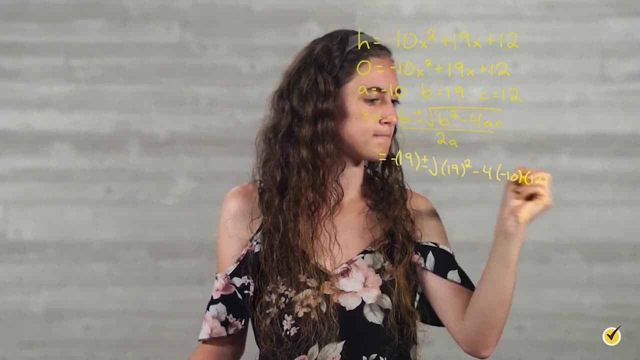 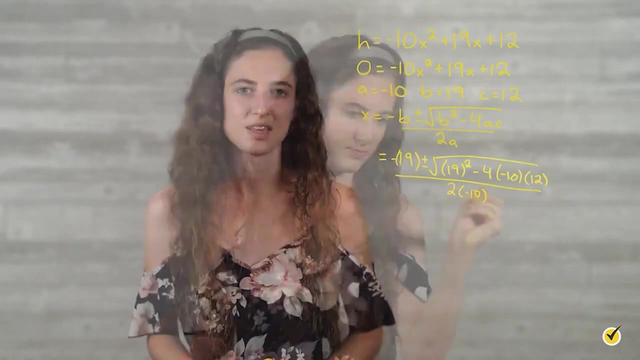 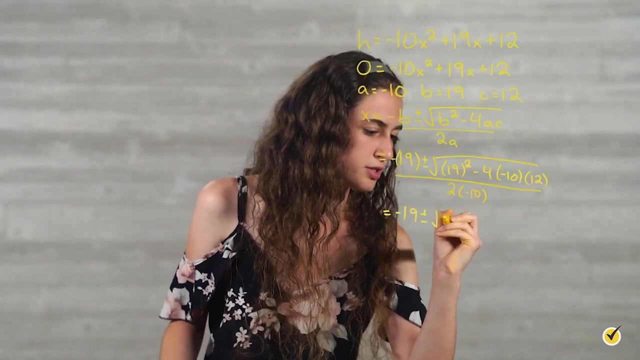 Plus or minus. the square root of 19 squared minus 4 times negative, 10 times 12.. All over 2 times negative 10.. So this is equal to negative 19 plus or minus. the square root of 19 squared is 361.. 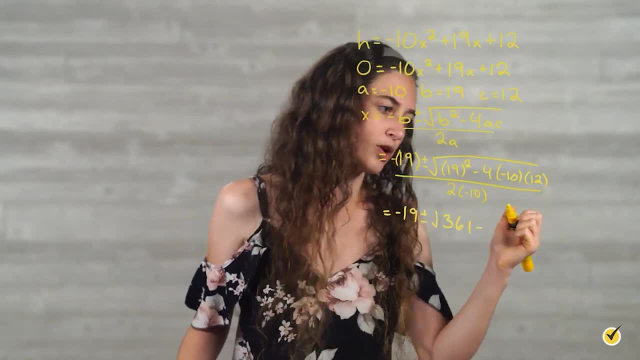 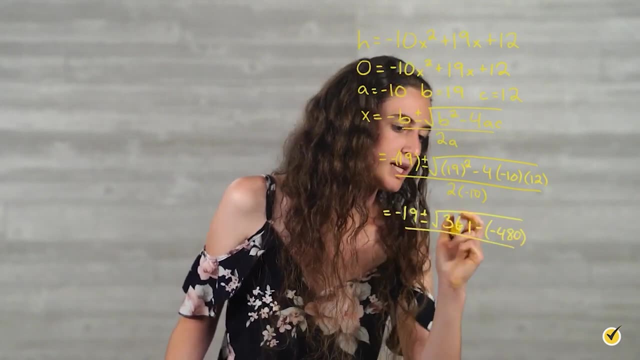 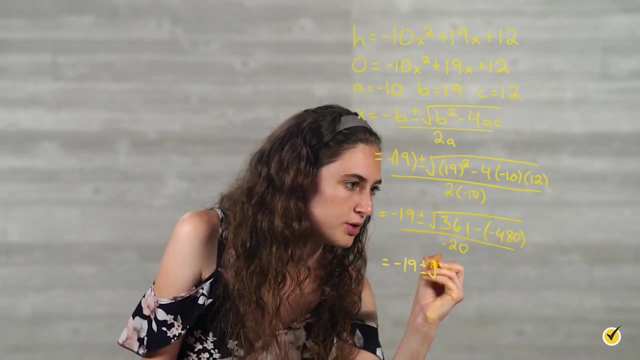 Minus 4 times negative. 10 times 12 is negative 480.. Over 2 times negative 10 is negative 20.. So this is equal to negative 19 plus or minus the square root of 361.. 361 minus negative 480 is the same as saying plus 480.. 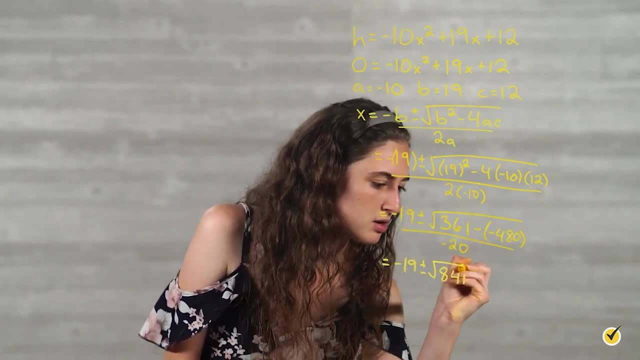 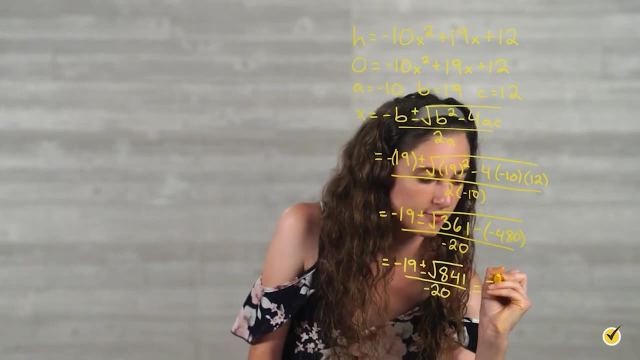 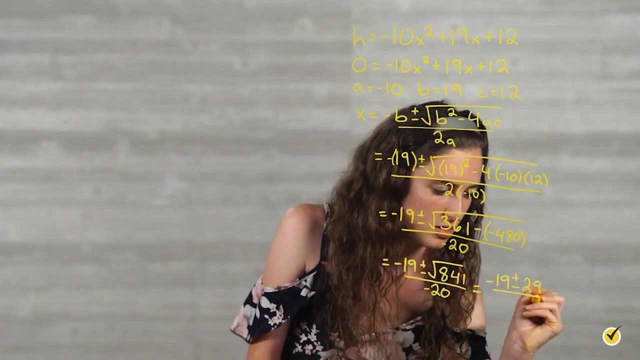 So the square root of 841.. That's what you get when you add those two numbers together Over negative 20.. So this is equal to negative 19 plus or minus. the square root of 841 is 29 over negative 20.. 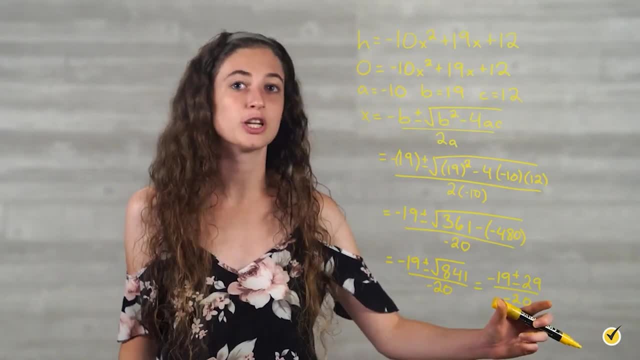 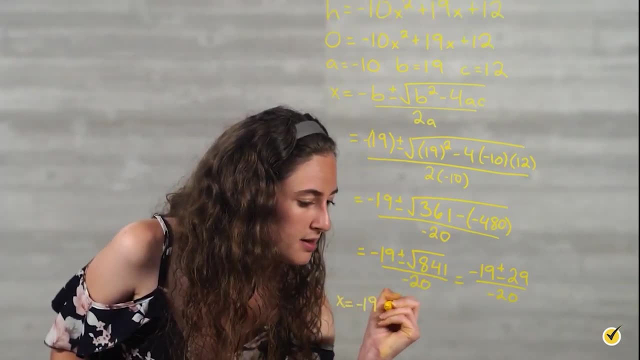 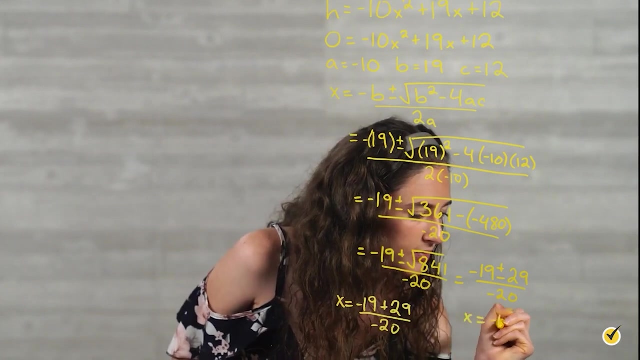 And now, from this step, we're going to take this equation and break it into two separate equations Because of this plus or minus. So we're going to have: x is equal to negative 19 plus 29 over negative 20.. And we're also going to have: x is equal to negative 19 minus 29 over negative 20.. 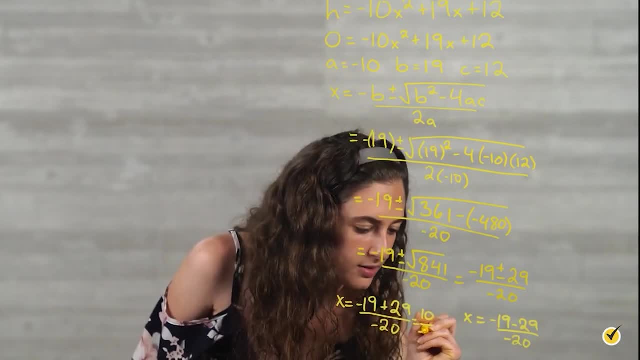 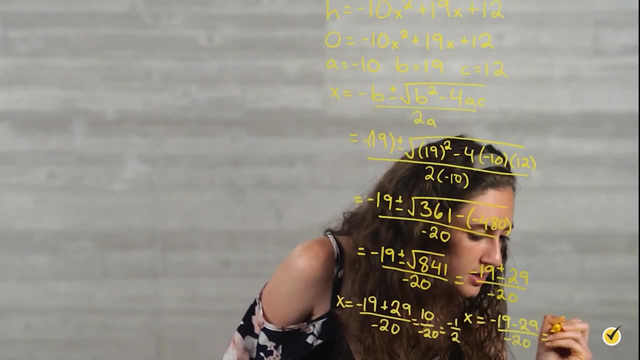 Negative 19 plus 29 is equal to 10 over negative 20.. Simplifies to negative 1 half And over here, negative 19 minus 29 is negative 48. Over negative 20.. Our negatives will cancel each other out. 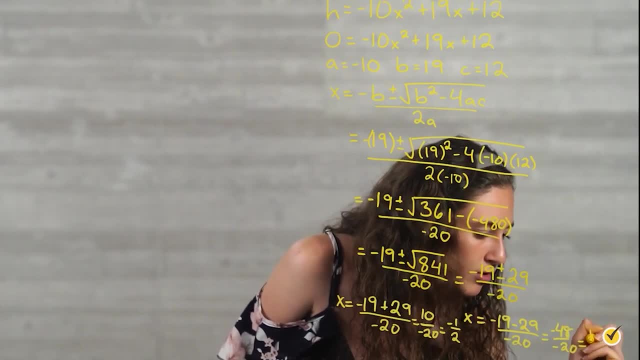 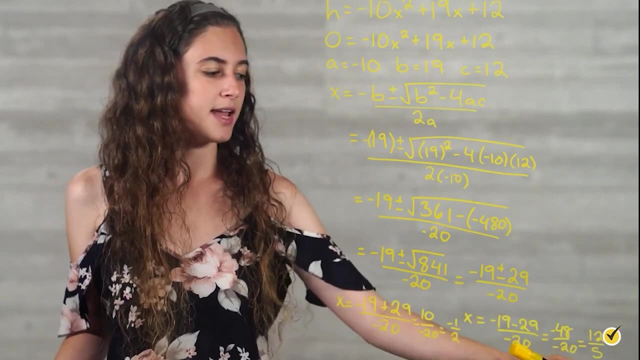 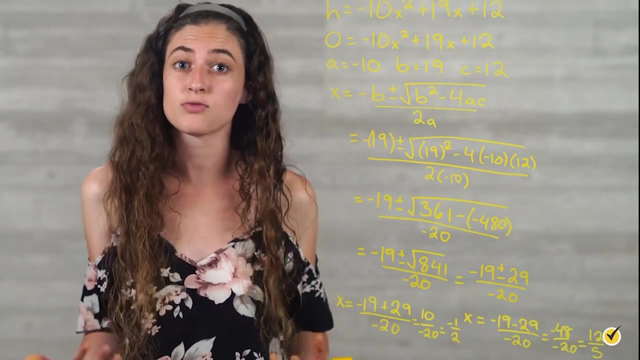 And if we divide both the numerator and denominator by 4, we'll get 12 over 5.. So the solutions to this equation are: x equals negative 1 half and x equals 12 over 5.. Now that we have the two roots for x, we must interpret what they mean in the context of the word problem. 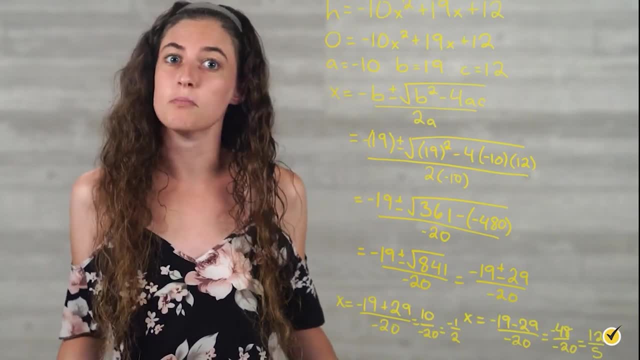 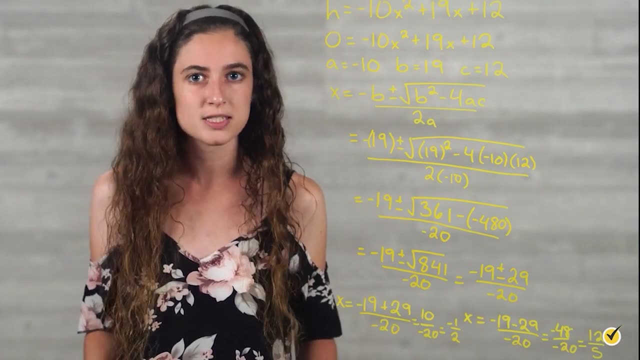 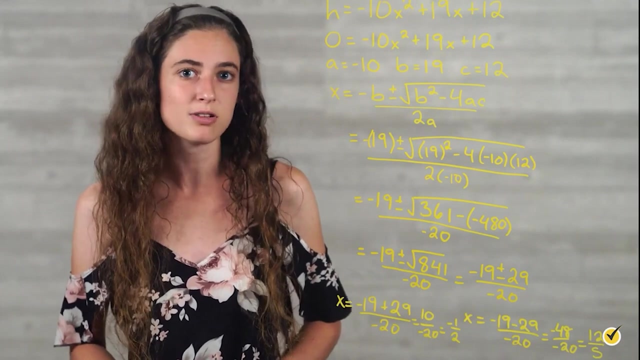 Recall that x stands for seconds, Measuring the amount of time it takes for the model rocket to hit the ground. Time is measured with positive numbers, not negative numbers. Therefore, the negative root of x does not apply to this scenario. Based on the positive solution for x, the amount of time that it will take for the rocket to hit the ground is 12 over 5 seconds. 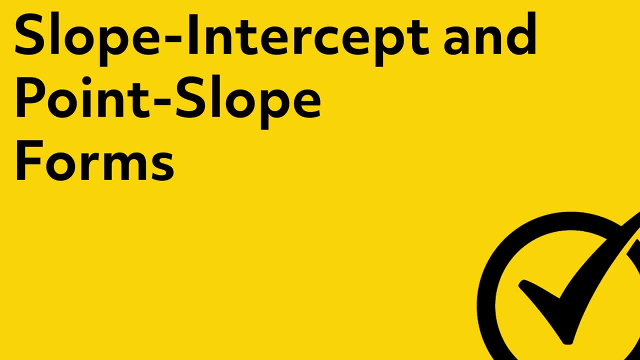 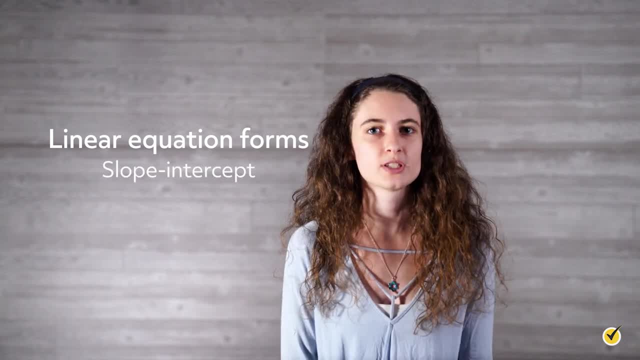 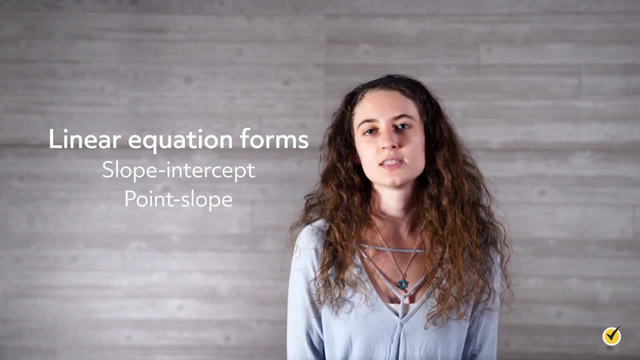 Great work, Hi, and welcome to this review of linear equation forms. Specifically, we'll be talking about slope-intercept and point-slope forms. We will also review the terminology And the process of graphing linear equations in these forms. Let's get started. 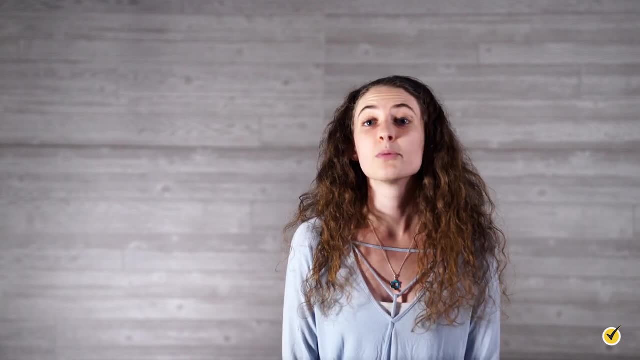 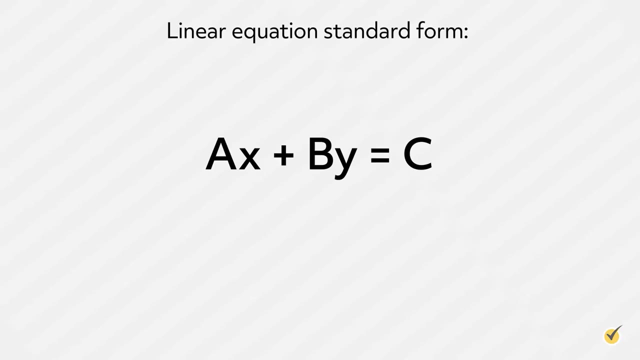 A linear equation can be expressed in many different ways, But no matter which form you use, it just represents a straight line. The standard form of a linear equation is written as ax plus by equals c, Where a, b and c are constants. 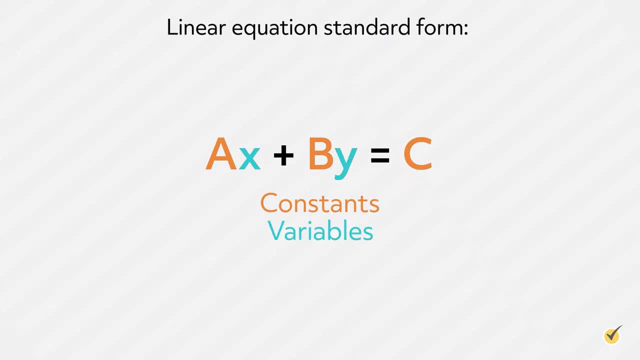 And x and y represent variables. This form of the equation is very useful for some purposes. in math, For example, A line can be quickly graphed when it is in this form, by finding the x and y intercepts. There are also methods of solving systems of equations that require each equation in the system to be written in this form. 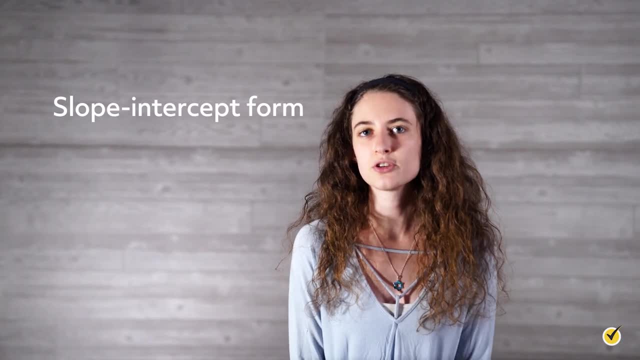 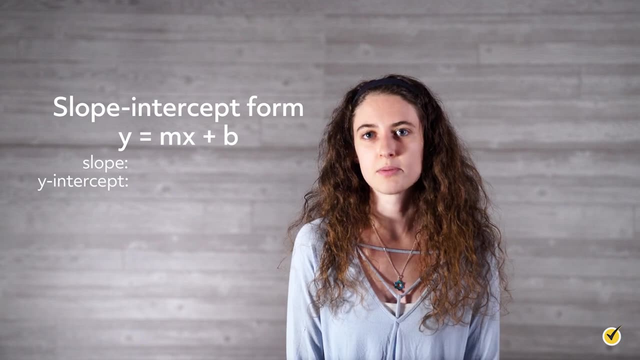 Rearranging this standard form equation into slope-intercept form- y equals mx plus b- reveals other key features of the line, Namely the slope and the y-intercept. The slope of a line describes the slant or steepness. 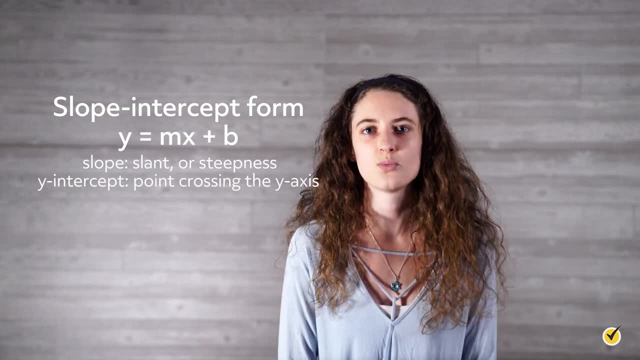 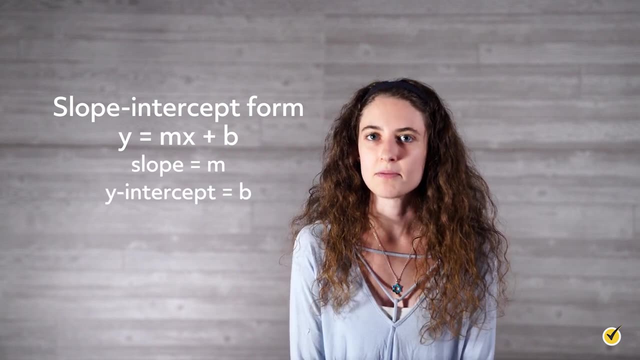 And the y-intercept is the point on the graph Where the line crosses the y-axis. Notationally, slope is represented by m And the y-intercept is represented by b, Because the y-intercept is an actual point on the coordinate plane. 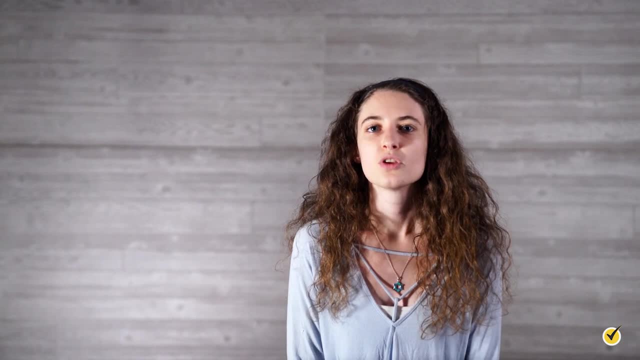 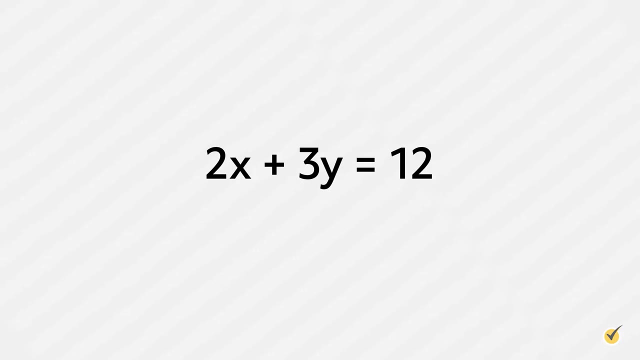 It is represented as an ordered pair: 0, b. Sometimes you will be asked to rearrange an equation from one form to another. Here's an example: 2x plus 3y equals 12.. Remember The standard form of a linear equation. 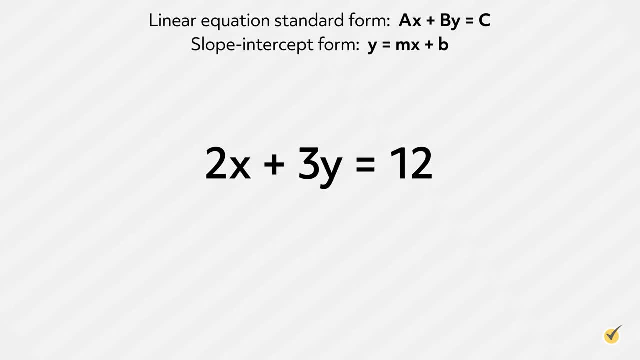 Is ax plus by equals c. So this is currently in standard form. If we want to change it to slope-intercept form, We are going to need to rearrange it so that y is by itself on our left side. Our first step is to subtract 2x from both sides. 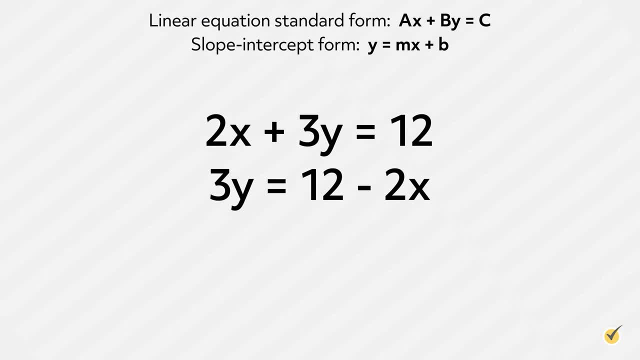 3y equals 12 minus 2x Is what we have now. Then we're going to divide everything by 3. Which gives us y equals 4 minus 2 thirds x. This is almost right, But if we look again at slope-intercept form, 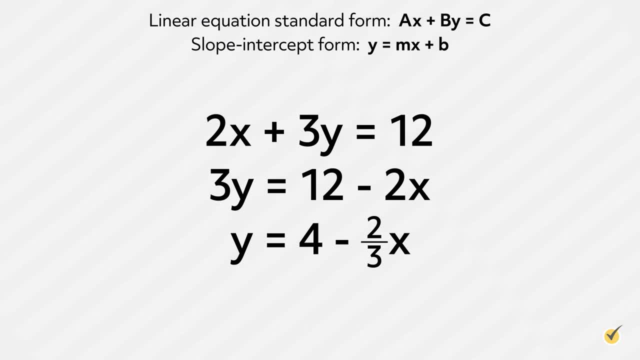 We see that we need the x term to be in front. Thankfully, we can think of this as 4 plus negative 2 thirds x And use the commutative property of addition to swap their places. This gives us y equals negative 2 thirds x plus 4.. 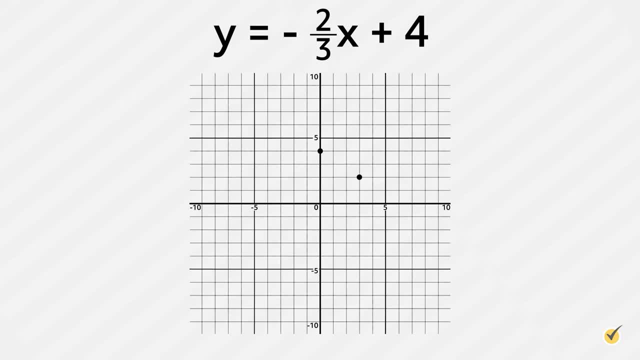 The resulting equation is more informative about the line than the original equation in standard form. The coefficient of x negative 2 thirds Is the slope A negative slope. A negative slope tells us that the line slants downward from left to right. The y-intercept of 4 tells us that the line crosses the y-axis at the point. 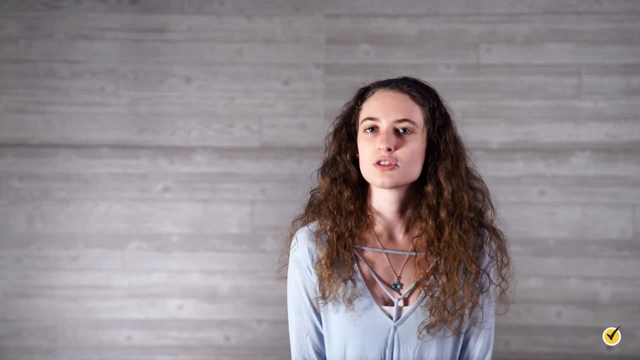 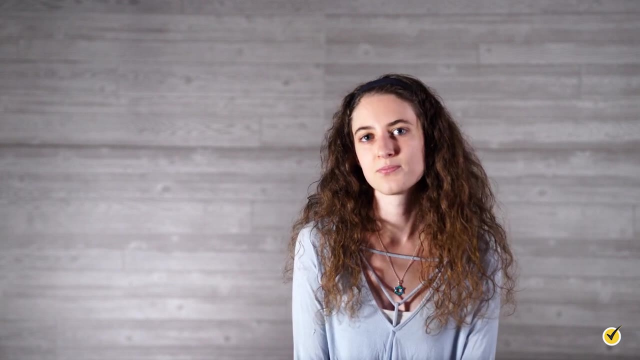 Now that we have seen how to convert a standard form equation into slope-intercept form, Let's practice recognizing the key features of slope and the y-intercept with a few examples. For these examples, we want to name the slope, Describe the slant of the line. 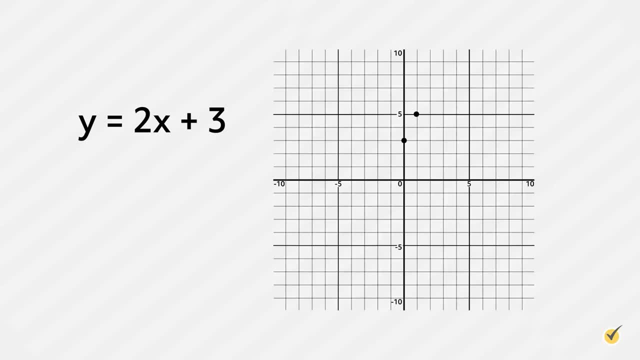 And name the y-intercept as an ordered pair. y equals 2x plus 3.. The slope of this equation is m equals 2.. The coefficient of the x variable- A positive slope- indicates that the line slants upward from left to right. 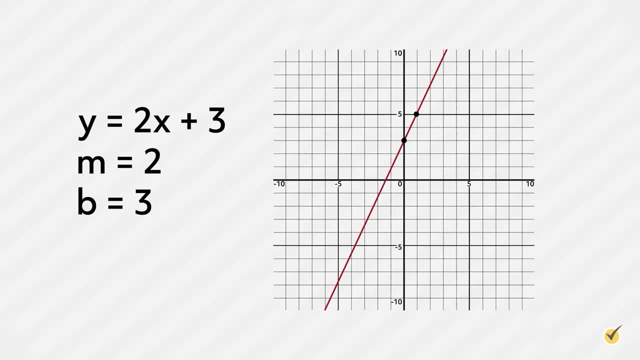 The y-intercept is: b equals 3.. Which indicates that the line crosses the y-axis at the point. Let's try another one. y equals 3 fifths x minus 2 thirds. The slope of this equation is: m equals 3 fifths. 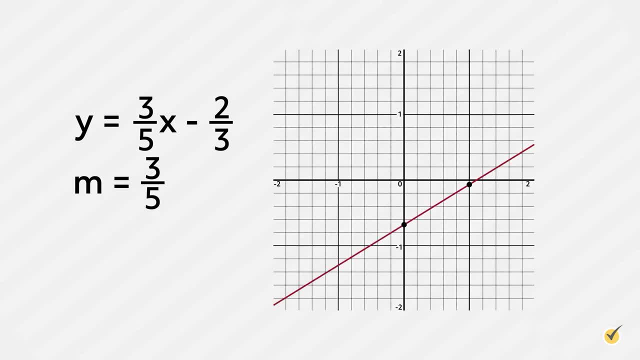 Because the slope is positive, the line slants upward from left to right. The y-intercept is negative 2 thirds, Which indicates that the line crosses the y-axis at the point. Let's try one more: y equals negative 5x minus 2.. 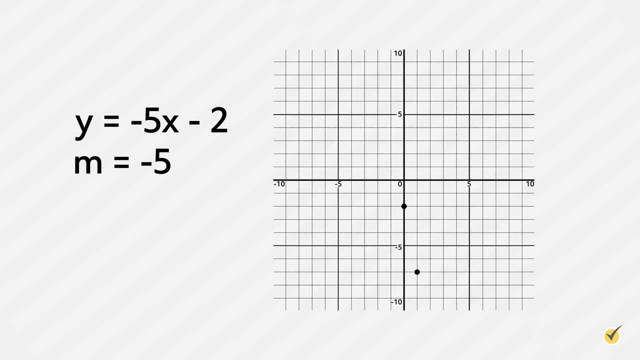 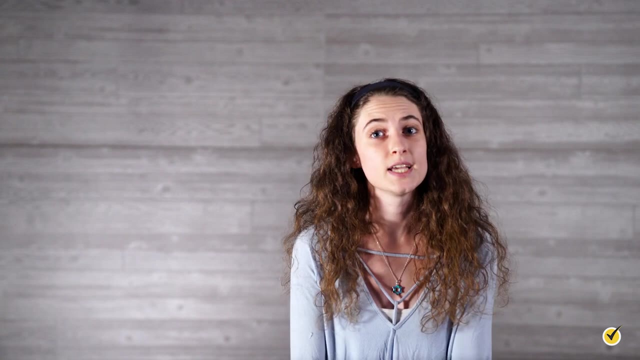 The slope is m equals negative 5. Negative slope means that the line slants downward from left to right. The line crosses the y-axis at the point. As you can imagine, knowing where the line crosses the y-axis and the slope of the line will make the line very easy to graph. 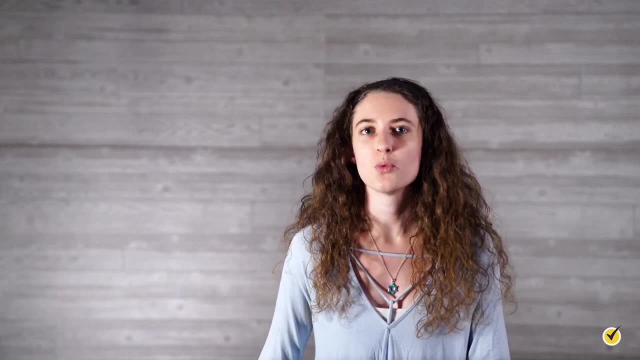 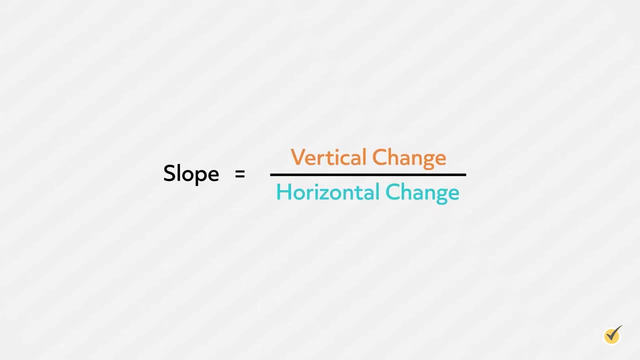 Now let's take a look at how slope provides you with instructions to graph from the y-intercept. Any value of slope can be looked at as a fraction, Where the numerator indicates where to move along the y-axis and the denominator indicates where to move along the x-axis. 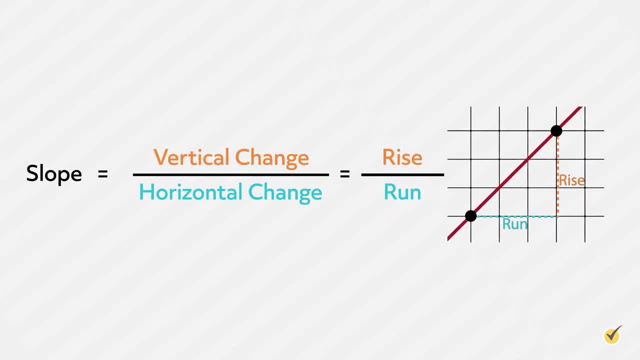 Movement along the y-axis is typically referred to as the rise. A positive rise value would instruct a move up the y-axis, while a negative rise would indicate a move down the y-axis. Likewise, a positive run value would mean a shift to the right and a negative run would mean a shift to the left. 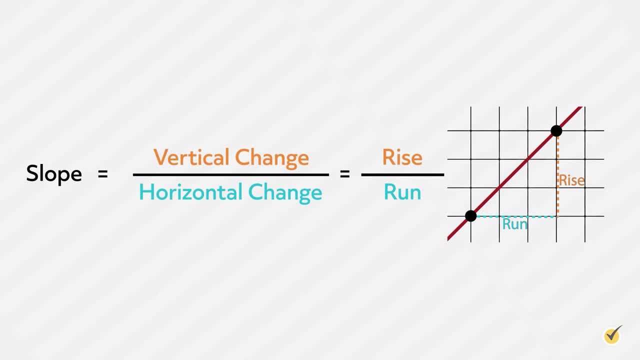 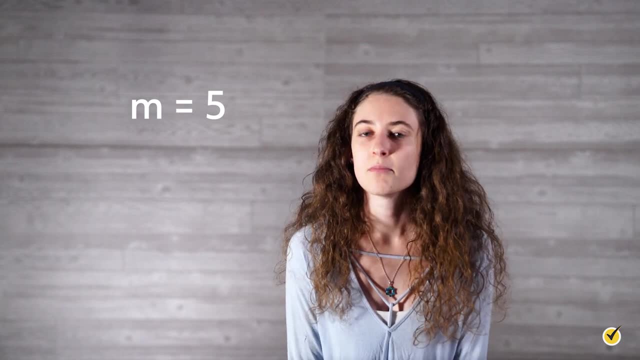 Here are a few examples to practice identifying the rise and run indicated by a given slope: m equals 5.. This slope is not written as a fraction, but any whole number can be rewritten as a fraction over 1. m equals 5.. 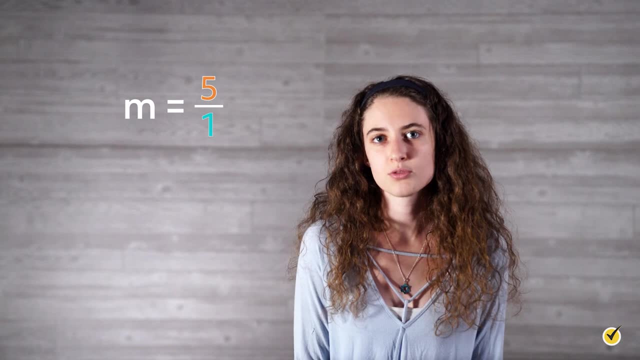 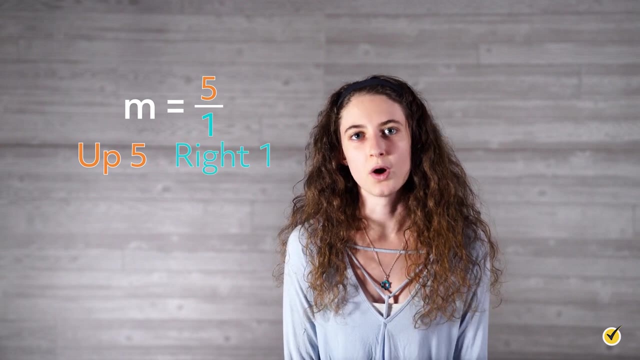 m equals 5 over 1. The numerator 5, is the rise. The positive value means up, 5. The denominator is the run. Positive value means right, 1. Let's try another one. m equals negative 2 thirds. 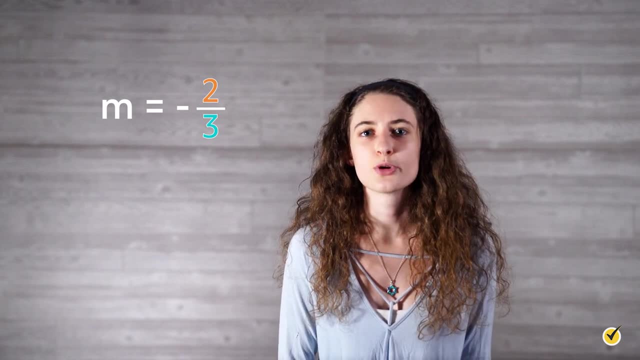 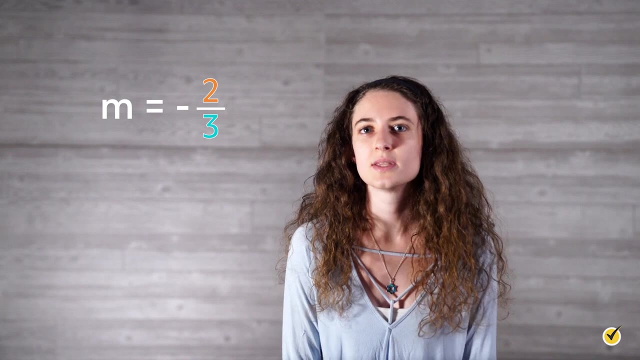 When you have a negative slope, you can consider either the numerator or the denominator to be negative, not both. For this example, let's consider the numerator the rise to be the negative value. Negative value means down: 2.. The denominator 3, is the run. 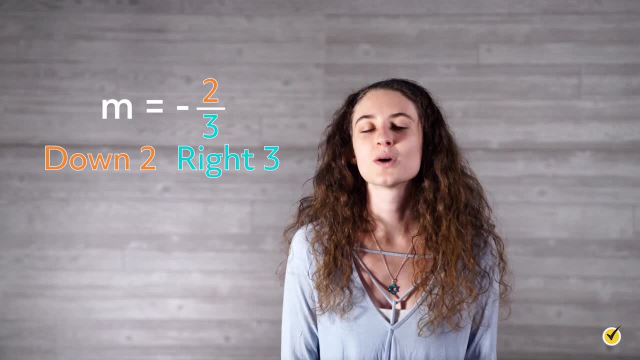 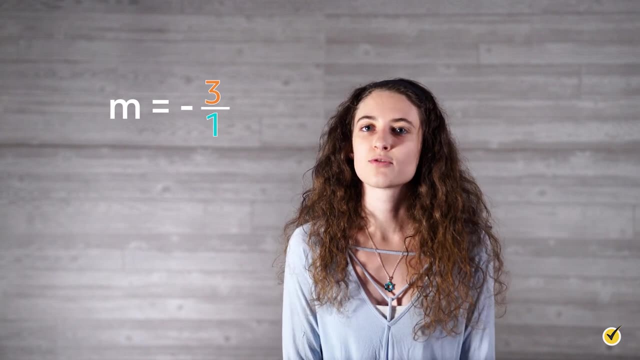 Positive value means right 3.. Here's one last example: m equals negative 3.. First we need to rewrite the whole number as a fraction: Negative 3 over 1. Let the numerator be the negative value. Rise is negative 3.. 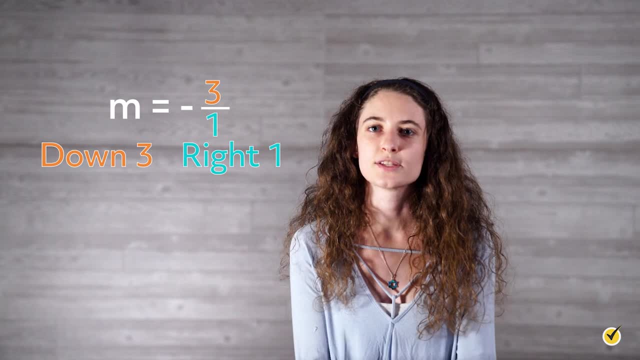 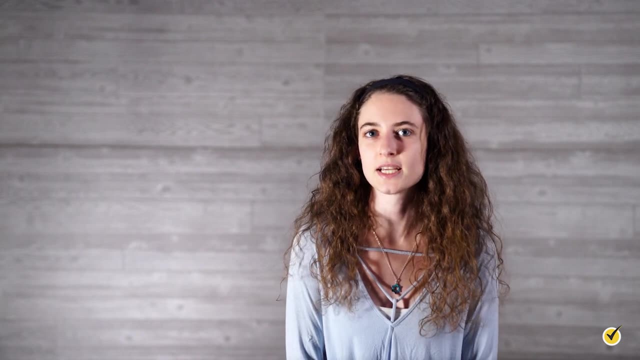 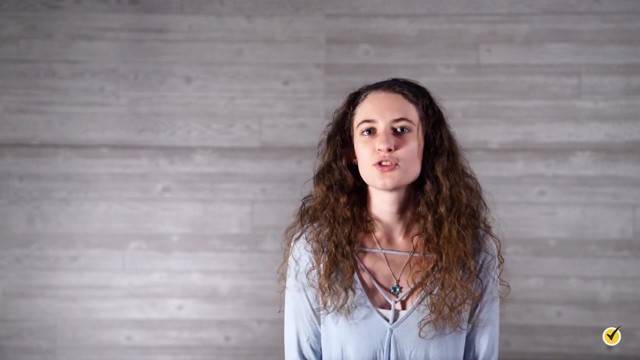 Down 3.. Run is 1.. Right, 1.. Now on to some graphing. People sometimes find it helpful to use the notation of slope-intercept form. to get started, Begin at b and move according to m. Let's graph the linear equation in slope-intercept form. 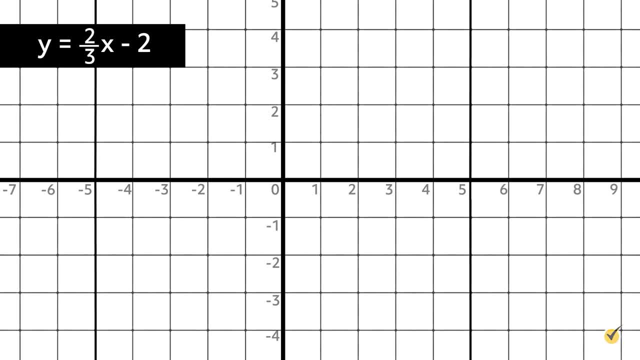 y equals 2 thirds x minus 2.. Step 1. Begin at b. Plot the y-intercept 0, negative 2.. First point. Step 2. Move by m equals 2 thirds. Rise equals up 2.. 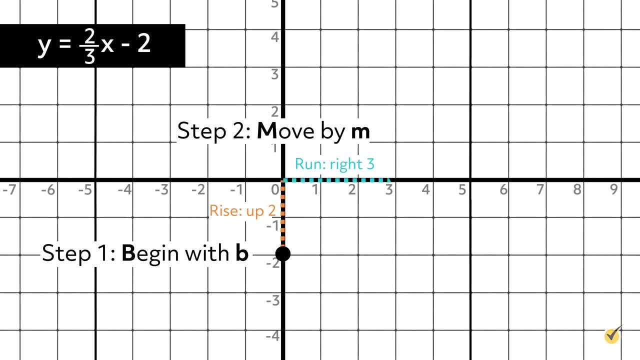 Run equals right. 3. Plot the second point at 3.. 0.. Step 3.. Repeat the rise equals up, 2 and run equals right. 3.. Plot the third point at 6, 2.. Step 4. Draw a straight line through the three points. 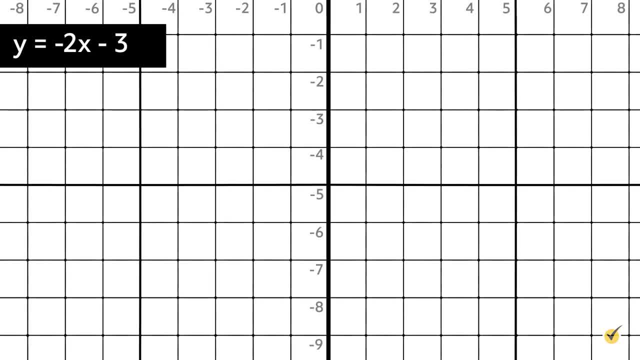 Got the hang of it. Let's try one more. y equals negative 2x minus 3.. Step 1. Begin at b, Plot the y-intercept: 0, negative 3.. First point, Step 2. Move by m equals negative 3.. 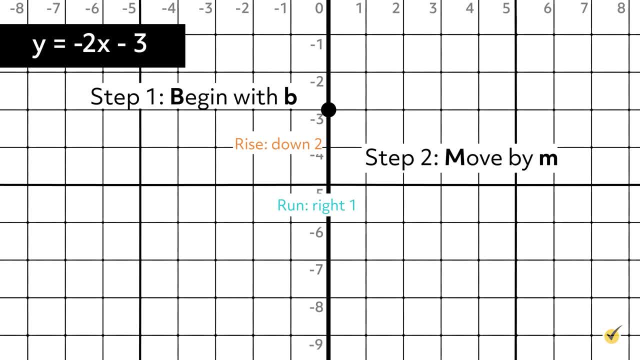 Run equals right. 5. Run equals right. 3. Run equals up. 2. Run equals right. 6. Step 1. Begin at b. Put the y-intercept 2, negative. 2. Let the rise be negative. Rise equals down. 2.. 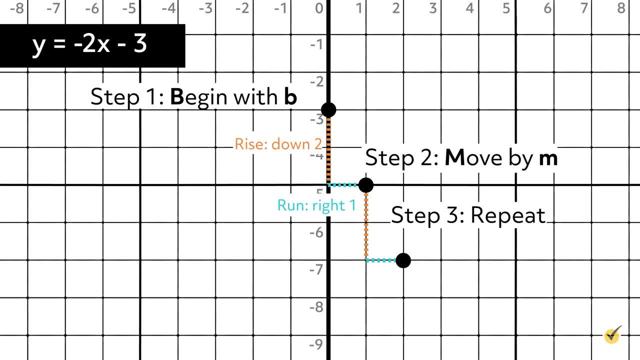 Run equals right. 1. Plot the second point at 1, negative, 5. Step: 3. Repeat the rise equals down 2 and run equals right. 1. Plot the third point at 2, negative, 7. negative slope in this equation. 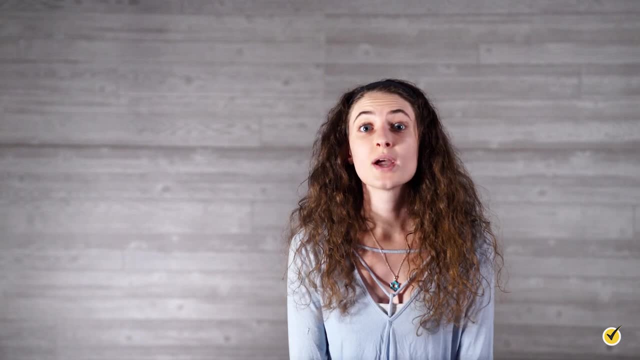 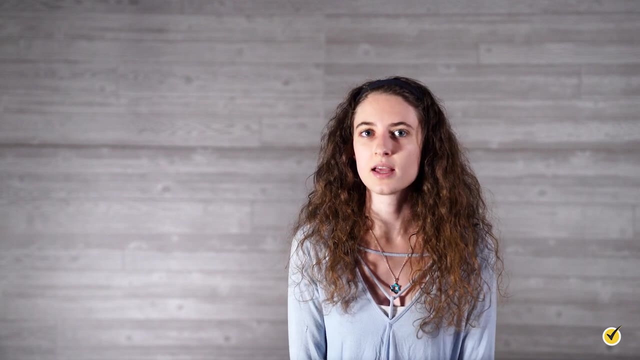 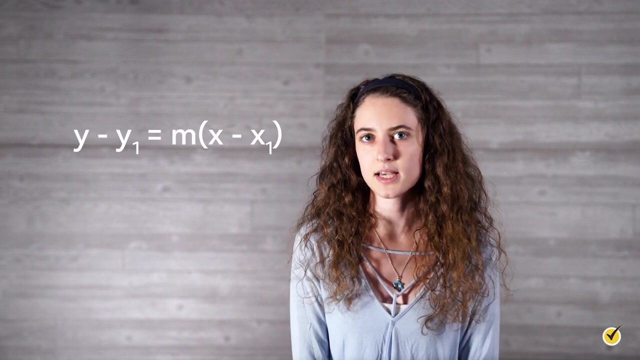 Now that we have had some review of the key features of linear equations, we have the tools to explore the point-slope form. This form is of special use if we know one point that is on the line and the slope. The general form of this arrangement is: y-y1 equals m times x-x1, where m equals the slope. 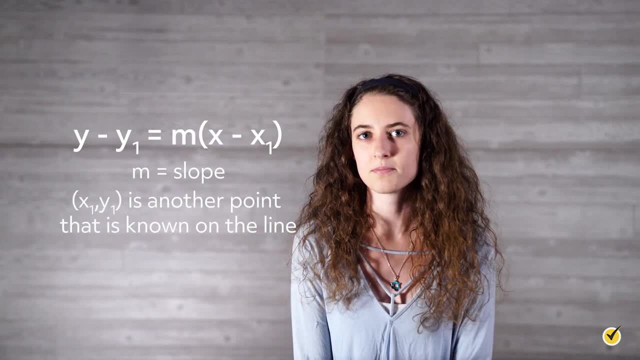 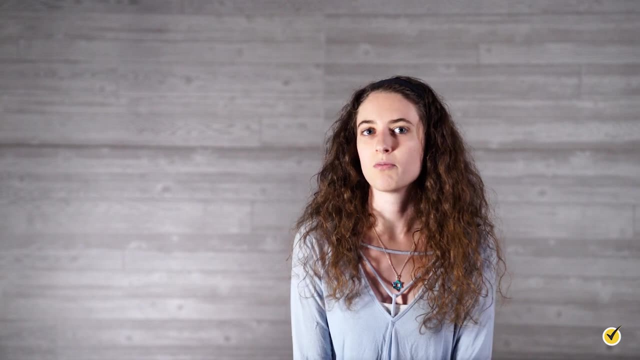 and x1y1 is another point that is known on the line. Using this template, let's practice identifying the slope and the point from the following examples of point-slope form: y minus 5 equals 3 times x minus 2.. 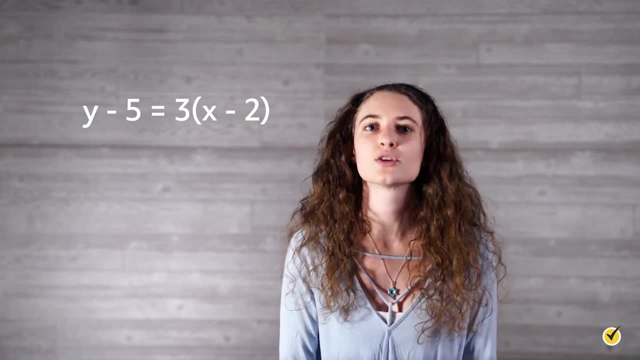 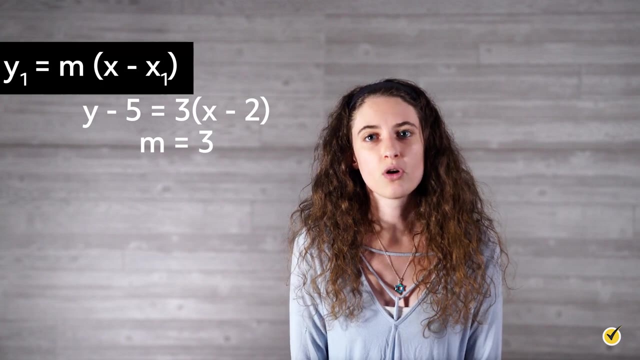 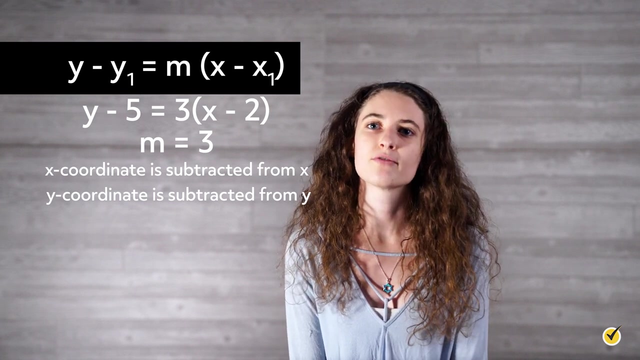 This is a straightforward example. First, identify the slope as the coefficient outside the parentheses, m equals 3.. When naming the point on the line, note that in the general form the x-coordinate is being subtracted from x and the y-coordinate is being subtracted from y. so the ordered pair. 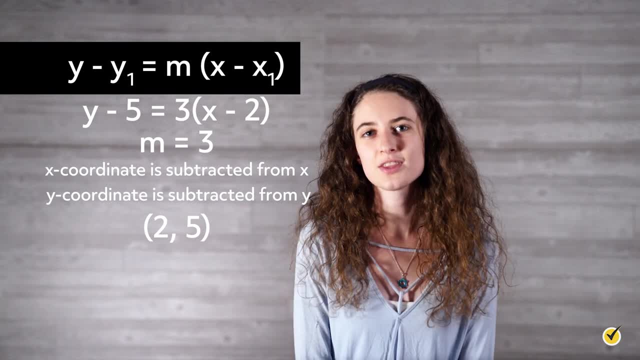 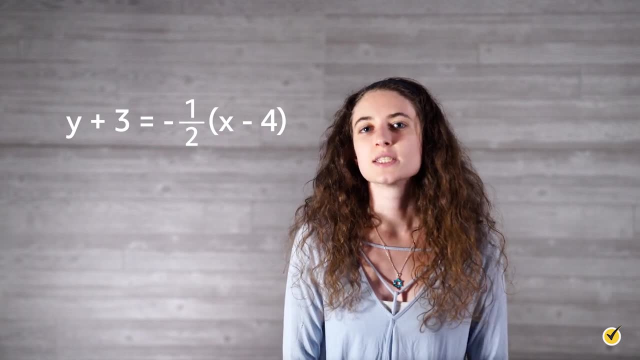 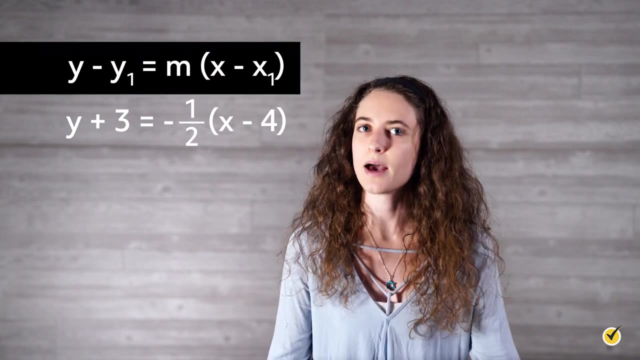 of the point will be 2, 5.. Here's another one: y plus 3 equals negative one half times x minus 4.. The slope in this equation is: m equals negative one half. How is this equation different from that general form? y-y1 equals m times x-x1?. 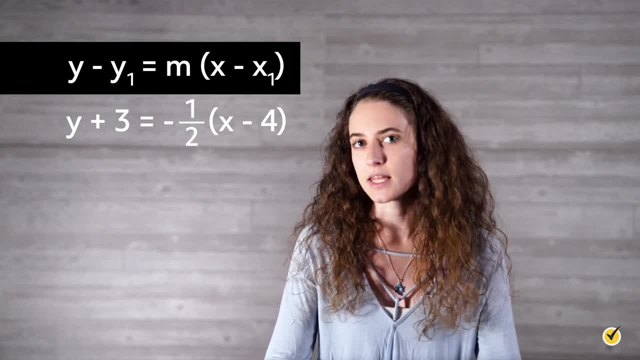 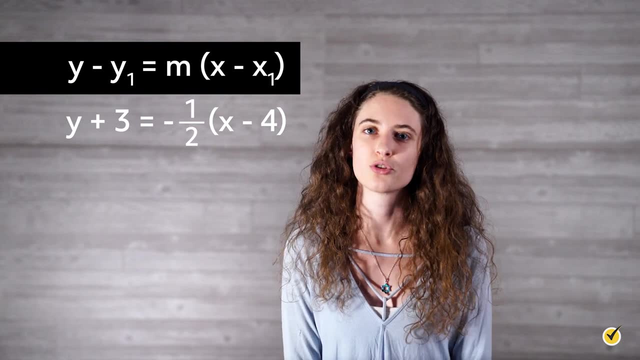 You may have noticed that the y value of point-3 is being added To identify the point, that is on this line, the equation must look like the general form which subtracts the coordinates of the point. Therefore, the point can be seen more clearly if the equation is written as y minus negative. 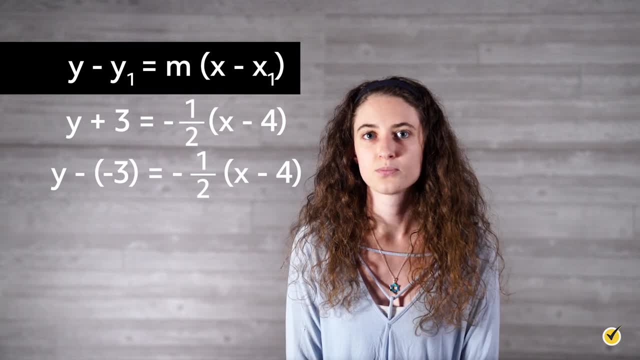 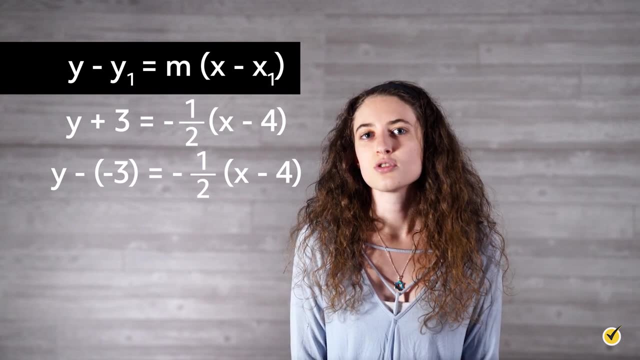 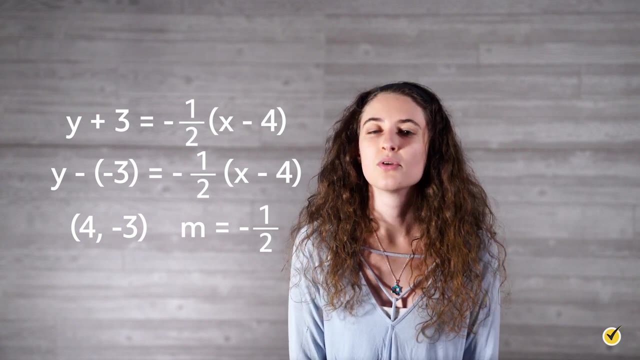 3 equals negative one-half times x minus 4.. Subtracting a negative value is the same as addition. Now we can see that this line travels through the point and has a slope. of m equals negative one-half. Let's look at one more example. 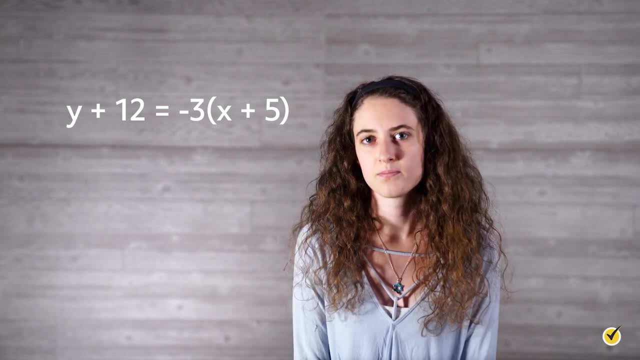 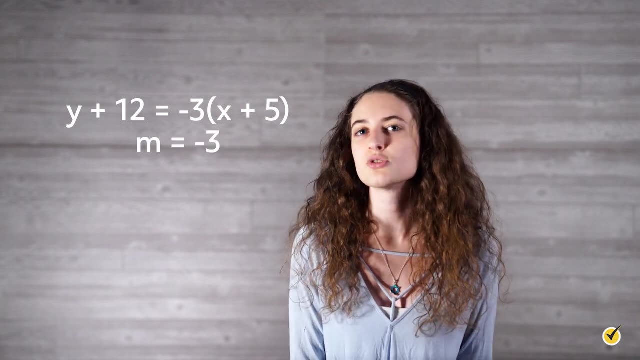 y plus 12 equals negative 3 times x plus 5.. By now you can quickly see that the slope of this equation is: m equals negative 3.. This equation also does not match the general form, but it can be rewritten as follows: 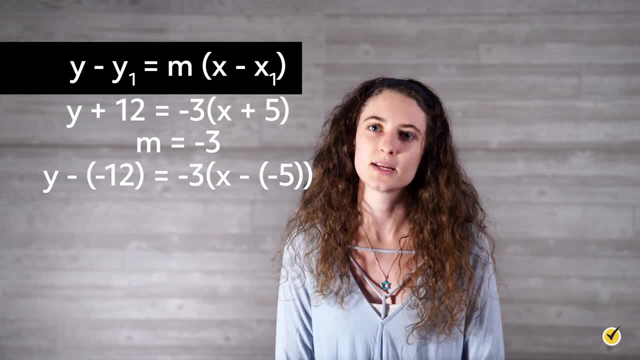 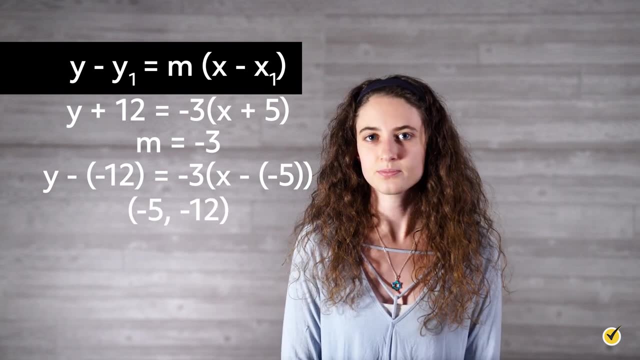 y minus negative 12 equals negative 3 times x minus negative 5.. This adjustment reveals that the point that is on the line is negative 5, negative 12.. Once you feel comfortable with identifying the slope and the point from this form, you: 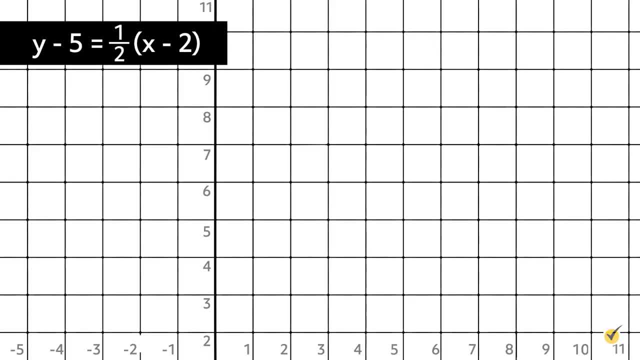 can graph the line as we did before: y minus 12 equals negative 3 times x minus 5.. y minus 12 equals negative 3 times x minus 5.. y minus 12 equals negative 3 times x minus 5. equals one-half times x minus 2.. 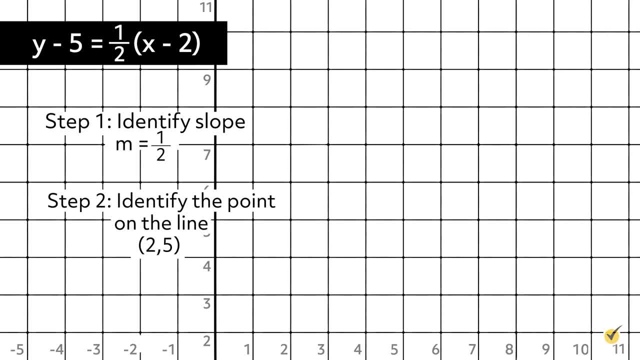 Step 1. Identify the slope. m equals one-half Step 2. Identify the point on the line. Some students find it helpful to switch the sign of the given formula to determine the coordinates of the point. Step 3. Plot the point as the first point. 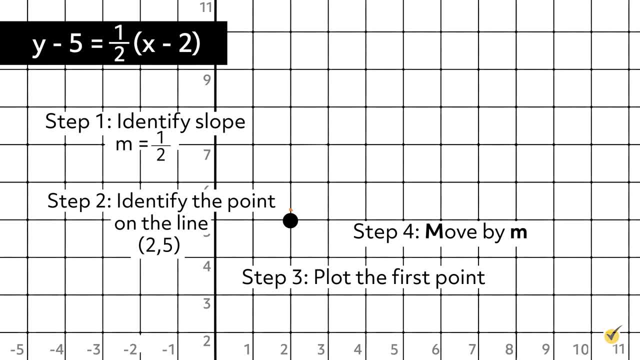 Step 4.. Move by m equals one-half. Rise equals up 1.. Run equals right. 2.. Plot the second point at 4, 6. Step 5.. Repeat the rise equals up 1 and run equals right 2.. 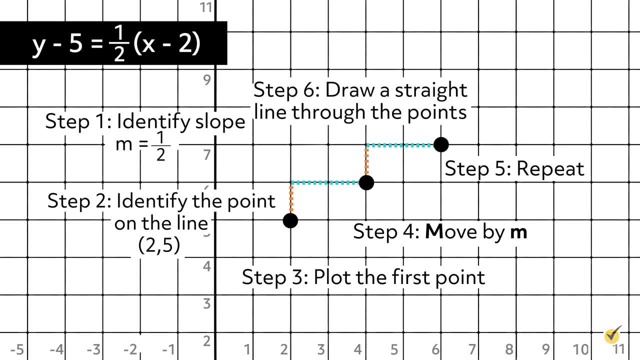 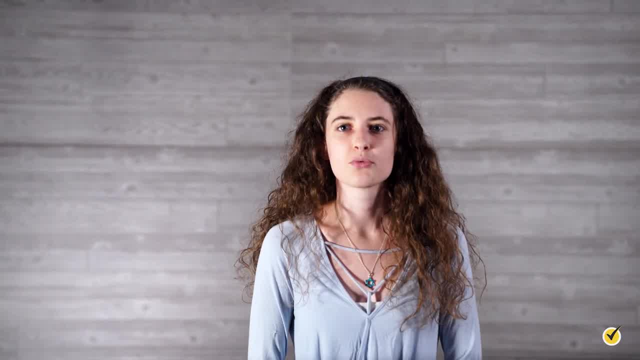 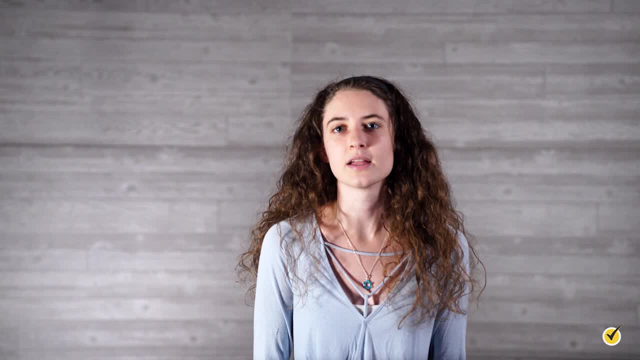 Plot the third point at 6, 7.. Step 6. Draw a straight line through the three points. Alright, we've covered a lot of ground in this video regarding the different ways linear equations can be written. While the structure of the equations looks different, they all represent a line. 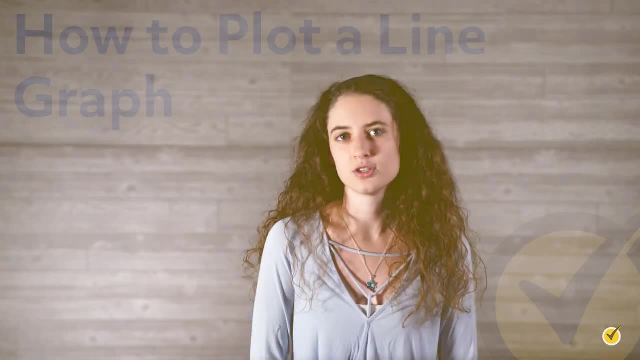 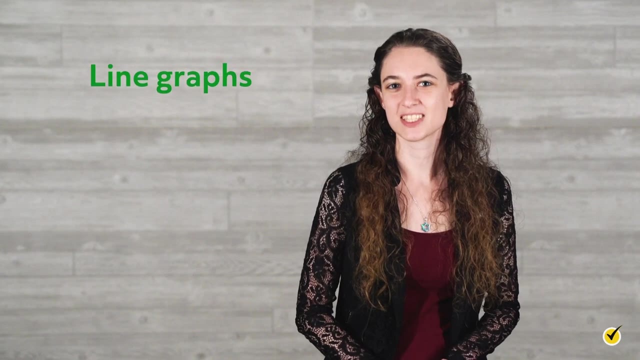 The use of each depends on what you are given or what you are given. The use of each depends on your own interpretation of the equation or what you are asked to do. Hello and welcome to this video about line graphs. Today, we'll explore what a line graph is and what type of data it's used to represent. 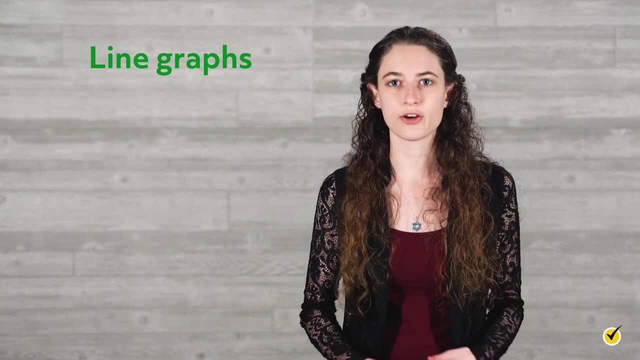 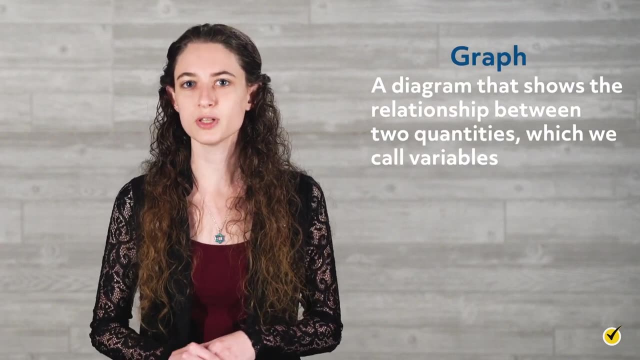 We'll also learn how to use line graphs to interpret situations in the real world. Before we get started, let's review a few things First. a graph is a diagram that shows the relationship between two quantities, which we call variables. These variables are measured along the x-axis and y-axis on a coordinate plane. 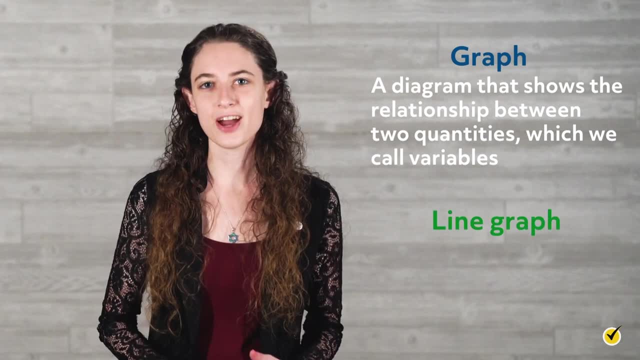 The line graph is a diagram that shows the relationship between two quantities. The line graph is a diagram that shows the relationship between two quantities, which we call variables. A line graph is a type of graph that displays quantitative data as a series of points called. 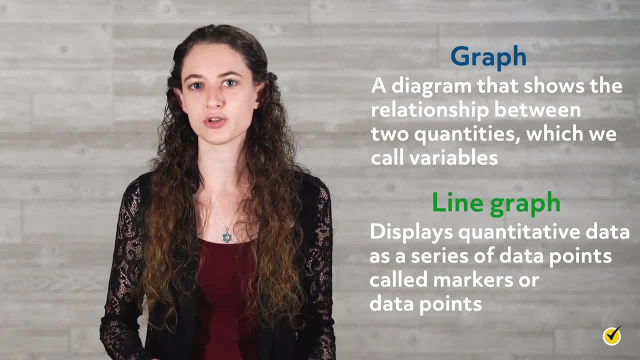 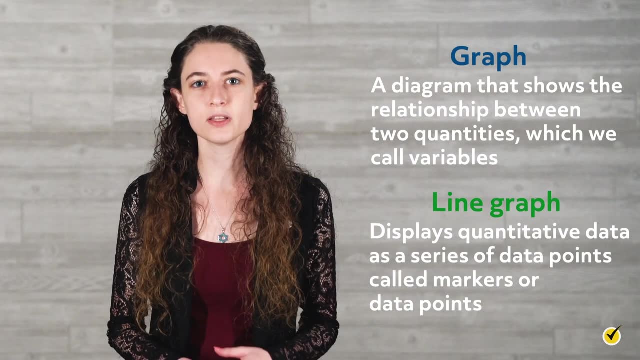 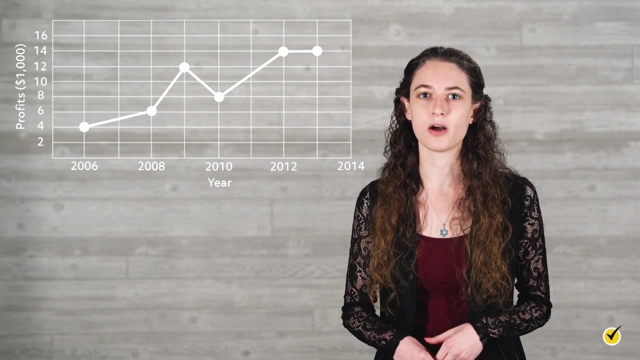 markers or data points. These data points are connected by straight line segments. The connected data points show the relationship between two variables. A line graph is typically used to show information that changes over time. Let's take a look at an example. This line graph shows the change in a company's profits over 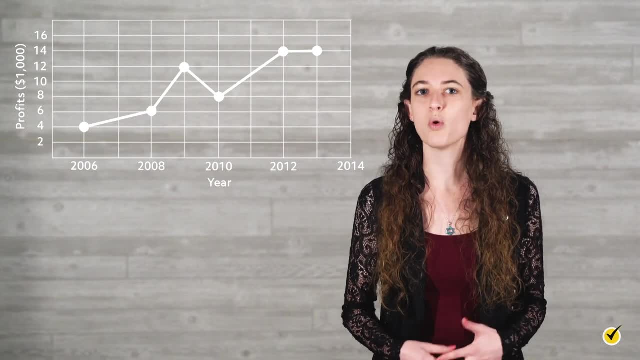 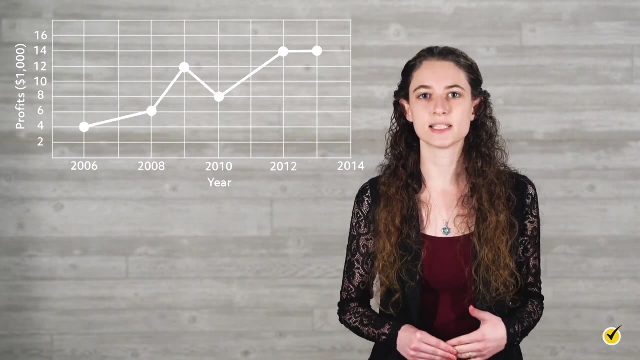 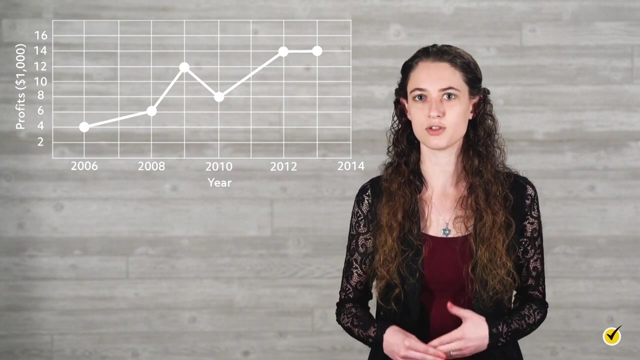 several years. The x-axis is labeled year and the y-axis is labeled profits. We see that line segments connect the data points plotted on the graph. Since the line segments are generally moving in a positive direction, we can say that the company's profits tended to increase from 2006 to 2013.. 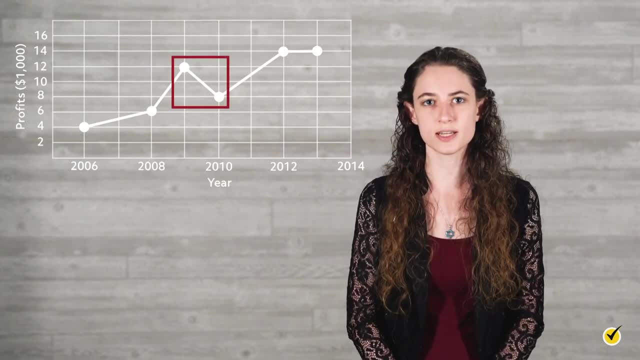 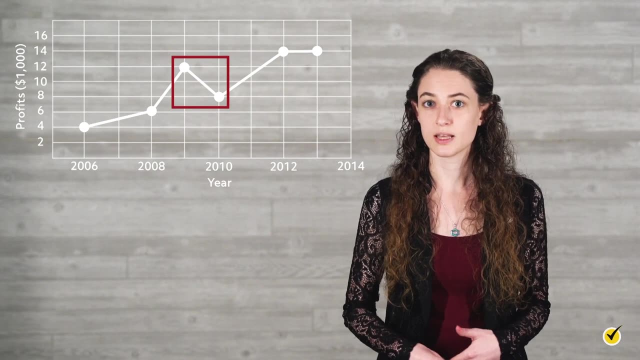 Let's take a look at the line segment connecting the data points for the years 2009 and 2010.. We can see that this particular line segment is positioned in a downward or negative direction. This tells us that the company's profits decreased from 2009 to 2010.. 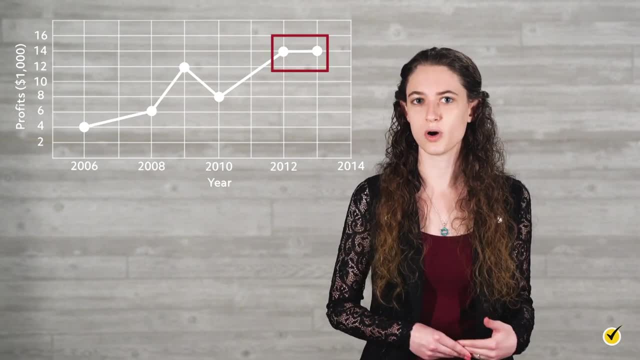 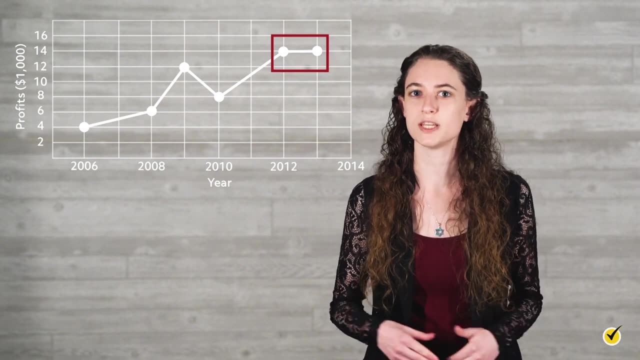 What do you notice about the line segment connecting the data points for 2012 and 2013?? They form a straight horizontal line. This shows that the company's profits neither increased nor decreased during this time frame. Instead, they stayed the same. 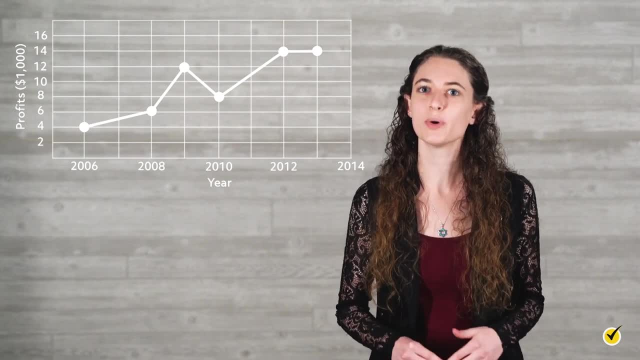 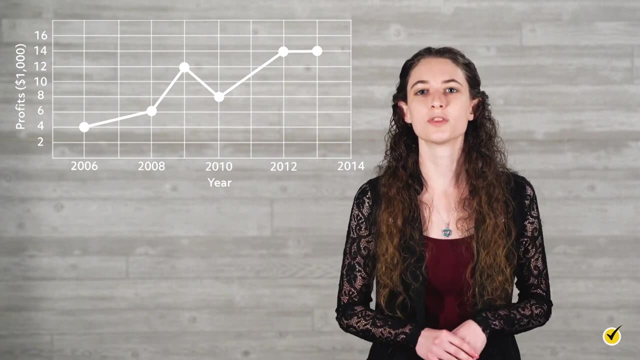 When constructing a line graph on a coordinate plane, the x-axis is always used to plot the independent variable and the y-axis is always used to plot the dependent variable. With line graphs, the independent variable is usually time In the graph we just looked at. 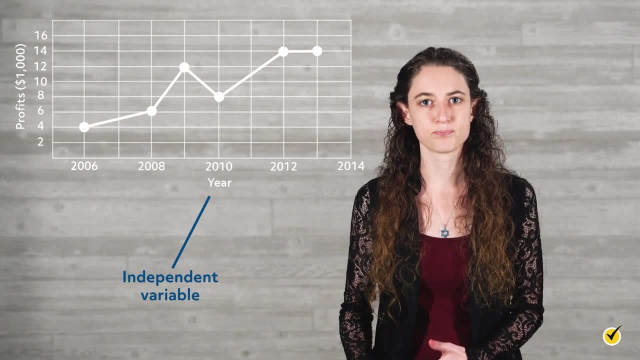 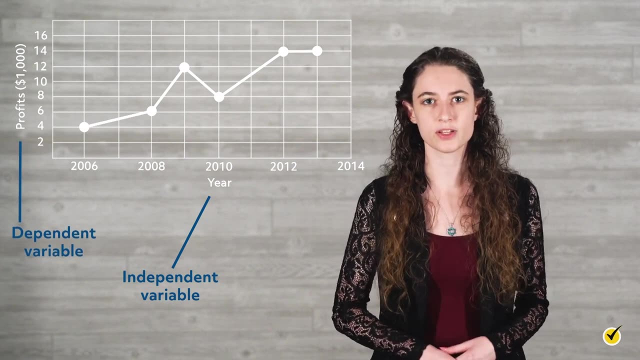 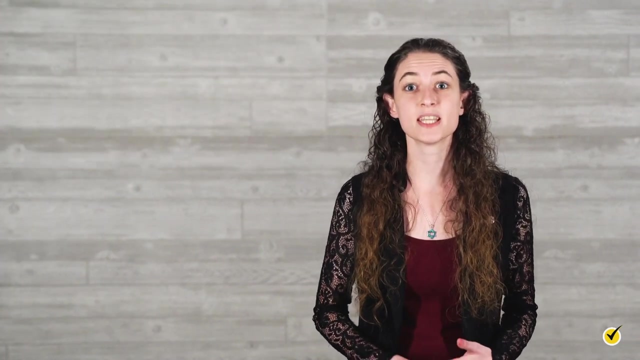 the independent variable is years, which is a measurement of time. The dependent variable is the factor that changes over time. In our example, the dependent variable is the company's profits, which increased and decreased from 2006 to 2013.. Line graphs are an important part of our everyday lives because they can swiftly 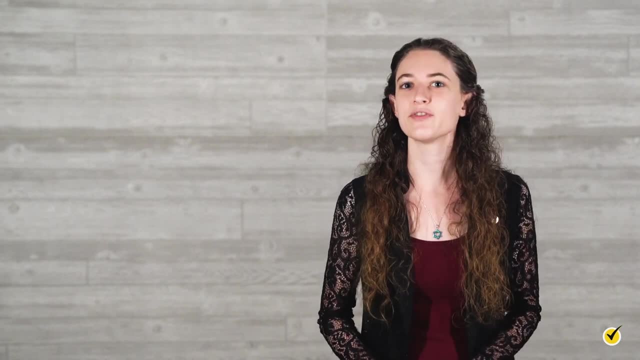 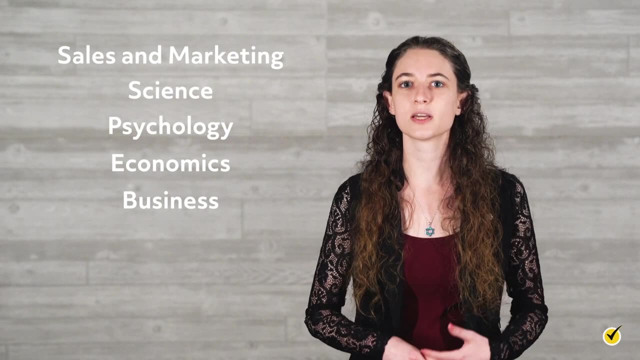 communicate data and trends. They're used in a wide variety of fields, including sales and marketing, science, psychology, economics and business. Additionally, line graphs can be used to make predictions. Let's look once more at our line graph showing the company's change in profits. 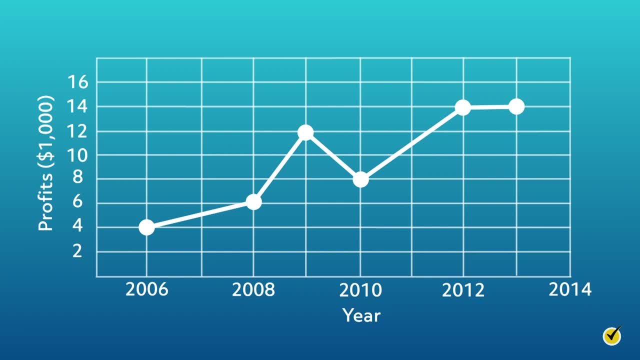 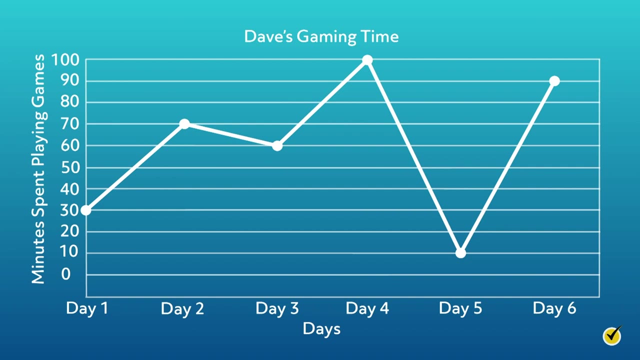 Based on the general trend shown, do you think the profits will increase or decrease in the future? We can infer that the profits may continue to increase based on the positive trend shown in previous years. Let's look at another line graph together. This graph shows how much time Dave spent playing video games each day. 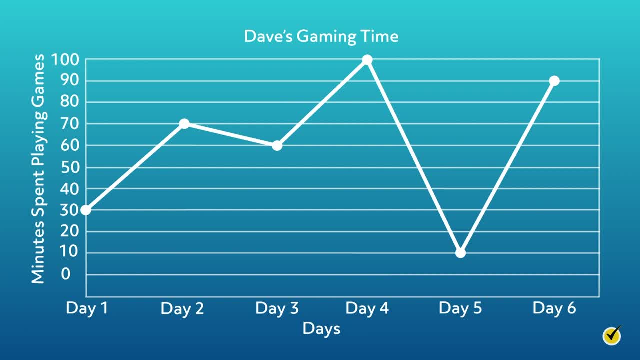 The horizontal x-axis shows the independent variable, which is days, and the vertical y-axis shows the dependent variable, which is days. The horizontal x-axis shows the independent variable, which is minutes spent playing games. Each marker shows the data point for how many minutes of. 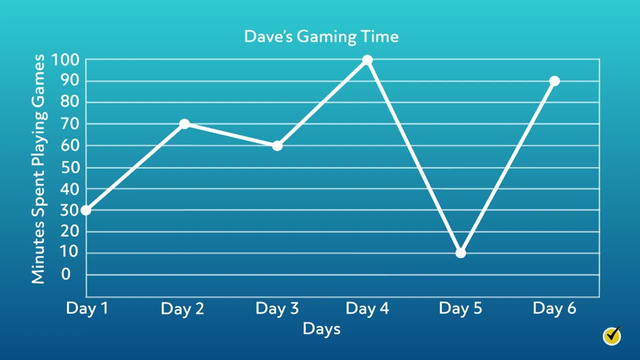 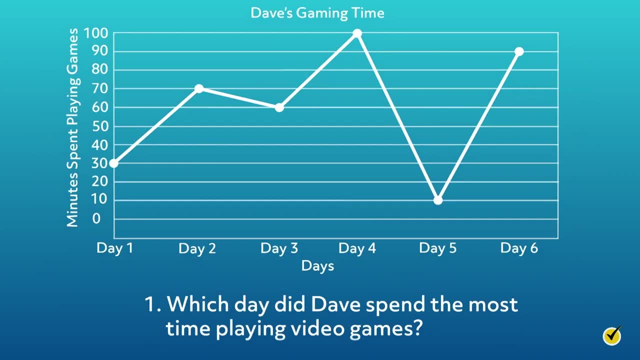 video games Dave plays each day. Let's use this information to answer some questions. Which day did Dave spend the most time playing video games? Dave spent the most time playing video games on day four. We know this because the marker for day four is higher than the markers for the rest of the days shown. On day four, Dave played games. 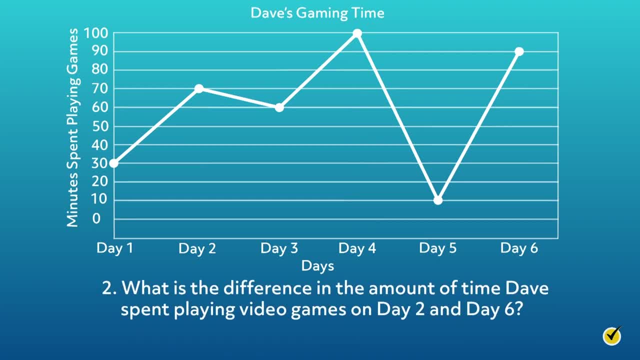 for a hundred minutes. That's a lot of gaming. What is the difference in the amount of time Dave spent playing video games on day two and day six? Looking at the markers, the graph shows that Dave played games for 70 minutes on day two. 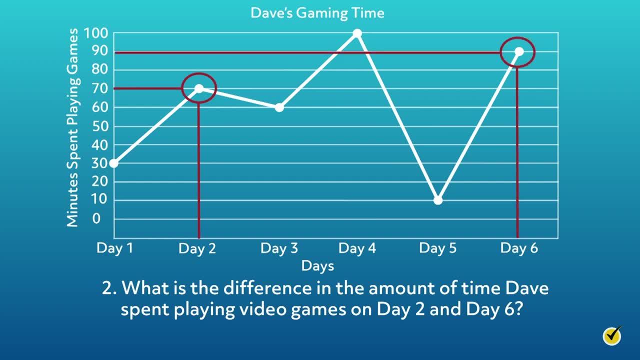 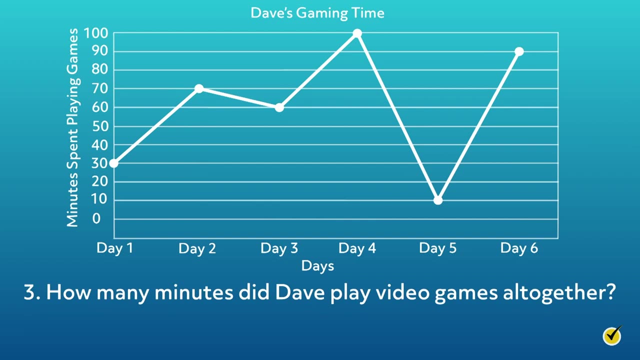 and 90 minutes on day six. The difference is calculated by subtracting, Since 90 minus 70 equals 20, the difference is 20 minutes. Dave spent 20 more minutes playing video games on day six. How many minutes did Dave play video games altogether To find the total amount of time? 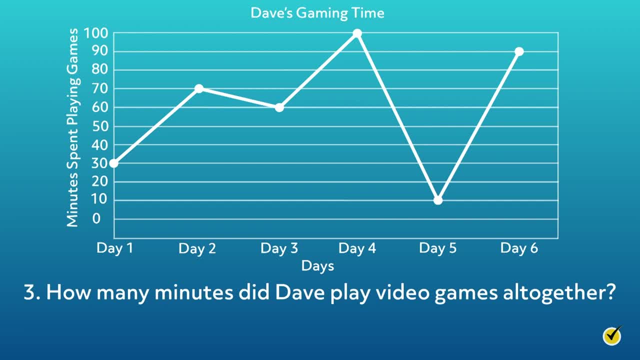 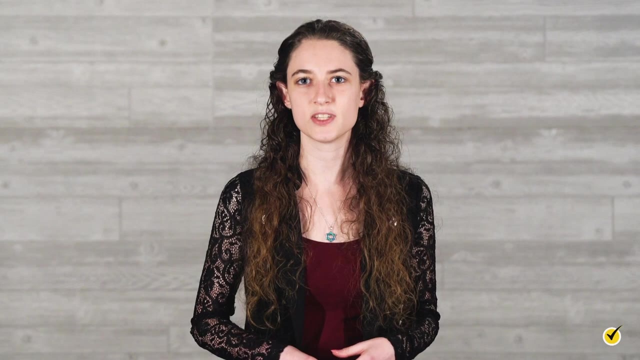 Dave played video games. add the amount of time Dave spent playing video games on day six: Dave spent 30 plus 70 plus 60 plus 100 plus 10 plus 90 equals 360.. Therefore, Dave spent 360 minutes playing video games from day one through day six. A line graph can show multiple sets of. 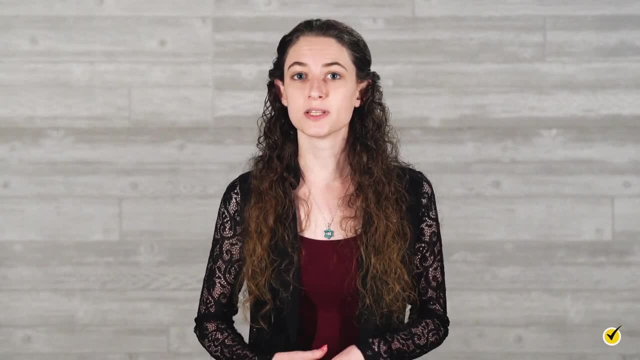 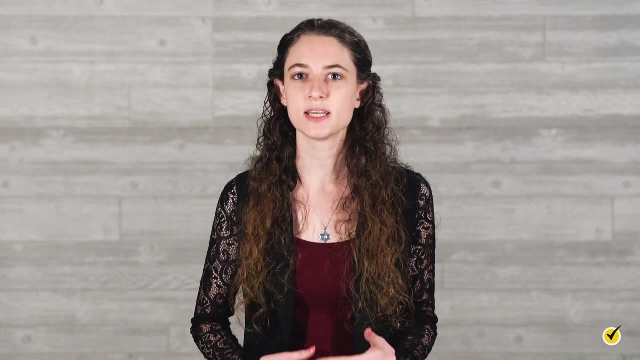 data if the same two variables are related. Graphing multiple data sets on a line graph can be very informative because they can be compared and contrasted. When this happens, each data set is typically represented by a distinct color. The line graph contains the: 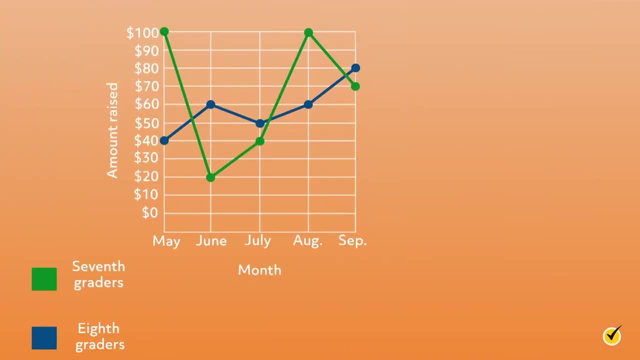 key that explains what data set each color stands for. Let's take a look at a line graph that shows two sets of data. This graph shows how much money was raised in a school fundraiser each month. The horizontal x-axis shows the independent variable, which is month, and the vertical y-axis shows the. 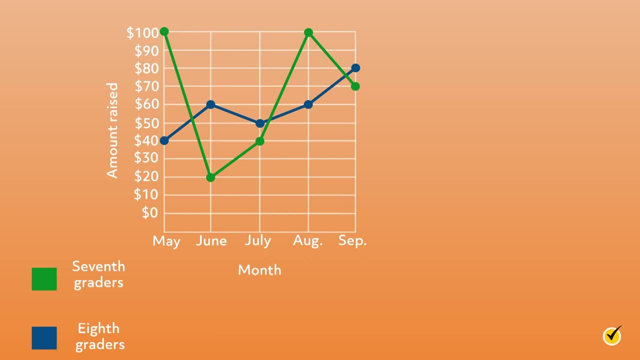 dependent variable, which is amount raised. Each marker shows the data point for how much money was raised in each month shown. The two data sets are graphed in two different colors: blue and green. By reading the key beneath the graph, we see that green represents money raised by 7th grade students. 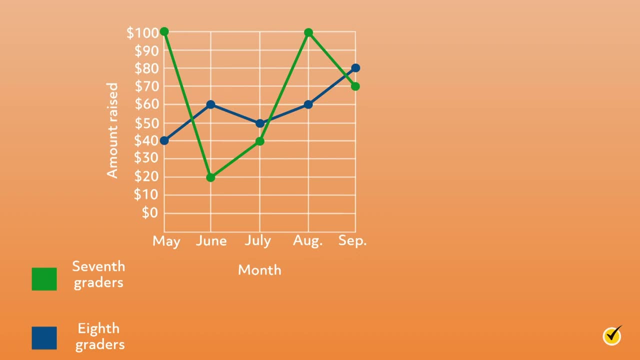 and blue represents money raised by 8th grade students. Let's use this information to answer some questions. Pause the video after each question is asked. Then look at the graph and see if you can answer it yourself. When you're ready, resume and check your work. 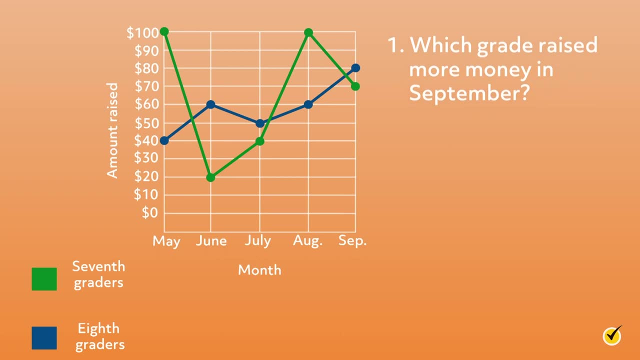 Which grade raised more money in September? 8th grade students raised more money than 7th grade students in September. Remember that blue. blue data points represent 8th grade students and green data points represent 7th grade students. Looking at the markers for September, we see that the blue marker is higher than the green marker. 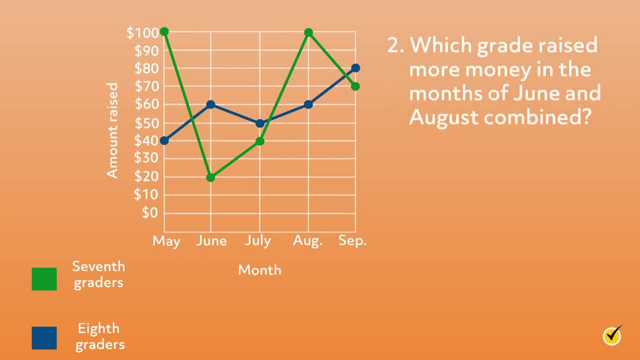 so 8th grade students raised more money in September. Which grade raised more money in the months of June and August combined? The 8th grade students shown in blue raised $60 in June and $60 in August. 60 plus 60 equals 120,. 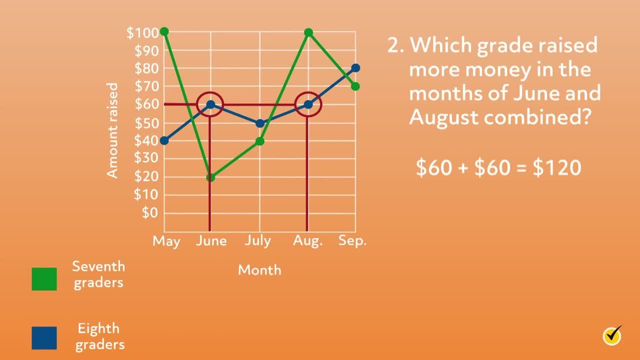 so the 8th grade students raised $120.. The 7th grade students shown in green raised $20 in June and $100 in August. 20 plus 100 equals 120, so the 7th grade students raised $120 in June and August. As you can see, both grades raised the. 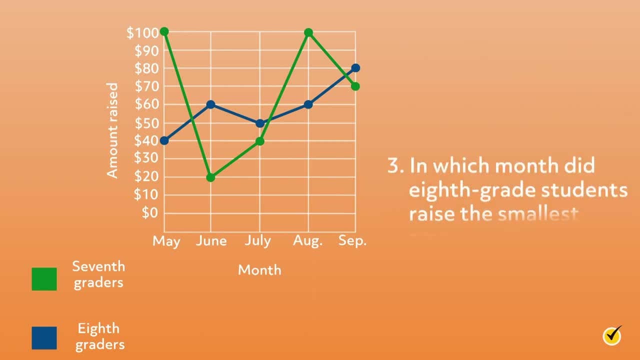 same amount of money in the months of June and August combined. In which month did 8th grade students raise the smallest amount of money? How much money was raised? We can find the answer by examining the blue markers representing the 8th grade data points in each month: The month that. 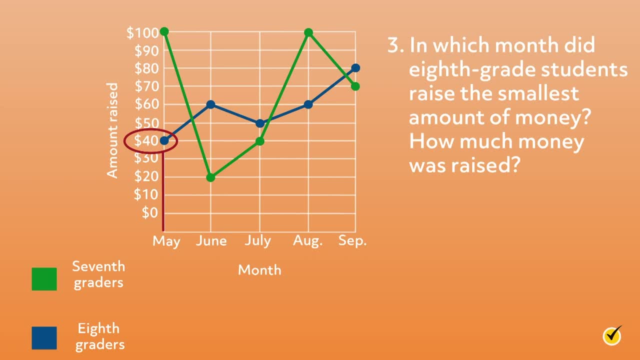 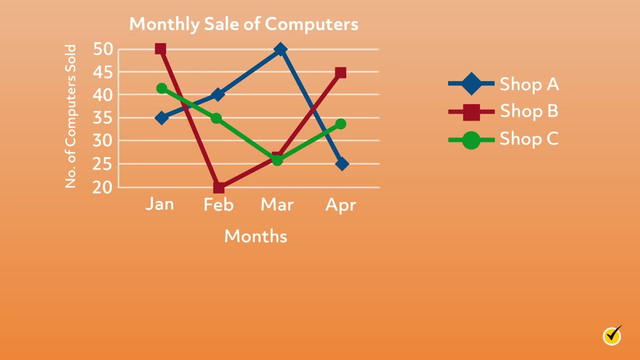 the marker is placed. the lowest is in May, when they raised $40.. I have one last graph for you to analyze. This one is a little more challenging, but I know you can handle it. As you can see, this line graph displays three sets of data. Consider the following questions. 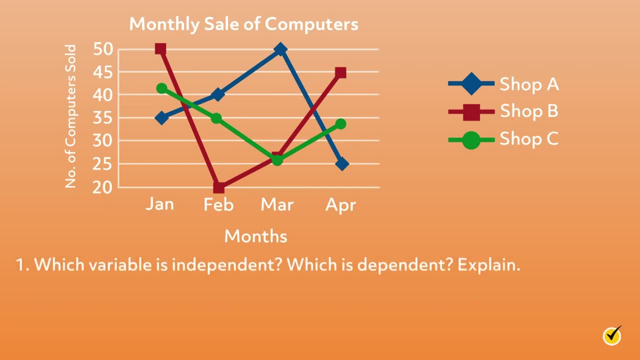 Which variable is independent? Which is dependent? Explain In which month was the number of computers sold in shop C almost identical to the number sold in shop B. In which months did shop A sell more computers than shops B or C? Pause this video and analyze the line graph and see if you can answer these questions yourself. 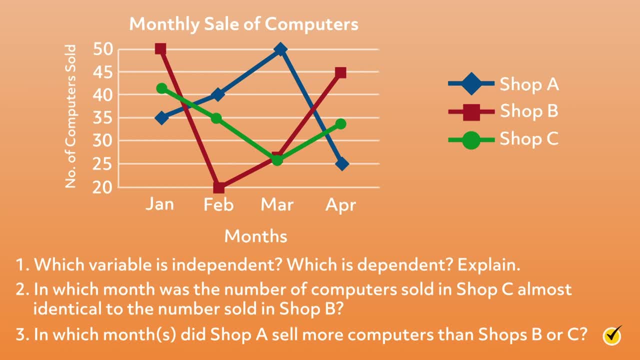 When you're ready, resume the video and we'll go over the answers together. Now that you've tried these problems yourself, let's go over them together. Which variable is independent? Which is dependent? Explain: The variable is months. which is on the x-axis? The independent variable is always measured along the 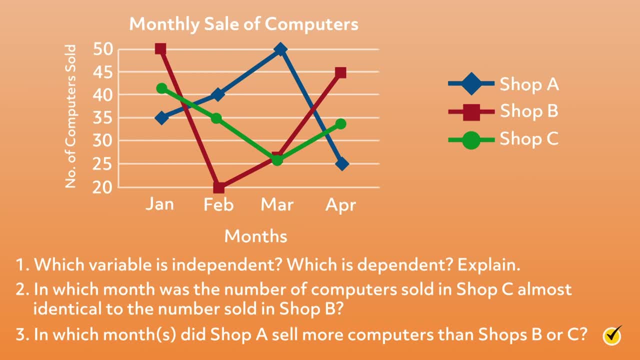 x-axis and it usually pertains to time. In this case, time is measured in months. The dependent variable is number of computers sold, which is on the y-axis. The value of the dependent variable relies on the independent variable. In this case the number of computers each store sold depends. 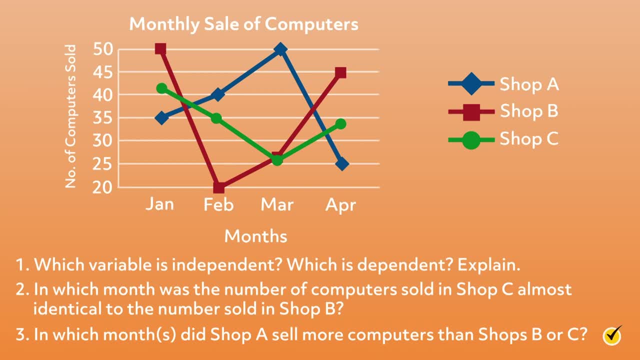 on the month. In which month was the number of computers sold in shop C almost identical to the number sold in shop B, March? When we look at the markers for that month, we see that the red marker for shop B and the green marker for shop C almost overlap entirely. This indicates that the number 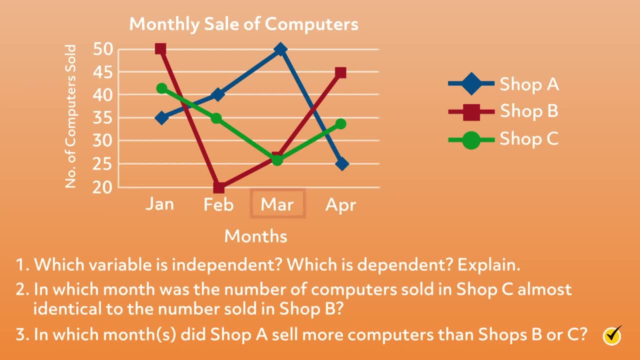 of computers sold by each shop was about the same. In which months did shop A sell more computers than shops B or C? February and March. To find out when shop A sold the most, look for when the blue markers are higher than the green or red markers. 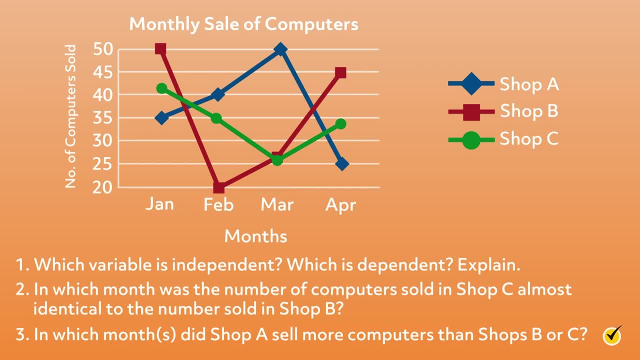 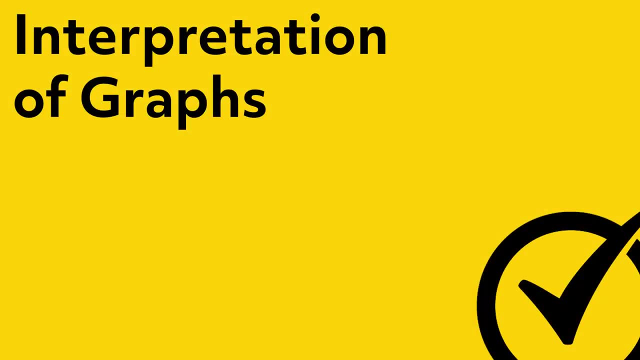 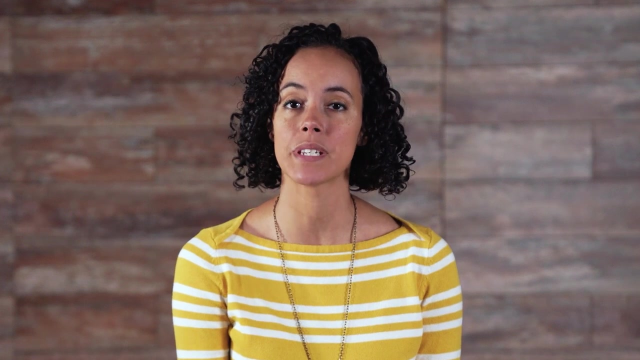 Shop A sold four: 40 computers in February and 50 computers in March. Line graphs are useful tools for showing how factors change over time. It's been said that a picture is worth a thousand words. This is true of the many different ways that data can be transformed into visual representations for easier interpretation. 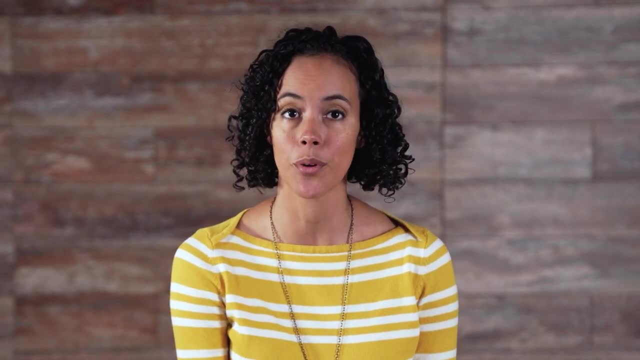 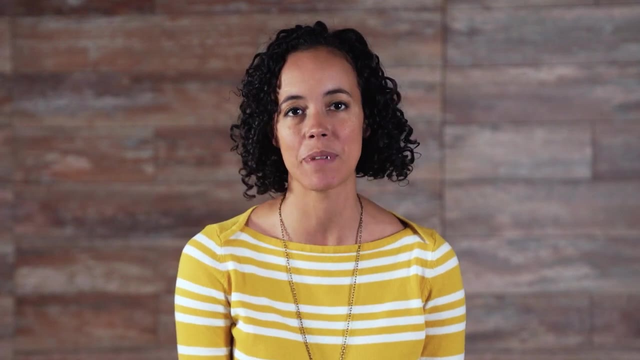 Data in and of itself can be difficult to explain, but when it is carefully organized, patterns can be revealed, or it may become apparent that no patterns exist. Either way, both results are meaningful. Advances in technology enable us to collect and track data like never before. An interpretation of 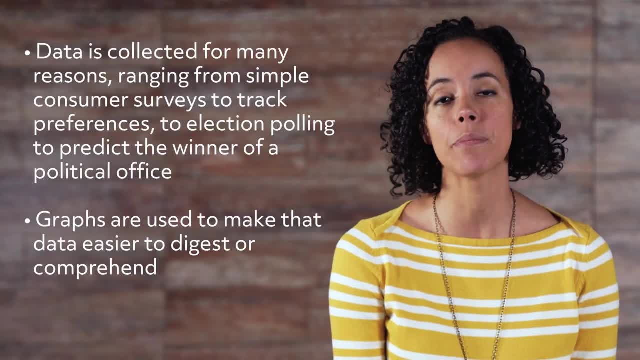 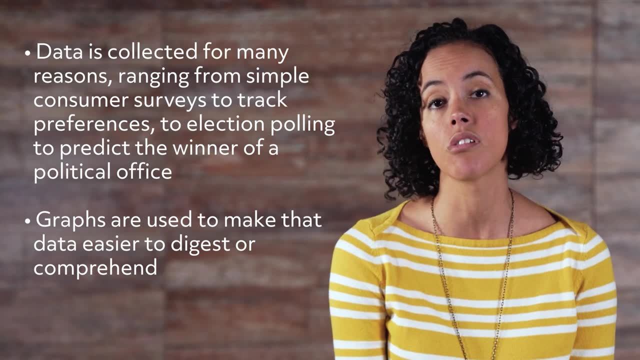 data is simplified with the use of graphs. Data is collected for many reasons, ranging from simple consumer surveys to track preferences, to election polling to predict the winner of a political office. Graphs are used to make that data easier to digest or comprehend Before we get to the 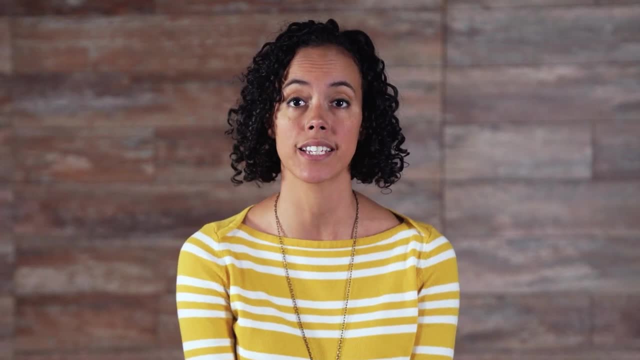 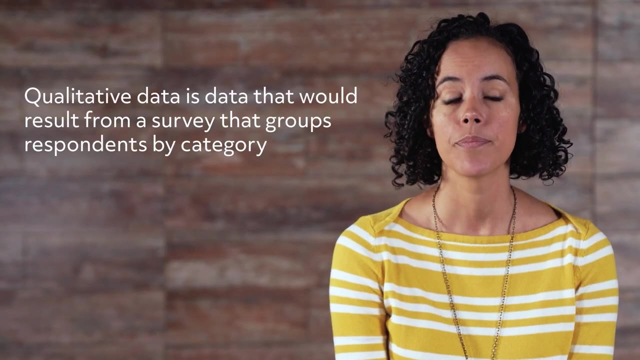 graphs. you should know that there are different types of data that can be collected. The first one we'll talk about is qualitative data. The first one we'll talk about is qualitative data. This data is from a survey that groups respondents by category. For example, you can survey students in your 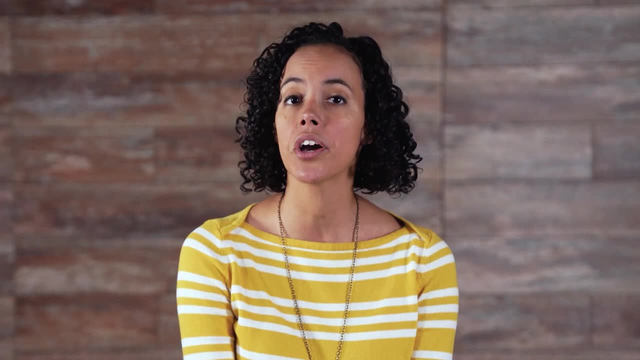 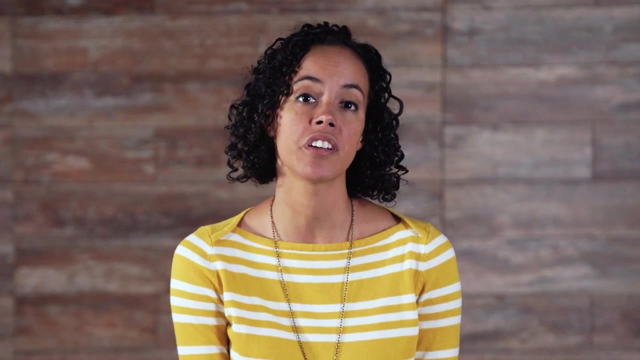 school and ask them to report their eye color, gender, area code and favorite movie type. These categories provide information for your study. In this case, maybe you're wondering whether there is a relationship between the number of blue-eyed sci-fi fans living in a particular area code. Well, 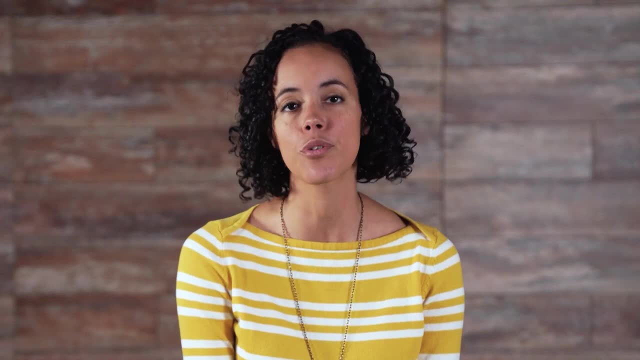 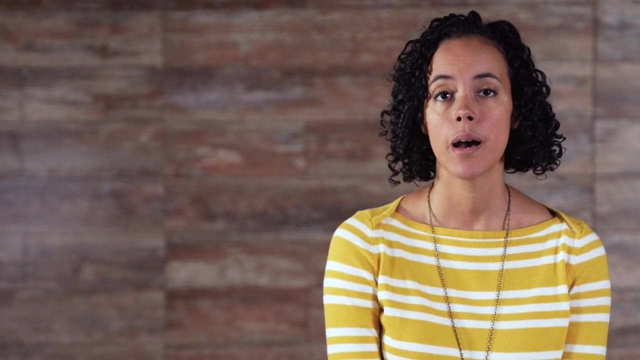 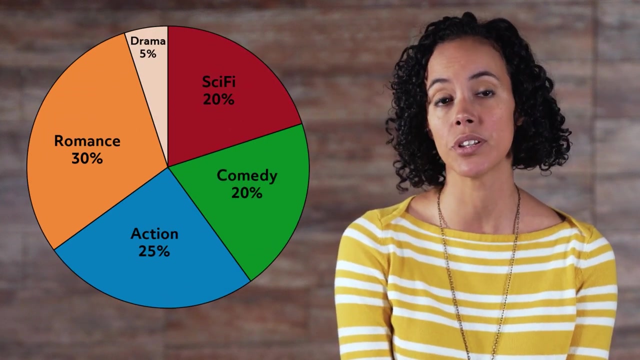 you may be able to detect a pattern in the counts of qualitative data by category. Graphs that are used to depict qualitative data are pie charts and bar graphs. A pie chart looks exactly like what you might expect: A pie: A circle representing 100% of a particular variable of. 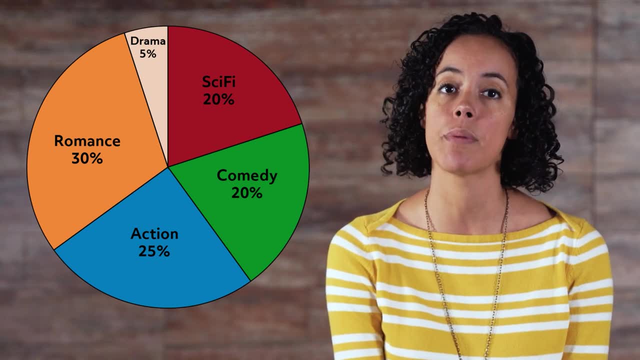 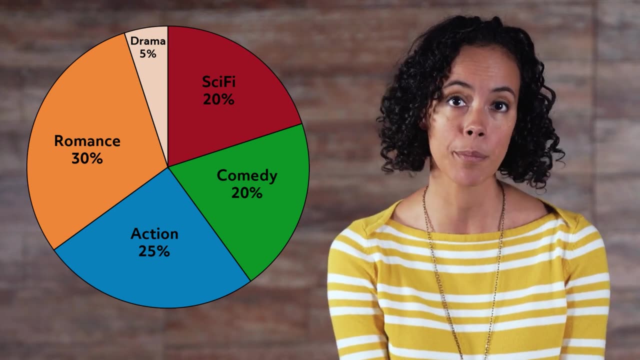 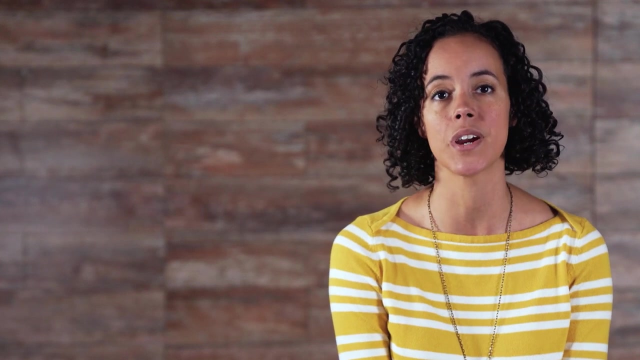 interest is divided into categories. Segments of the pie represent a percentage of the whole Pie. charts can also show counts. In this example, six people, or 30% of the respondents, favored romantic movies. Bar charts also show counts or percentages by category, but in a different way. 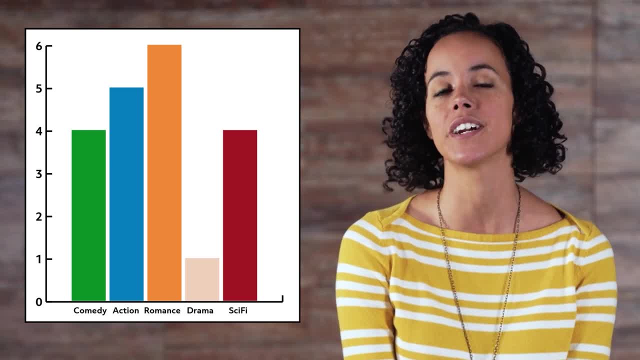 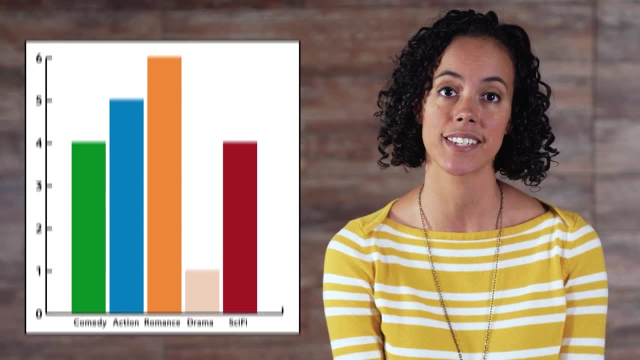 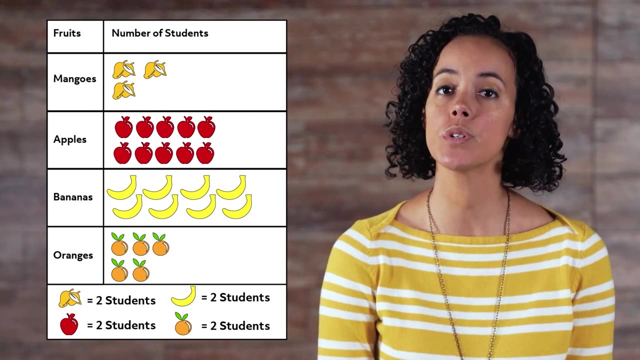 It looks like a city in the distance, with skyscrapers at varying heights. This bar chart shows categories on the horizontal axis with associated counts on the vertical axis. Next we have pictographs. As the name suggests, a pictograph provides visual context, Visual cues. 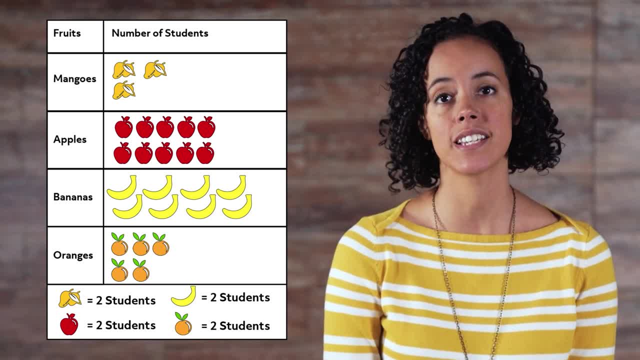 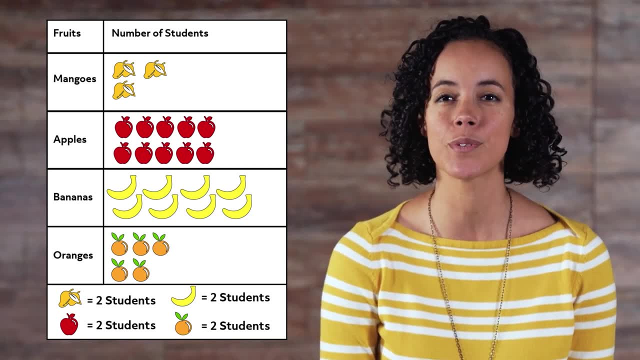 and images are used to represent the data, and keys are provided to tell you what each image or symbol represents. In this survey of student fruit preference, Apples took the lead, with 20 students reporting them as their favorite fruit. There are a total of 12 students and 12 students. 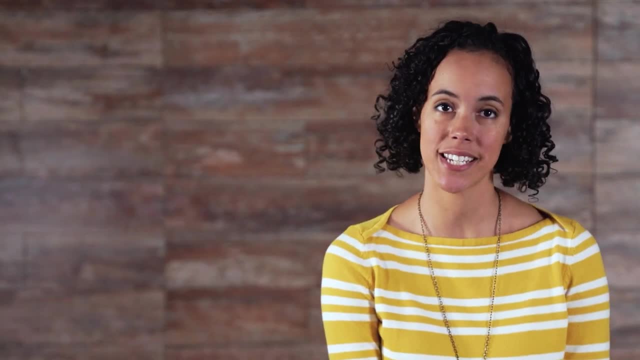 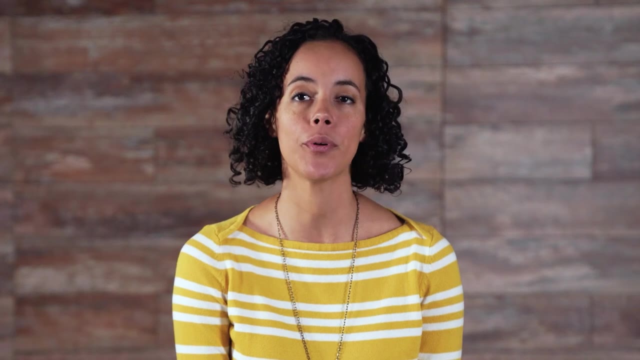 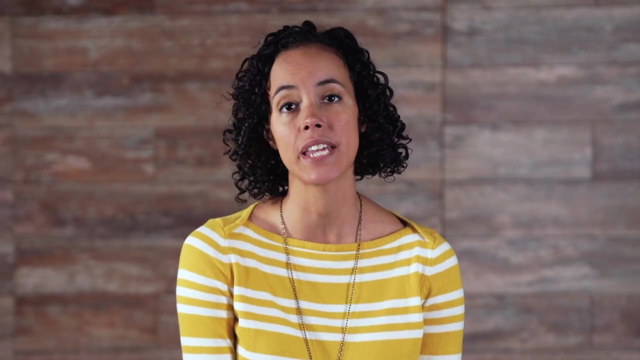 favorite. Another type of data that can be collected is known as quantitative. Unlike qualitative data, you can do math with quantitative data because it is numeric in nature. For example, what if you're interested in the average AP statistics score of the graduating class of your high school? Gathering reliable data may be the trickiest part of your study. 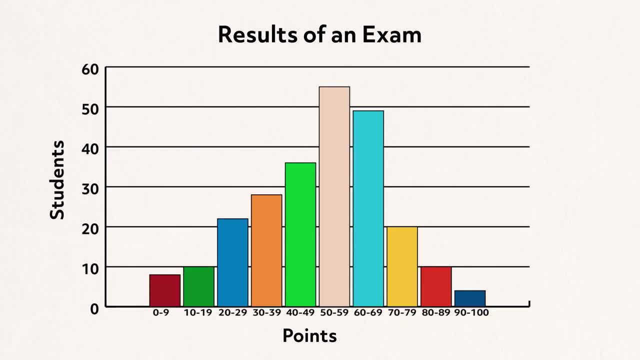 but a histogram can relay trends and the results with precision. A histogram resembles a bar graph, with the exception of spaces between the bars. There's a range of numeric values displayed on the horizontal axis and the counts of students are displayed on the vertical. 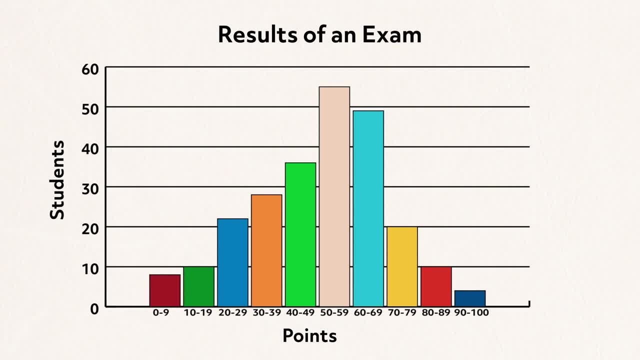 axis, The pattern of scores may appear somewhat symmetric, which is typically referred to as normally distributed. This would suggest that most students scored in the middle of the range and that there were some high achievers and others who were not so successful. A histogram. 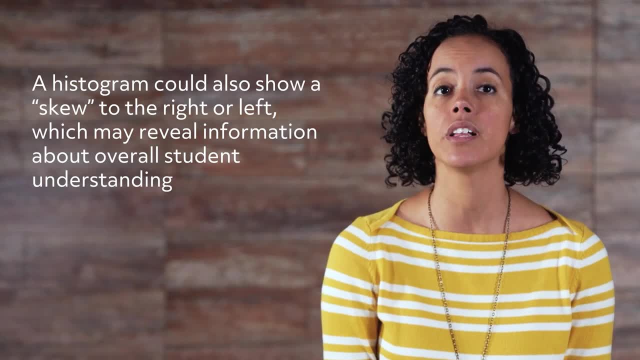 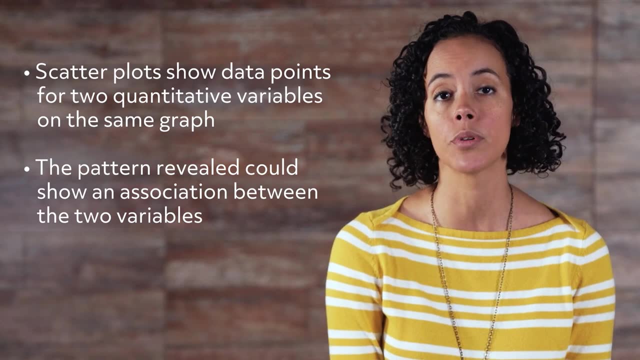 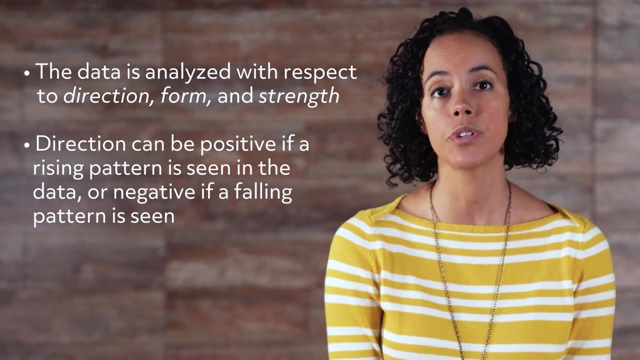 could also show a skew to the right or left, which may reveal information about overall student understanding. Scatter plots show data points for data points for two quantitative variables on the same graph. The pattern revealed could show an association between the two variables. The data is analyzed with respect to direction, form and strength. 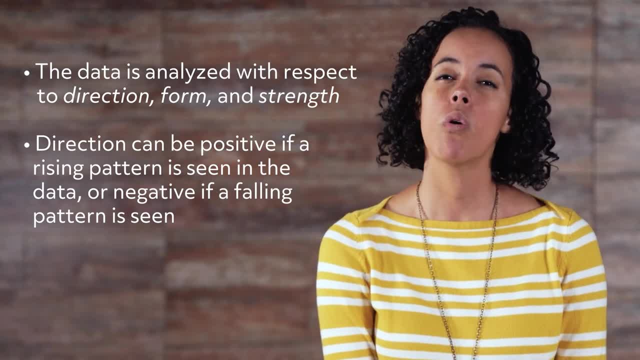 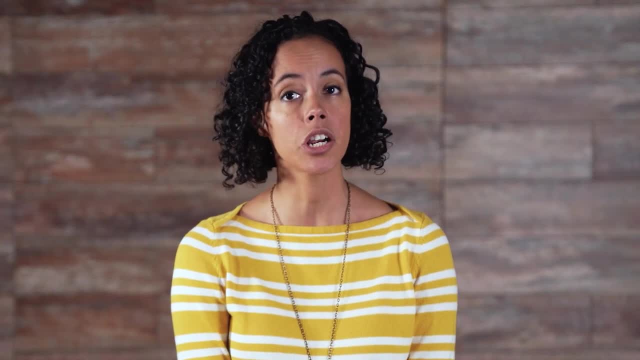 Direction can be positive if a rising pattern is seen in the data, or negative if a falling pattern is seen. The form of the scatter plot identifies whether the data appears somewhat linear, curved or cone-like in shape. Strength associates how tightly the points are gathered. 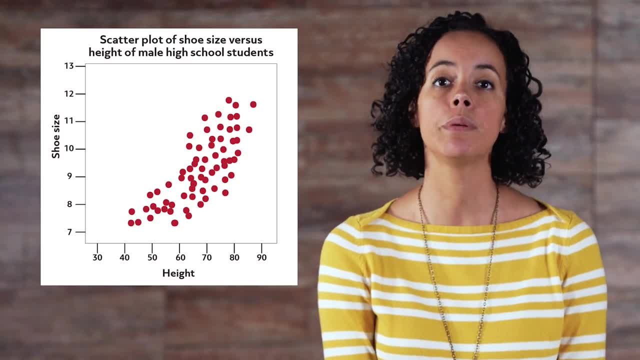 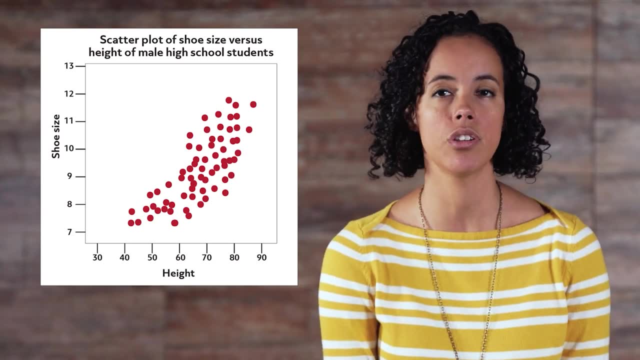 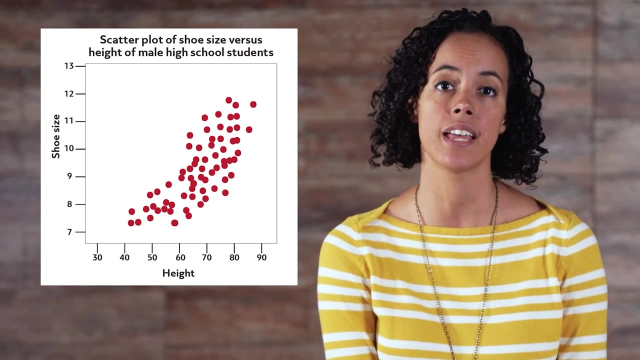 An example of a strong, positive, somewhat linear pattern could be revealed in a scatter plot of shoe size versus height of male high school students. Because typical male students continue to grow during the high school years, the data for all male students would likely show underclassmen data points at the lower end of the scatter. 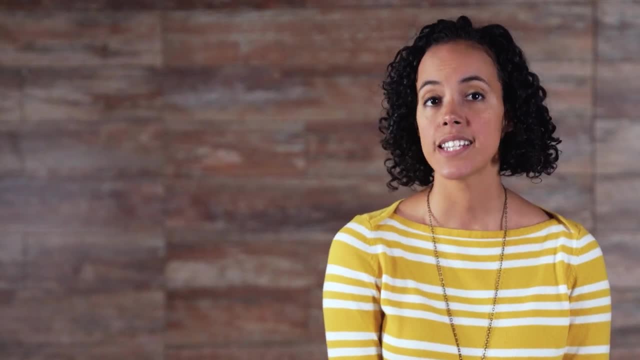 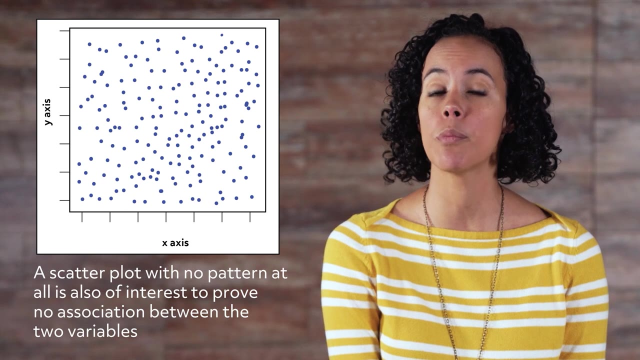 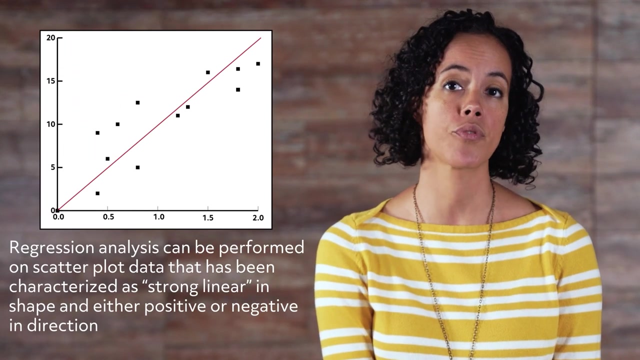 plot and upperclassmen represented at the higher end. Data points that do not fit a recognizable pattern are referred to as outliers. Finally, a scatter plot with no pattern at all is also of interest to prove no association between the two variables. Regression analysis can be performed on scatter plot data that has been characterized as strong.